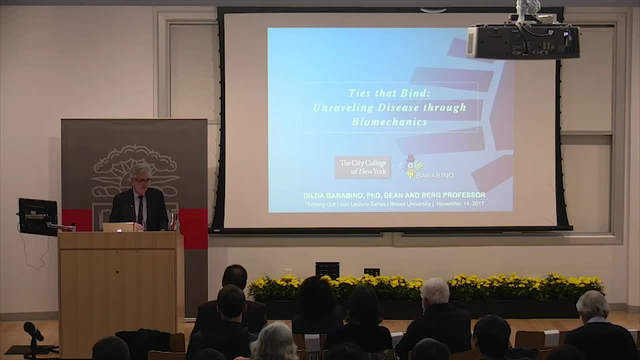 really a characteristic of the speakers that we've had come in the series that they are really amazing examples of people who are doing cutting edge scientific research, training graduate students, And I think it's a great example of that, And I would also say that she's very busy. 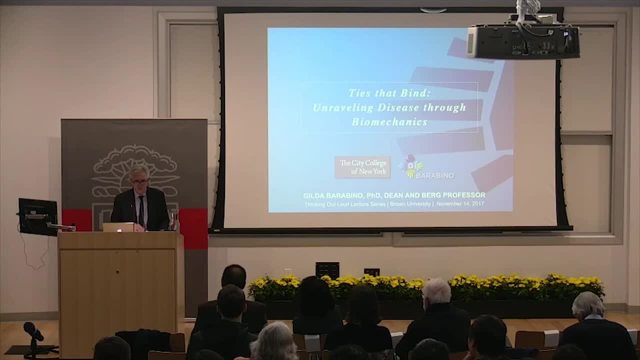 She's very, very active in the science field. She's working with undergraduates, giving lectures in high schools and elementary schools And, you know, at the same time remaining engaged at the level of the profession, which is so important, encouraging young scholars to take on those. the 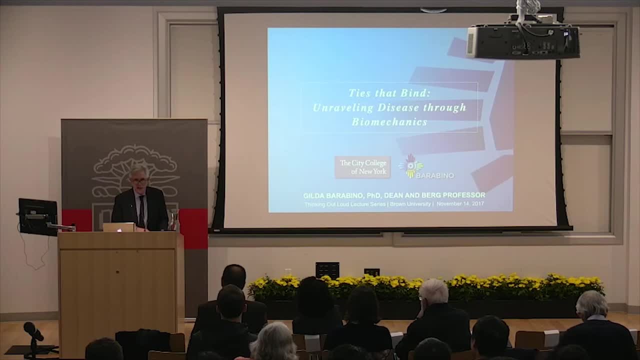 challenges of doing PhD work in the sciences, And especially from from for young scholars who may come from groups that have traditionally not participated in high levels in those endeavors. So it's a special pleasure to welcome Dr Gilda Barabino. 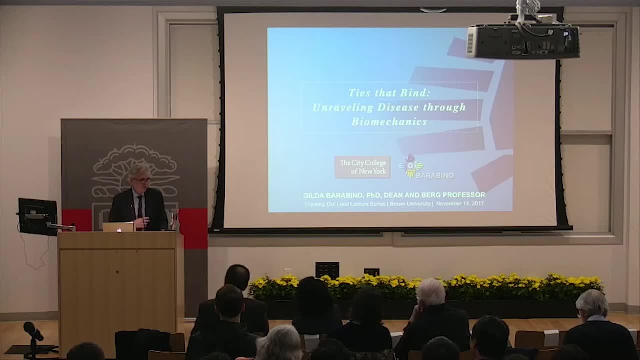 and I will just list a few of her positions and accomplishments before I turn it over to my colleague, Chris Rose. She is currently the Dean and the Berg Professor at the Grove School of Engineering at the City College of New York. She has faculty appointments in biomedical engineering, chemical engineering. 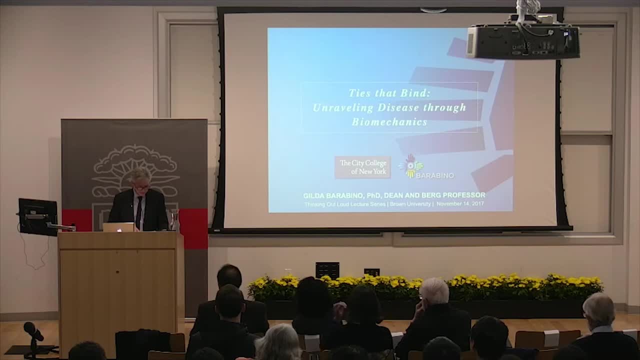 and also an appointment at the Sophie Davis School of Biomedical Education slash CUNY School of Medicine. Prior to CUNY, she was the Associate Chair of Graduate Studies and a professor in the Wallace. She also served at the H Coulter Department of Biomedical Engineering at Georgia Tech in Emory. 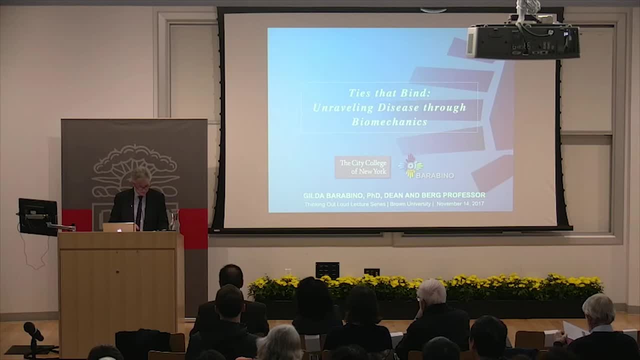 At Georgia Tech. she also served as the Vice Provost- the inaugural Vice Provost- for Academic Diversity. Prior to her appointments at Georgia Tech in Emory, she rose to the rank of full professor of chemical engineering and served as Vice Provost for Undergraduate Education at Northeastern University. 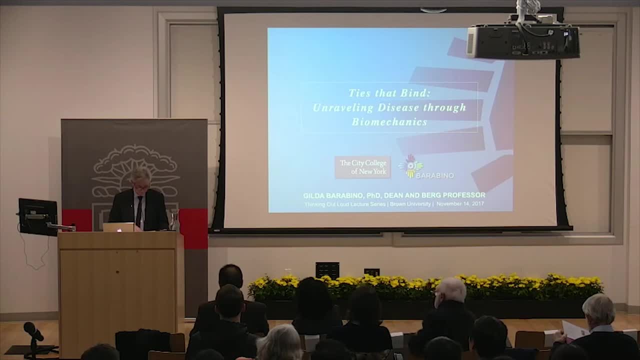 Her research is on sickle cell disease, as I'm sure most of you know, and on cellular and cellular disease. Her research is on sickle cell disease, as I'm sure most of you know, and on cellular and cellular disease, and on cellular and cellular disease. 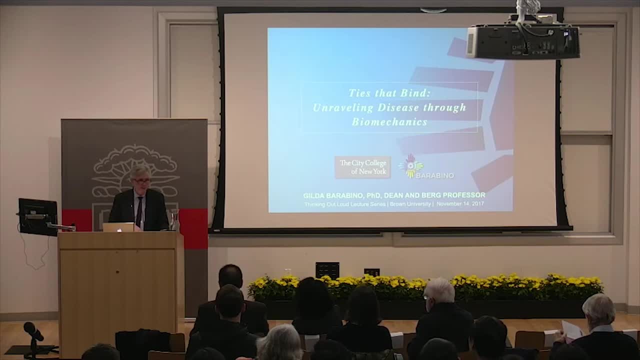 She has a degree in chemical tissue engineering and she also has spoken widely and participated in important discussions around race and ethnicity and gender in science and engineering. As I said, if you go on the internet, you'll see the number of venues she's been invited to speak at. 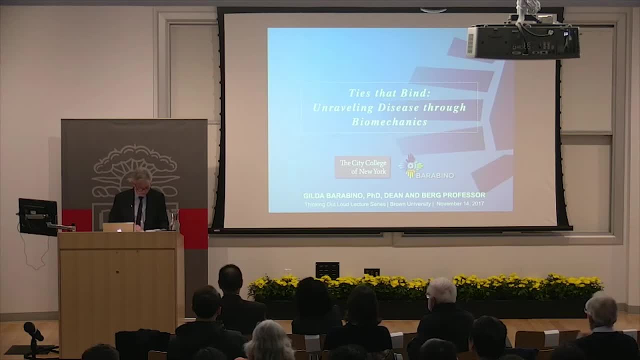 I won't list those here, but I will say that there's some really excellent video interviews of her on the web. if you'd like to learn more about her, Here's some of her ideas about diversity in higher education. Dr Barbino is also the immediate Past President of the BMES, which is the Biomedical Engineering Society. 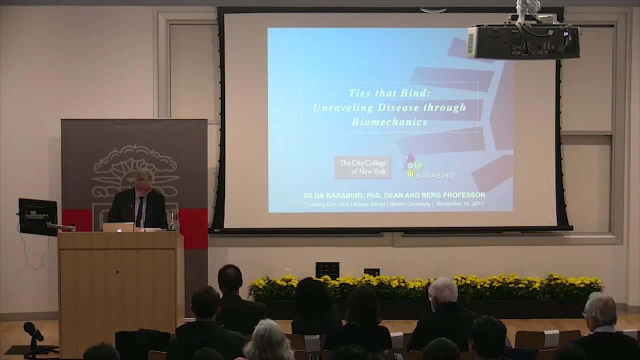 and President-Elect of AIMBE, which is the American Institute for Medical and Biological Engineering. She has over a decade of experience in leading NSF initiatives for women and minority faculty, And she's the founder and executive director of the National Institute for Faculty Equity. 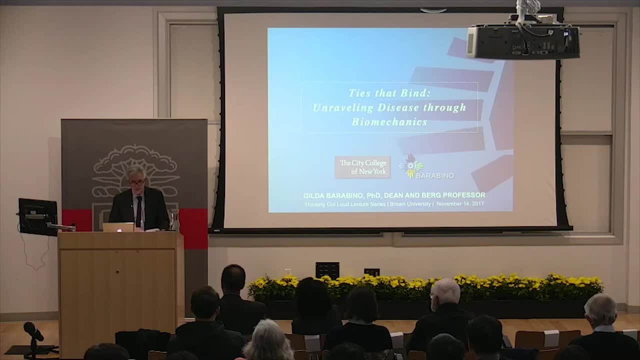 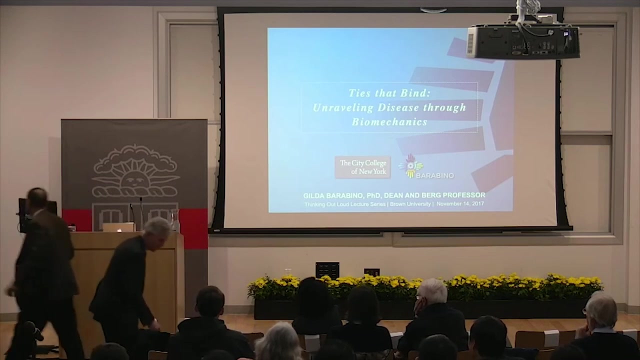 So it's my pleasure to introduce Dr Barabino and before that to introduce Dr Chris Rose, to welcome her as well. Thank you all for coming tonight. Okay, so you know, the first thing that I always ask at these things is how many people have been. 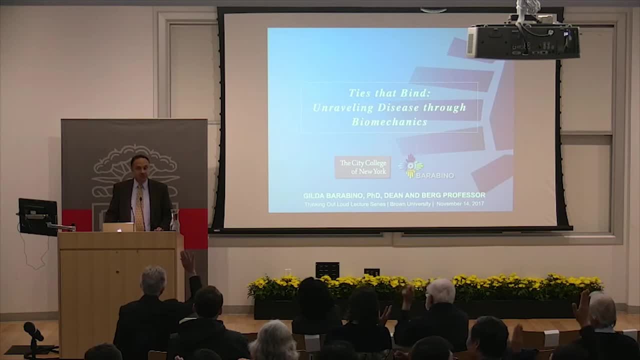 to a Thinking Out Loud before Right. so you know a significant number. So for those of you that haven't been, Rod, have you ever been to one of these? Of course, right, that's a silly question to ask. 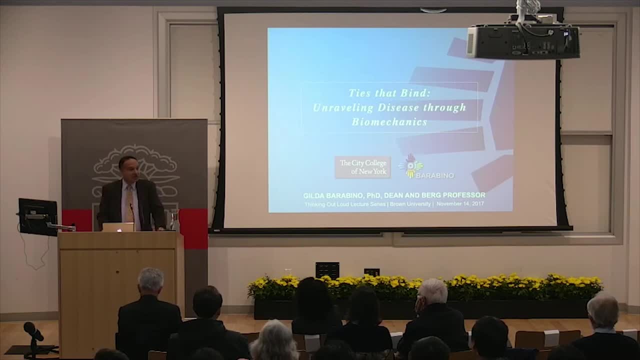 So the interesting thing about this series is that, you know, we did bring all sorts of people in here that were good at what they did, But we're looking for a particular type of mind, one that synthesizes across a variety of different areas. 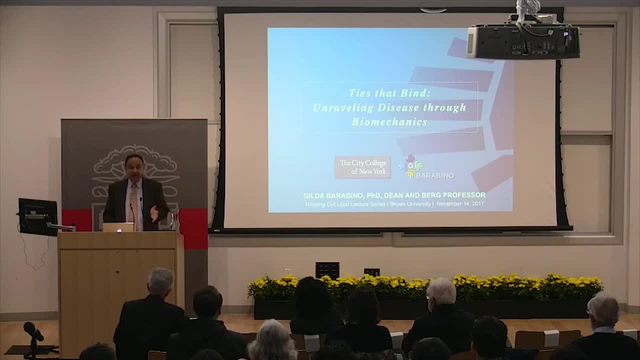 So you know, I knew of Gilda for a long time but hadn't met her actually. you know face to face until today And what I guess I found really interesting about Gilda in particular and as it relates to this series. 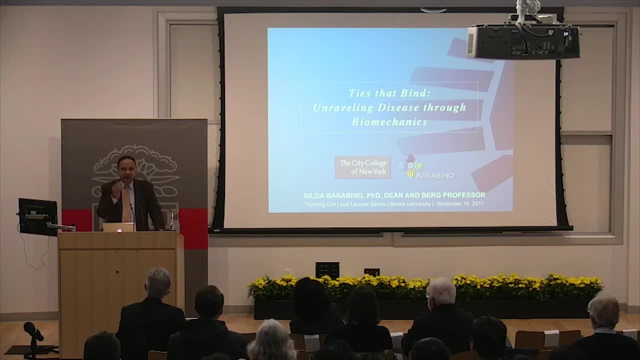 is what I always say for those recidivists here is that we look for a certain kind of crazy right. Honest to God, those are the best scientists: the ones who reach across areas that people never thought were connected and can connect them. 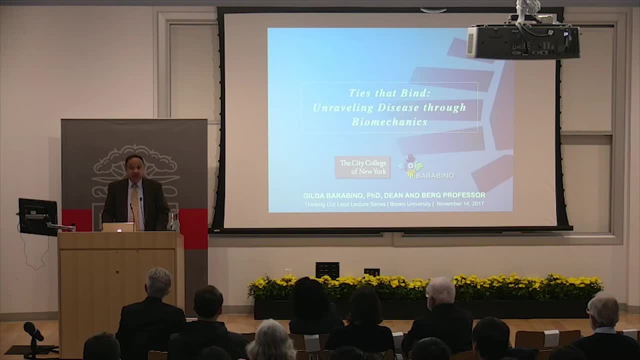 So now, Gilda most definitely fits that bill, but there's this essence. I guess the only way to say it is: Gilda is a warrior. I've never met anybody like her, but she's the most effective warrior I've ever seen. 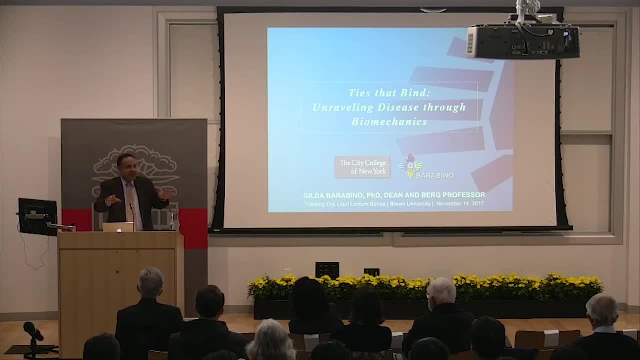 She kind of seeps into intellectual spaces and binds things together, applies what we do as scientists to a variety of different things and somehow it all fits together and somehow she's all still standing. As Kevin said, she's the most busy person. 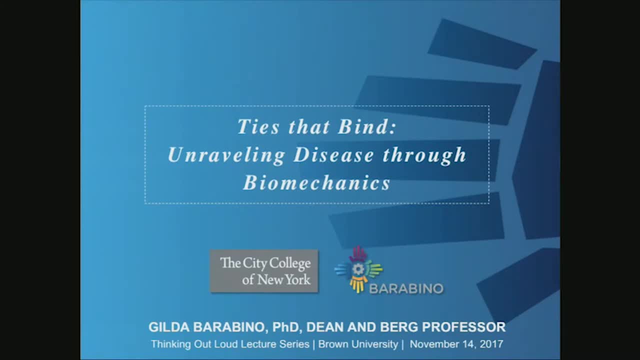 if you look at her CV that you've seen. So you know, with that I guess I'm really kind of I didn't realize how in awe I was going to be, but I'm really in awe. So thank you for coming. 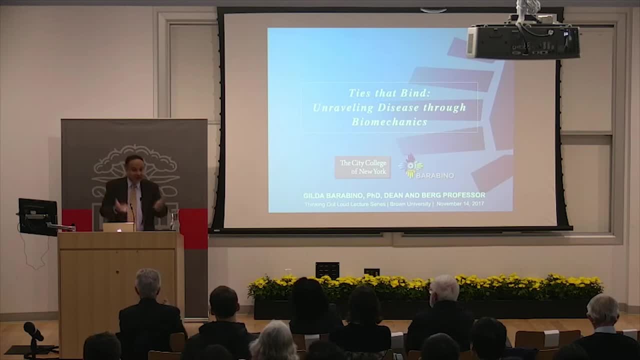 and you know, please help me welcome Gilda Barabino for Thinking Out Loud. Good evening. So first of all I'd like to thank Kevin and Chris for the very kind introduction and the warm welcome. Thank all of you for being here. 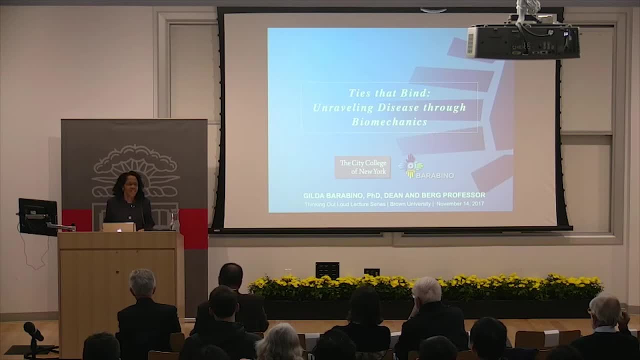 and I'd like to thank Brown University for putting on this distinguished lecture series, and I can't tell you how privileged I am to be one of the speakers in this series Today. I thought I'd tell you a bit about my own journey with the question in mind. 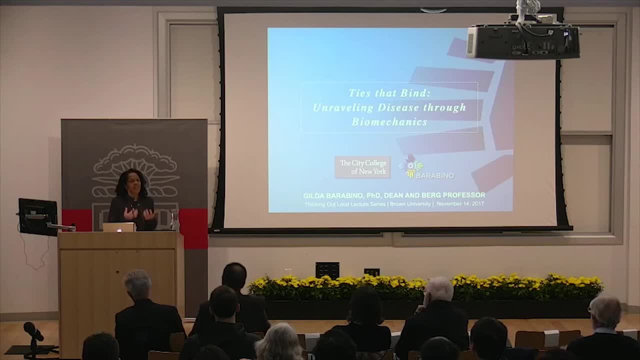 what is it about cell mechanics that can help us unlock the mysteries of disease? And I thought I'd start out by telling you a little bit about my own pathway, too, to come to this question, which has been pretty much my life's work. 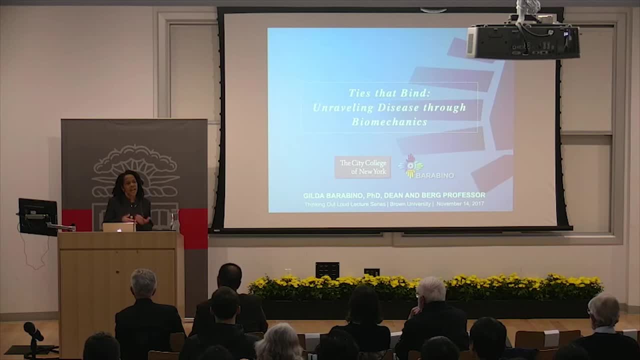 for my professional career and how I have then used that in the work that I've done historically and the work that is going on presently. So my pathway to this work in the area of looking at the ties that bind and how do we unravel disease through biomechanics. 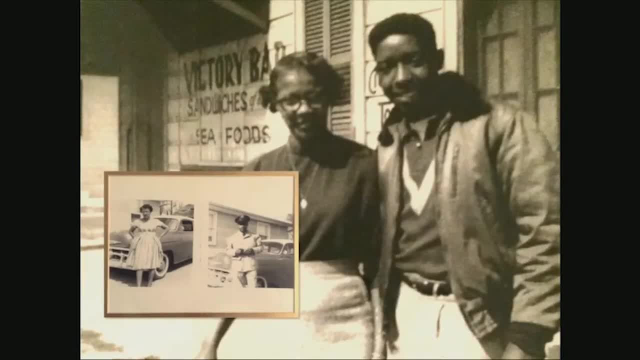 I was born into a military family. My mother and father hail from New Orleans. My father joined the military after high school. I was born in Anchorage, Alaska, and moved around the country, But when my father was ready to retire he moved the family to New Orleans. 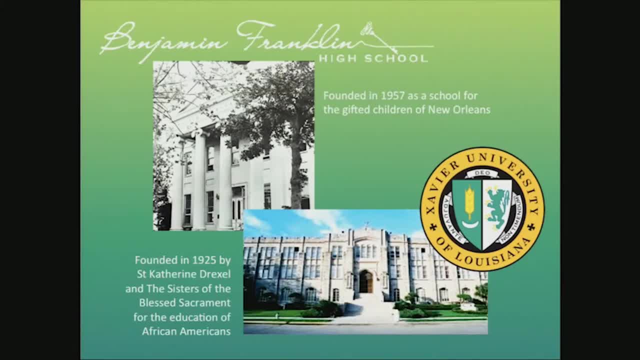 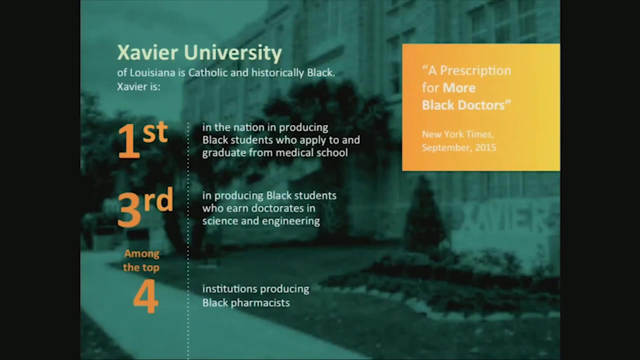 And in New Orleans. I attended high school at Benjamin Franklin High School and I attended undergraduate at Xavier University of Louisiana, And it was at Xavier that I first became interested in medicine. Xavier is very well known: It's the only black Catholic university in the country. 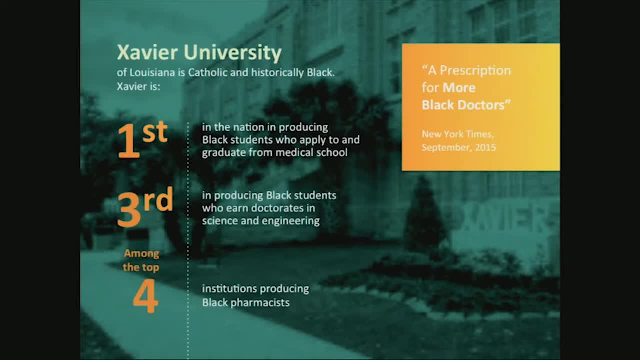 but it's also very well known for producing the most African Americans who are admitted to and finished from medical school. So I started out as a pre-med chemistry major and I was very much interested in pursuing medicine, but maybe not as a clinician. 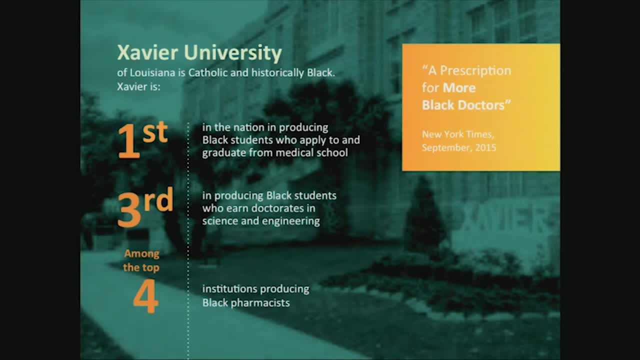 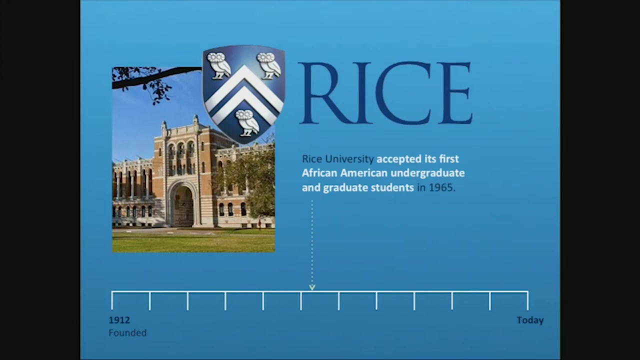 So if you're not interested in doing medicine as a clinician, what would you do to contribute to medicine? So I thought I would approach medicine through engineering. I was the first African American admitted to the graduate program in chemical engineering at Rice University. 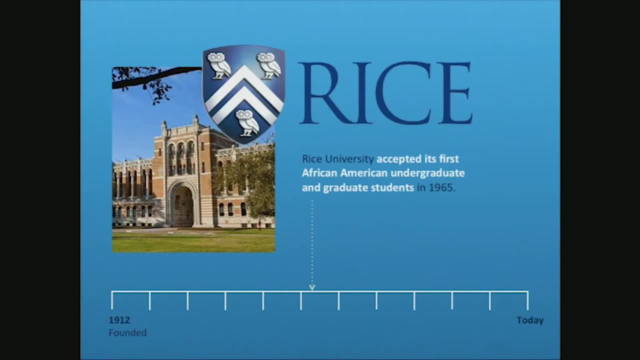 And when I was admitted there in 1981, it was only 15 years after they admitted the first blacks at the undergraduate and graduate level to Rice University. But it was at Rice where I honed my desires and my skill sets and capabilities around using engineering principles. 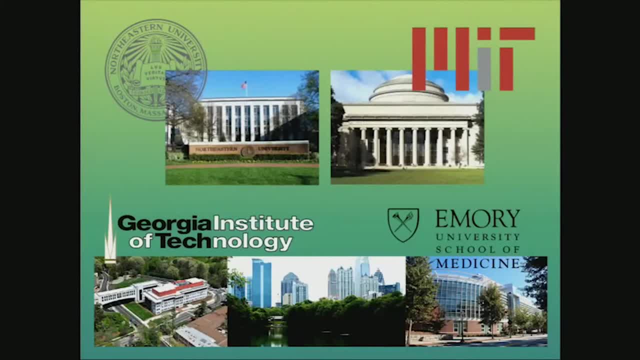 towards problems in medicine. After Rice, I started my academic career at Northeastern And while there, when I was on my first sabbatical, I did it at MIT with Robert Langer and started another area of research- tissue engineering- And I still do some work. 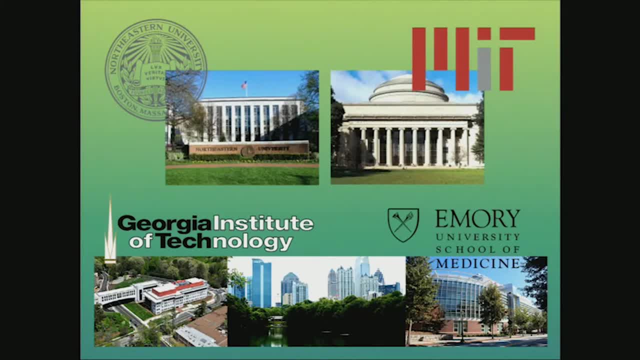 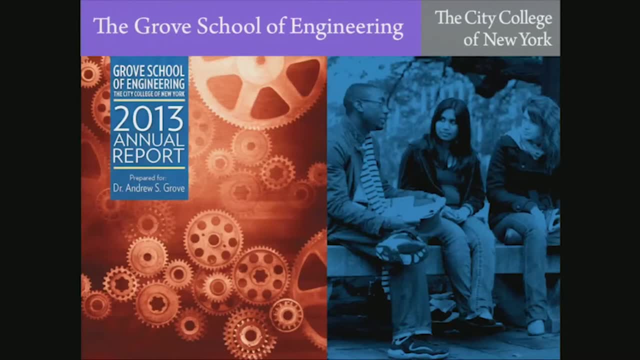 in orthopedic tissue engineering And then, as you've heard earlier, I also was on the faculty at Georgia Tech and Emory and then now currently in my position at the Grove School of Engineering as dean of engineering. But I maintained throughout my career. 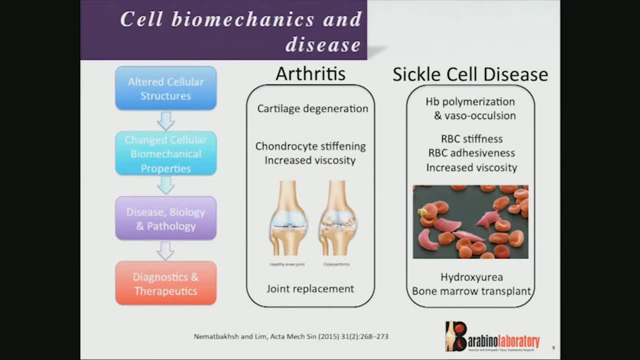 this interest in looking at the connection between cellular biomechanics and disease And it's very interesting that with the onset of disease there's unique cellular changes. There's a lot that we can learn from the changes in mechanical properties of cells that can tell us about. 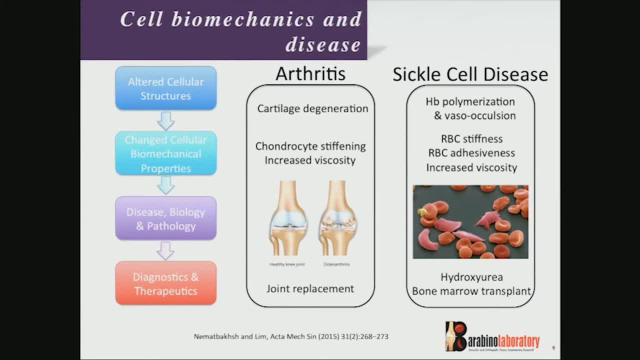 not just how the disease started but how it progresses. I have done works particularly in the context of osteoarthritis and sickle cell disease. So if we look at altered structures and properties in cells as it relates to what happens with disease, 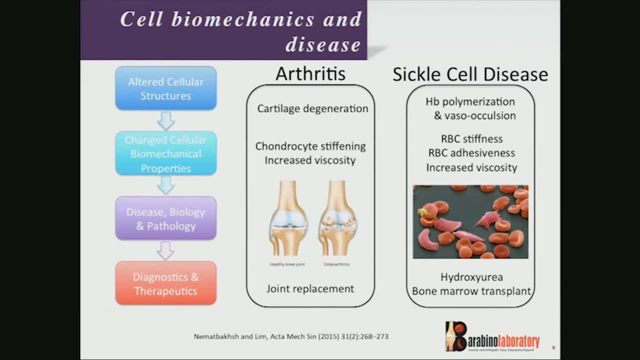 we can learn from that and understand more about the pathophysiology of that disease and that can give us instruction towards therapies. An example of osteoarthritis, for example: we know there's cartilage degeneration- The cell type of course. 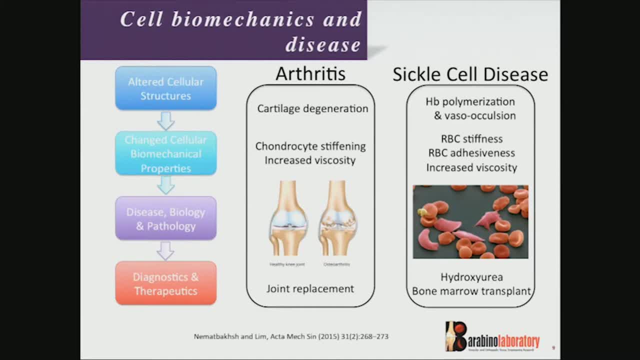 is the cartilage cell, the chondrocyte. Those cells become stiffened of mechanical property We understand. I'm sure many people have problems themselves, maybe with knees, or know of people who have problems with cartilage degeneration. 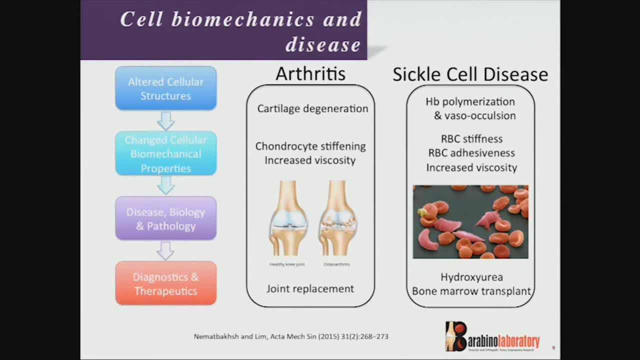 And we know that one of the primary strategies is around joint replacement. I'll tell you more further in the talk about sickle cell disease, but just to recap it, from the point of view of learning about cell biomechanics, there's a defect in terms of polymerization. 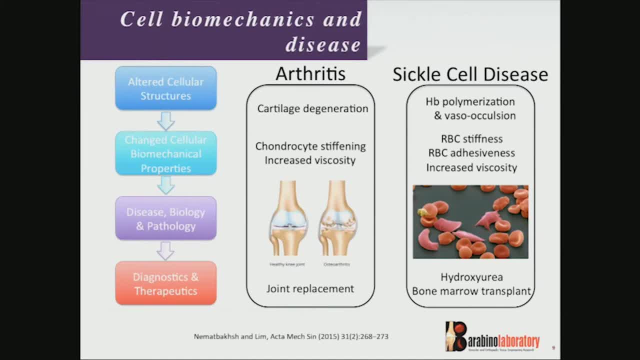 of hemoglobin in the red cell, which leads to problems of vaso-occlusion There. the problem with the cells is the stiffness of the cells and also increased adhesivity of the cells. Blockage of vessels causes a host of problems. 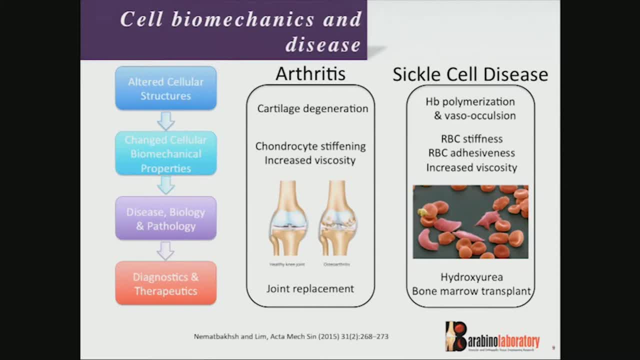 Right now, a primary drug treatment is hydroxyurea. It's a genetic disorder. so many of the therapies that we do they're not curative, but they can address symptoms And there's also one approach that is curative. 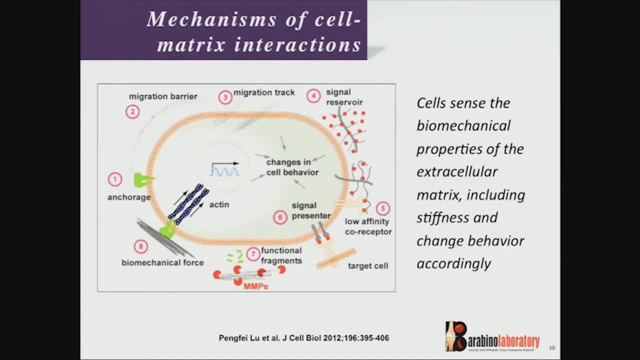 is a bone marrow transplant, So let's talk a little bit more about that. Let's talk a little bit more about the cells. The cells are very adept at sensing their mechanical environments and they interact very well with the matrix that they secrete. 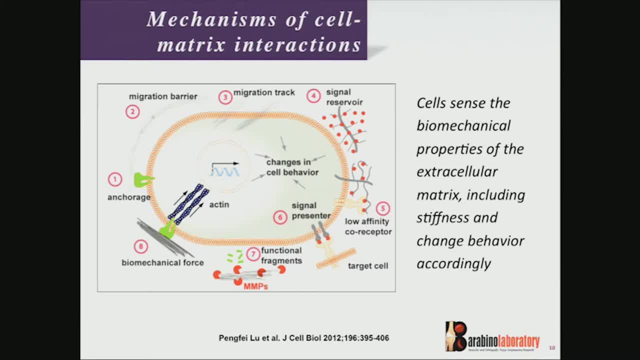 And in particular, because they can sense the biomechanical background, including the matrix and including properties like stiffness, that allows the cells to change their behaviors accordingly. And again, it's those kinds of ways that the cells behave that we can learn from to tell us. 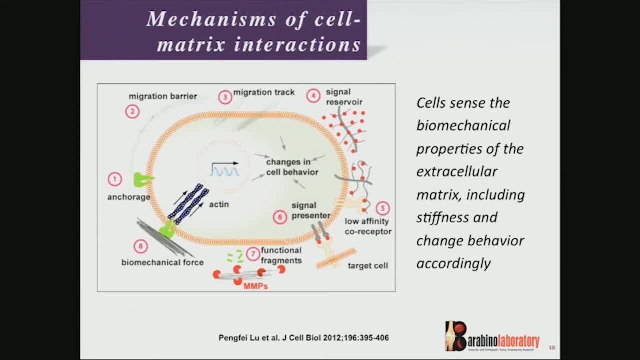 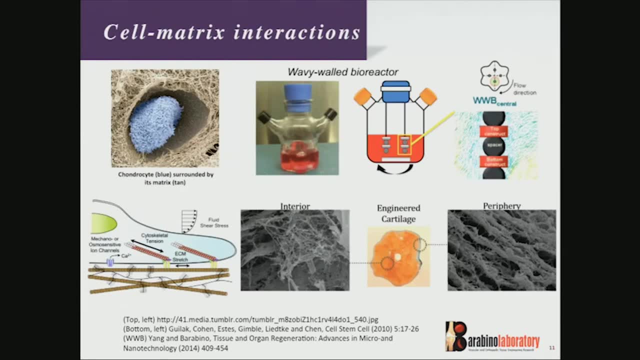 to help us tap into what's going on with the disease. So I'm going to give you some information around some of the studies that we've done in my laboratory around cartilage tissue engineering and use that as an example, by a way, of how cells respond to forces. 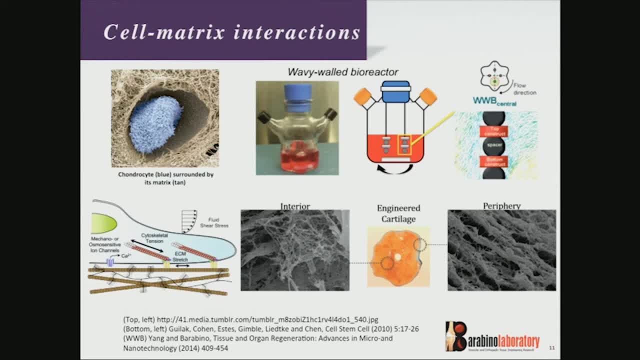 But for the rest of the talk I'm going to focus on using sickle cell disease as a way to explain to you the story and the connection, the interplay between cell mechanics and disease. But for chondrocytes, for example. 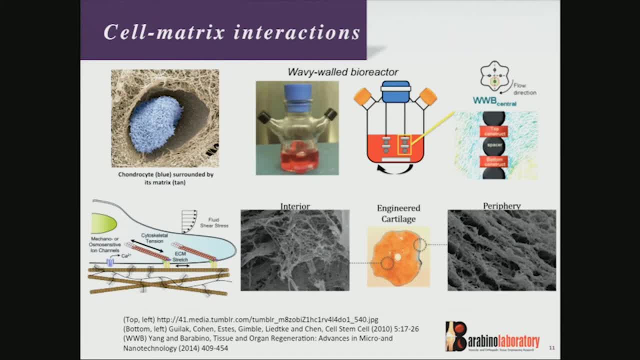 they secrete their matrix in response to mechanical forces, And one of the things that we looked at in particular in my laboratory, we used this novel wavy-walled bioreactor. What this bioreactor allowed us to do was to introduce fluid mechanical environments. 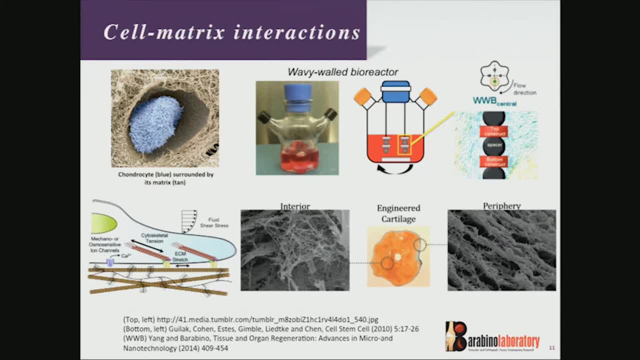 of different types onto growing cells and tissues. So we have these developing tissue constructs where we have cartilage cells seeded onto biodegradable scaffolds. They're in our bioreactors and now they're surrounded by fluid mechanical forces. What we learned from that is how the cells respond. 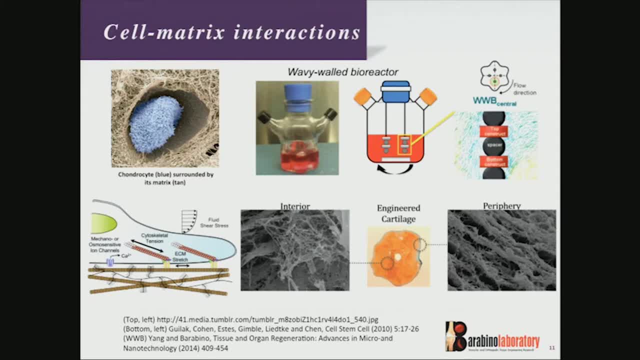 And here's one example. So, in response to the mechanical forces, the cells that were secreting matrix closest to the surface, the ones that are more in contact with the fluid mechanical force, if you look at the, the alignment of the fibers, 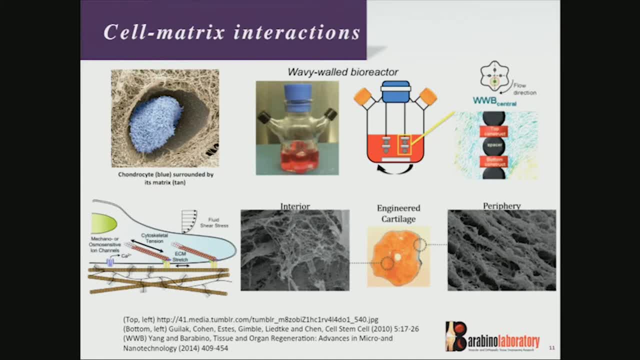 what you'll see, that here, the collagen fibers, that's in the matrix secreted by the cells, are aligned with the flow, But in the interior, where they're further away from the mechanical force of the flow, you see this disoriented arrangement. 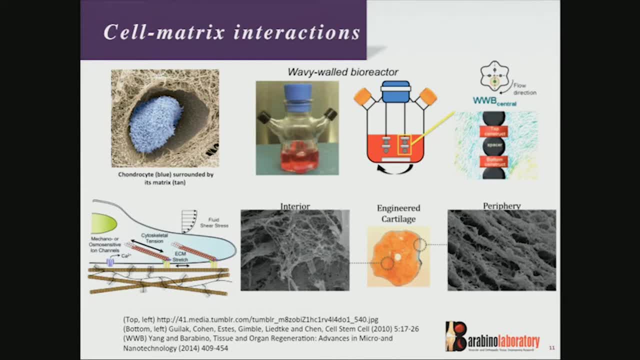 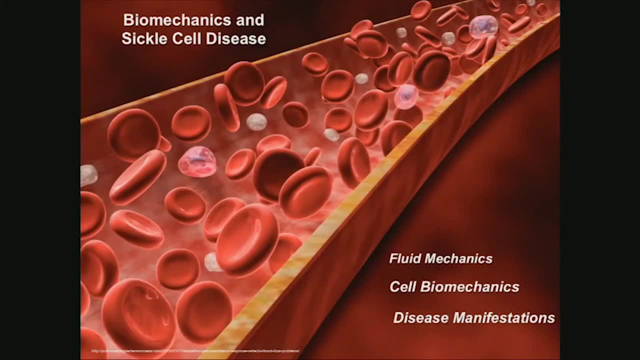 So that's something that we can learn from the mechanics about cellular behavior in response to mechanical forces. So now I'd like to move on and tell you more about the connections between sickle cell disease and biomechanics. To do that, I would like to first give you 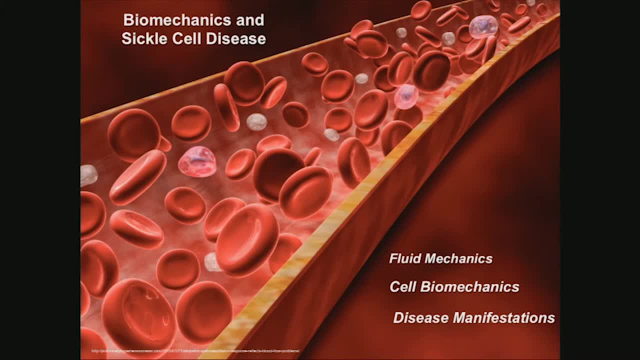 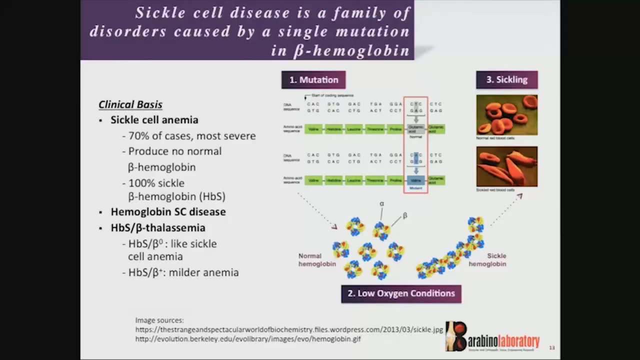 a bit of a primer about sickle cell disease so you'd have a better understanding of how the mechanics works in terms of the interplay. Sickle cell disease is actually a family of disorders with abnormal sickle hemoglobin And the defect basically is there's one amino acid. 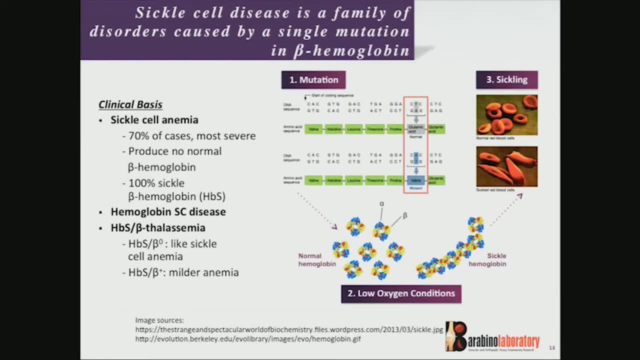 substitution in the beta chain of the hemoglobin molecule, and that one amino acid substitution causes the hemoglobin molecules to, rather than stay separated, to aggregate under deoxygenated conditions, And what you then get is cells that are now sickled in shape. 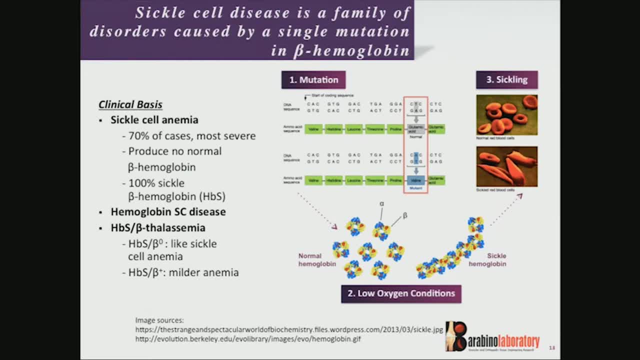 because of the polymerized hemoglobin and that causes a whole host of problems. There are other diseases that there's sickle hemoglobin, but not just sickle hemoglobin, There's also There's SC, so there's sickle hemoglobin and C hemoglobin. 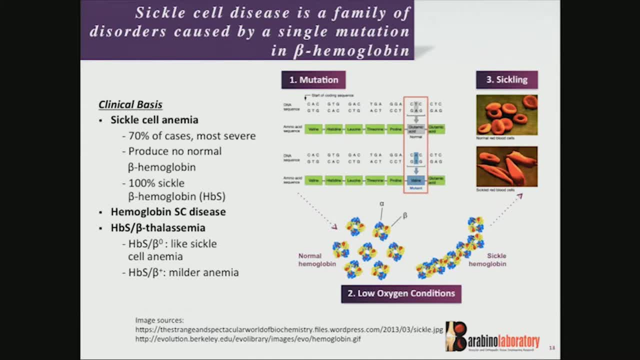 as well as thalassemia. The most prevalent would be sickle cell anemia, That's all sickle hemoglobin, And I'll tell you a little bit more about the disease so you can understand the importance of better understanding the pathophysiology. There's 3.2 million people who have the disease worldwide, 100,000 of which live in the United States, And there's an economic burden associated with the disease. About a million dollars is the estimate for the total lifetime of health care costs. 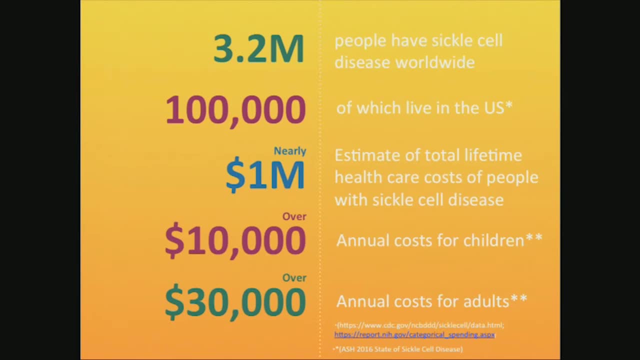 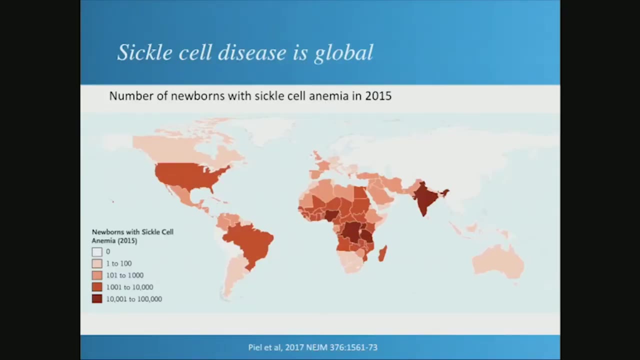 Over 10,000 for annual costs for children and 30,000 annual costs for adults. Sickle cell disease is global and in this chart what you see is the number of newborns with sickle cell anemia across the world in 2015.. 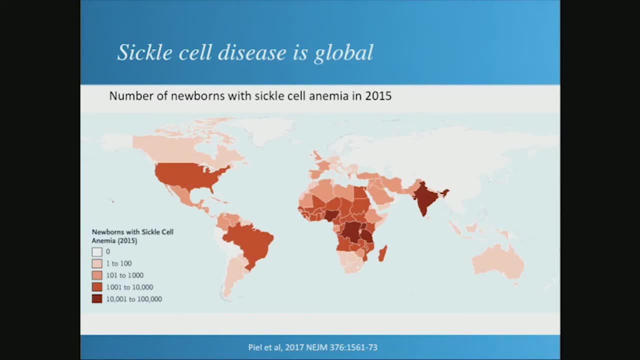 And you see, the darker regions have a higher incidence of sickle cell disease and it's not surprising that there's a higher incidence in equatorial regions. The disease was thought to be a mutation that evolved in response to becoming a protection to malaria. 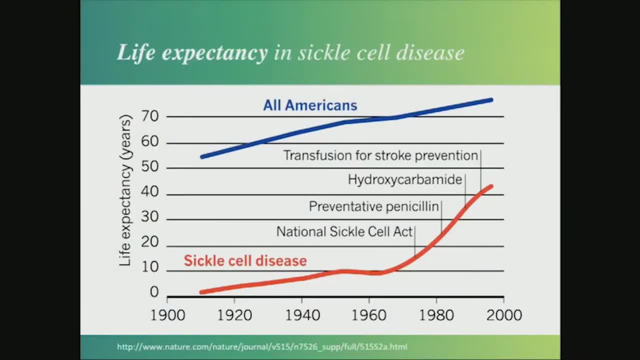 I'd like to tell you a little bit more. If you think about how the disease is manifested and what happens within society. looking at the life expectancy for sickle cell disease, the average age is about 40 for life expectancy, or mid-40s. 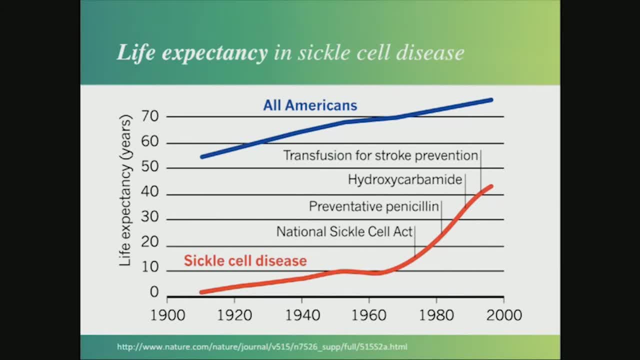 and it's slightly higher for women than men, about 45 versus 43. And I'd like to draw your attention to a number of things that have happened over time. In 1972 there was a national sickle cell act. It was passed by Congress. 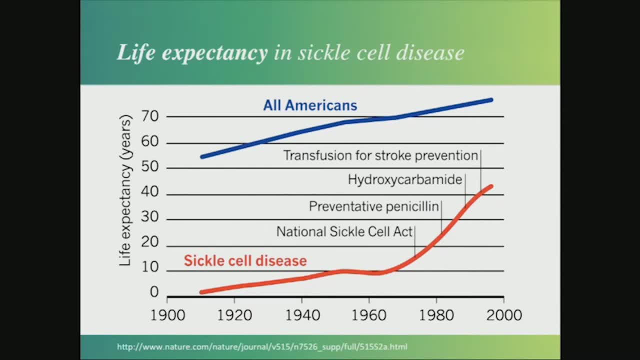 and that act actually was directed towards having more research, education, training and screening around sickle cell disease. At that time I was in high school and I remember there were a number of community activities. There were fairs, health fairs. 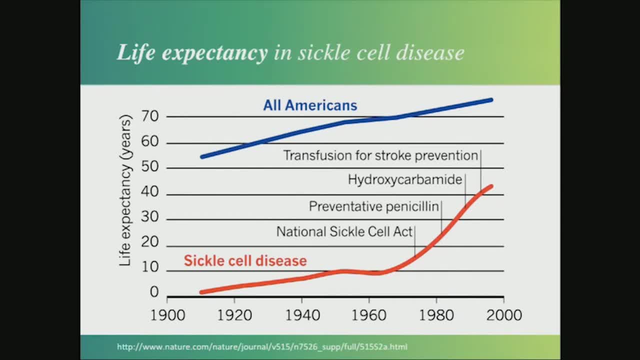 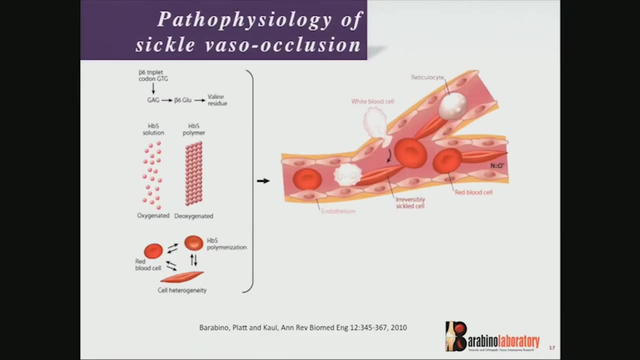 where there would be screening around the disease. But even with all of the studies that have been done and as much information that we know, there's still a lot of unanswered questions and I will bring it back to looking at biomechanics to answer some of those questions. 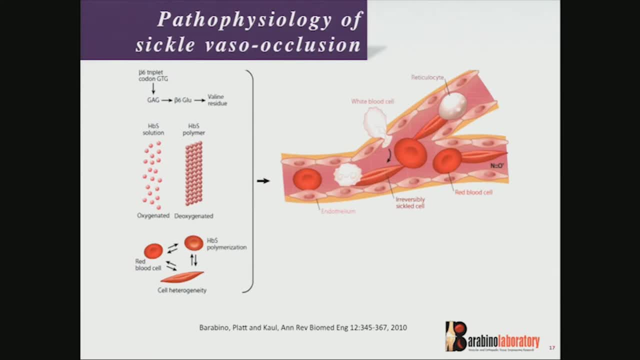 If we look at the pathophysiology of the disease, we need to understand that the hemoglobin polymerization that's present in the body, that's in response to this genetic defect, the one amino acid substitution causes these cells to take on a sickle shape. 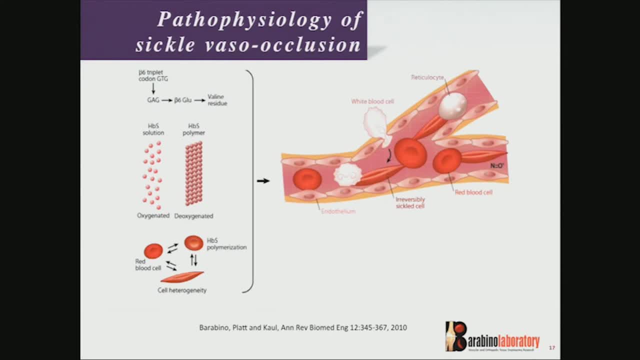 The polymerization that happens under deoxygenated environments is actually reversible, so that at any given time cells with sickle hemoglobin can go from oxygenated to deoxygenated sickle to un-sickle After repeated cycles of sickling. 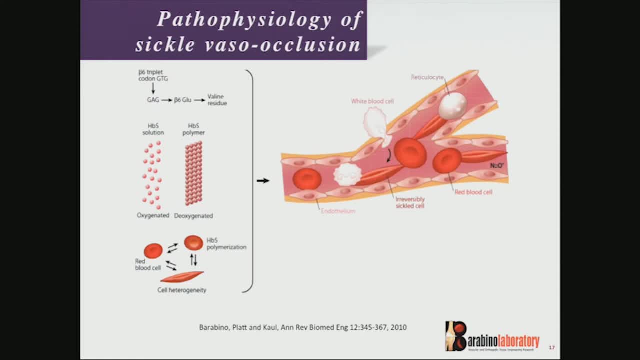 many of these cells become irreversibly sickle and cause a number of problems in the circulation. So if you think about a sickled cell, hemoglobin polymerized and the difficulty that it might have in the circulation in comparison to a normal cell. 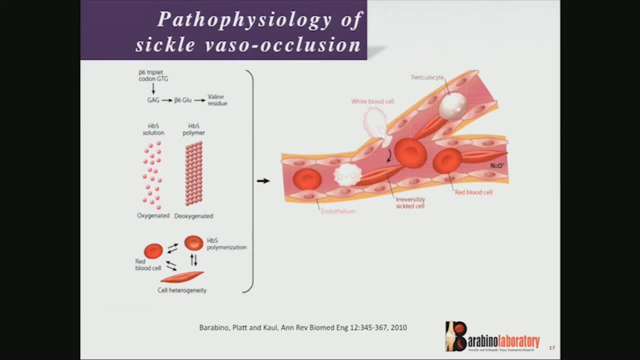 it's amazing in terms of properties. So a normal red blood cell. nature has this fantastic design for the normal red blood cell. It's a viscoelastic membrane, biconcave shape, and it surrounds an aqueous solution of hemoglobin molecules. 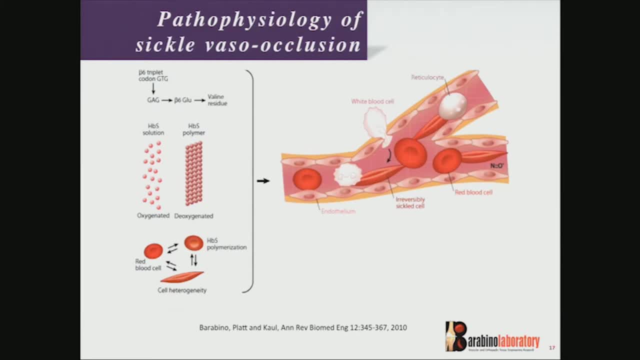 That normal red cell is about 8 microns in diameter and that structure I just explained to you allows that red cell to be extremely deformable. it's not stiff and it can fold over on itself and pass through vessels, capillaries, for example. 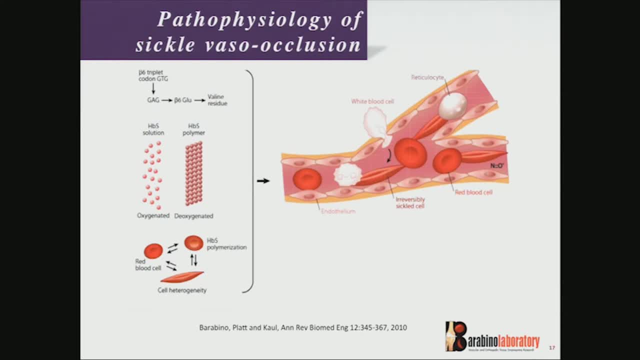 that have a diameter that's half the size of the diameter of a red cell. So that's something that we can learn from looking at normal situations and then looking at the disease state that deals with it. It deviates from normal. We also found that for sickle cells. 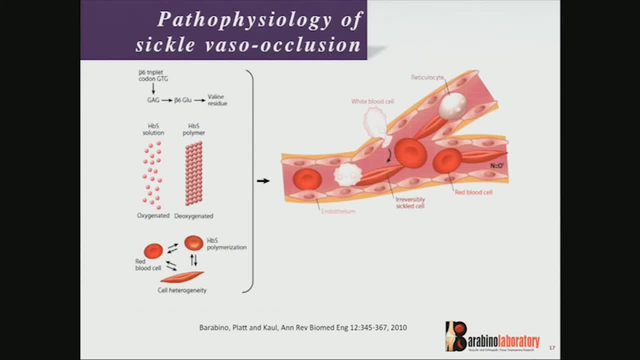 the sickle red blood cells. not only were they different in stiffness, in the way that they can block vessels. because of stiffness, they also are abnormally adherent, so they can adhere to each other, and they can adhere to the endothelial cells that line the vessel walls. 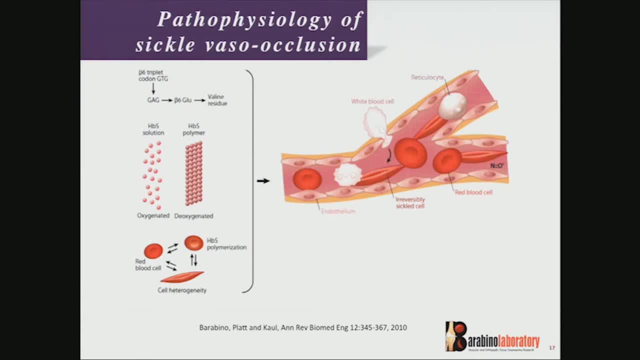 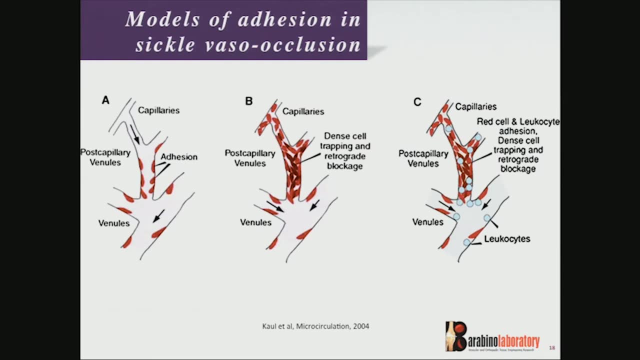 So you have a problem not just mechanical obstruction of a vessel, but also related to adherence. So we have models of adherence where you can have sickle red blood cells adhering to a vessel wall and maybe not causing a blockage, just by itself adhering. 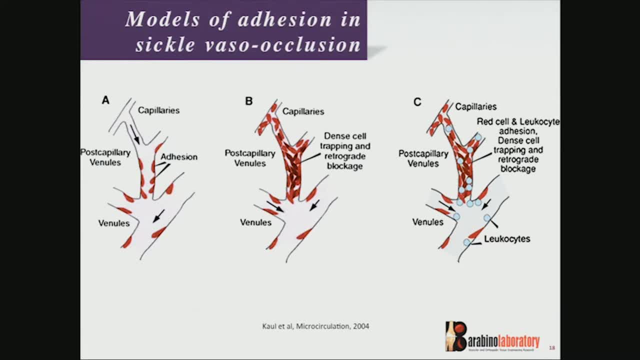 but if they adhere over a period of time and then there are other cells that come behind them that now cannot pass through the circulation because they're adhering or interacting with these cells that adhere to the vessel walls, you have another form of blockage. 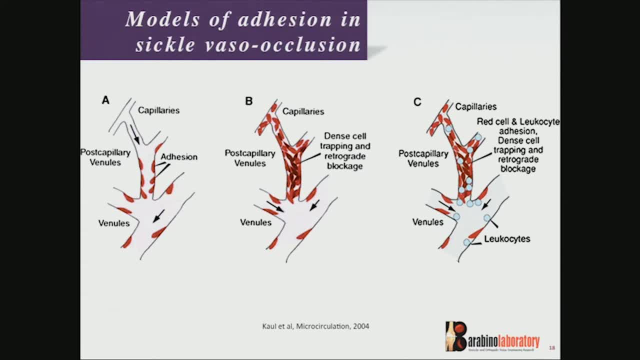 And so that's what this one shows you And this third model says. not only can you get trapping related to sickle red blood cells adhering, other blood cell types, like a white blood cell, could participate in the blockage, and we are trying to understand that as well. 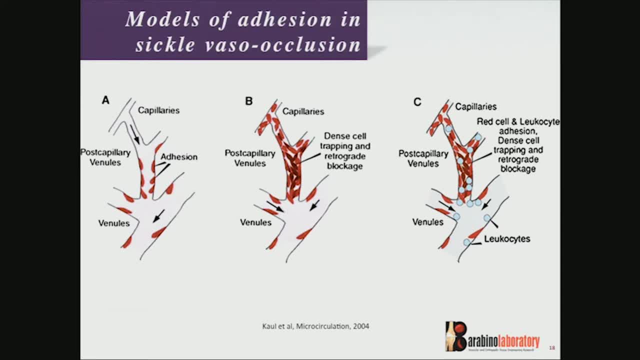 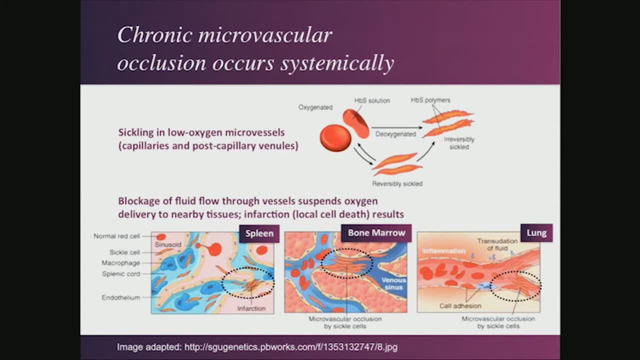 So, before I talk to you about some of the engineering approaches that we've taken, I want to give you a little bit more of a sense of the manifestations of the disease related to the vascular occlusion which is the hallmark of the disease. It occurs systematically. 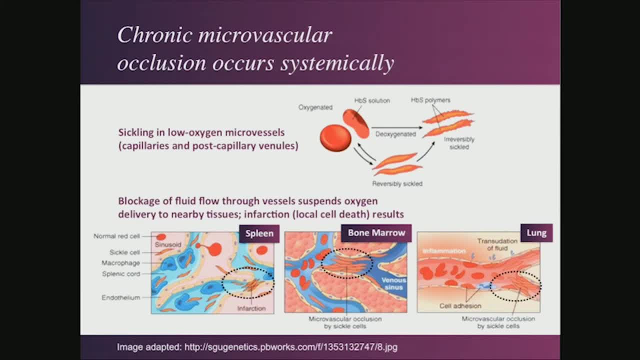 Since the red cells are responsible for carrying oxygen to the tissues. if there's a defect in that and they're no longer able to carry the oxygen to the tissues the way they normally do, because vessels are obstructed, the oxygen doesn't get to the tissues. 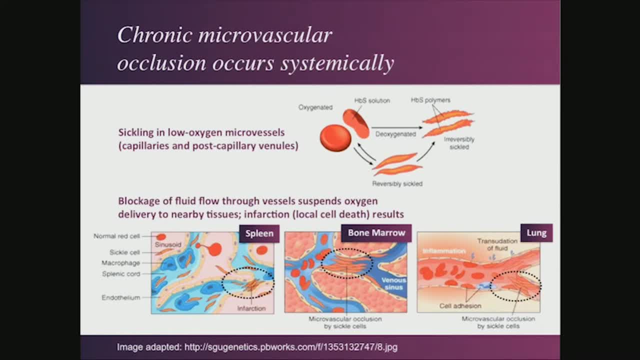 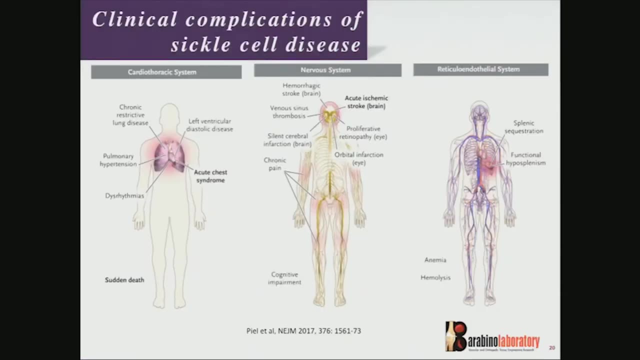 What happens to the tissues? They die basically. So now you've got organ damage And the more an organ has small vessels that are more prone to blockage, the more organ damage that you'll have. So some of the clinical manifestations that you see in the different systems: 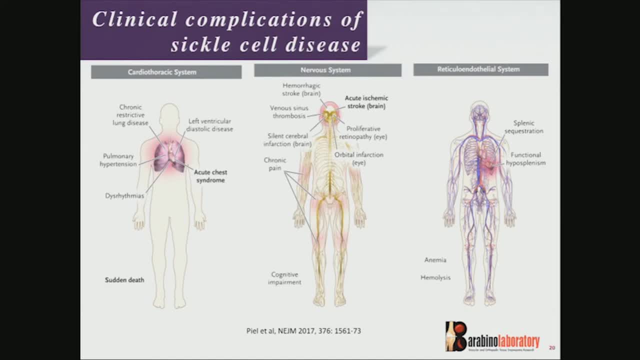 one in particular in the cardiothoracic system was acute chest syndrome. There's also other things that happen when you have vessels blocked in the brain, for example stroke. There are things that happen in the reticulothelial system like spleen sequestration. 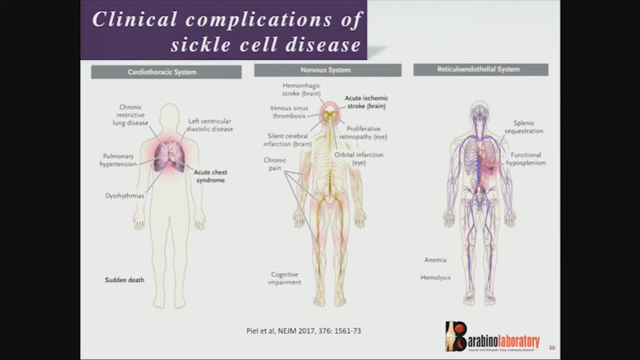 The spleen has so many small vessels that in sickle cell patients their small vessels and capillaries in the spleen become so blocked that they're effectively spenectomized. It's like they don't have a spleen, And then in other systems. 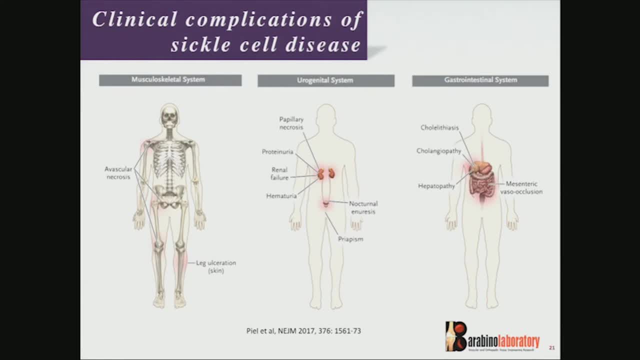 there's problems in the musculoskeletal system, particularly in blood circulation within bones. You have what we call infarcts in the bones. You're not getting oxygen to the tissues. Patient experiences that as extreme pain. There's also problems in the urogenital system. 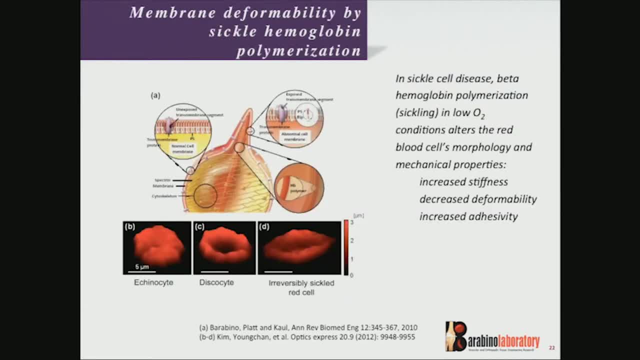 and the gastrointestinal system. So let's tie this back to cell mechanics. When the structure within the cell and you have hemoglobin polymerizing within the cell, it often pulls at the membrane And for sickle cells you now can have proteins. 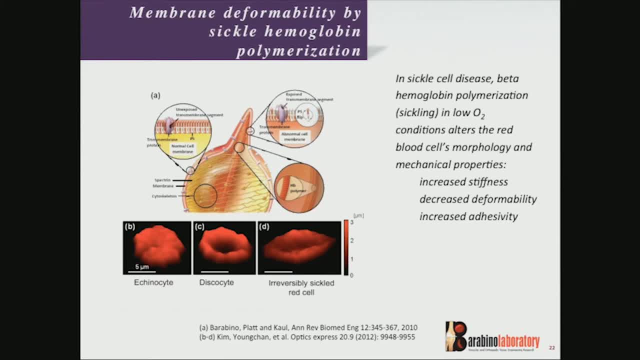 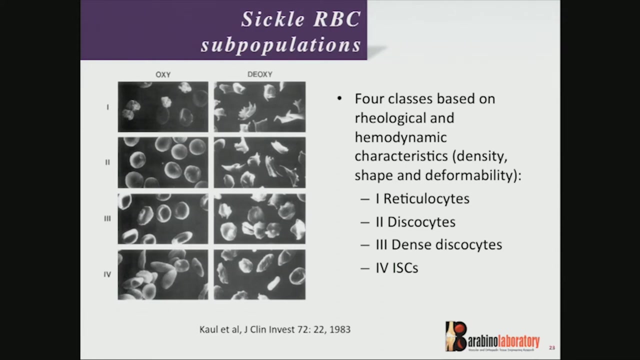 that normally might be embedded and not be exposed, be exposed because of that sickling process. You have cell shapes and changes and it absolutely makes a difference in terms of mechanical properties like stiffness, deformability and adhesivity. We also know that it's not even just one particular cell stiffness. 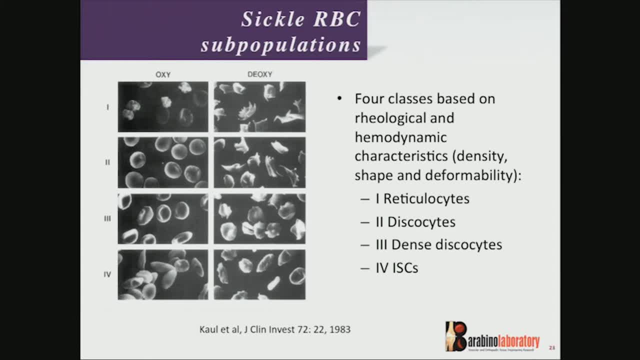 or cell shape that's prevalent in sickle cell disease. So we've classed that there's actually four different classes based on their biomechanical properties and their density. They can be young cells or reticulocytes, which are the young red blood cells. 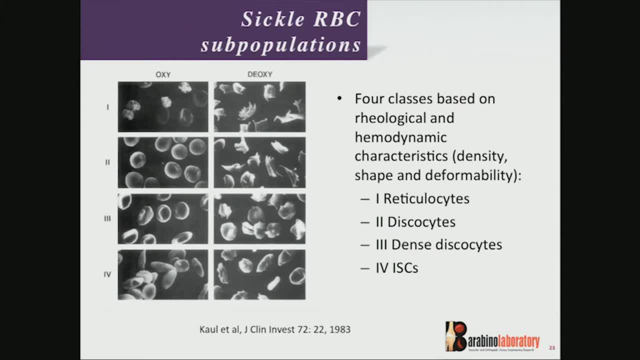 that are coming right out of the marrow. they tend to be more deformable and less of the hemoglobin polymerization. There are discocytes. there's dense discocytes and the ones that I mentioned to you that are permanently damaged, that are irreversibly sickle cells. 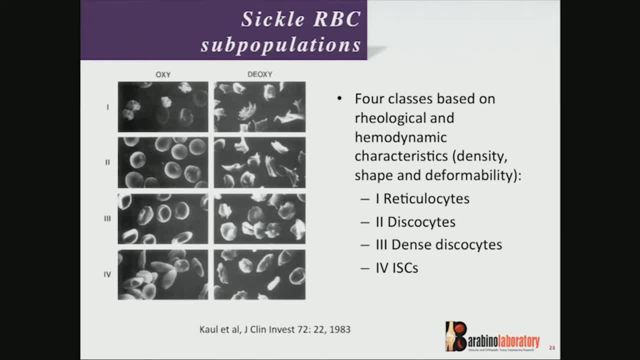 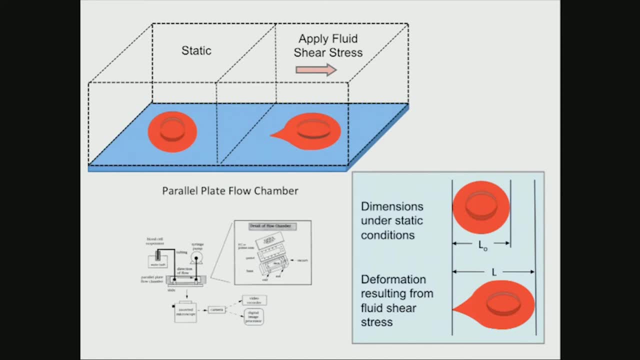 So we're interested in those populations of cells as well. Now we want to use an engineering approach so that we can exploit these mechanical properties, and we can also exploit fluid mechanics to better understand what's happening in the disease. So what we've used over time, 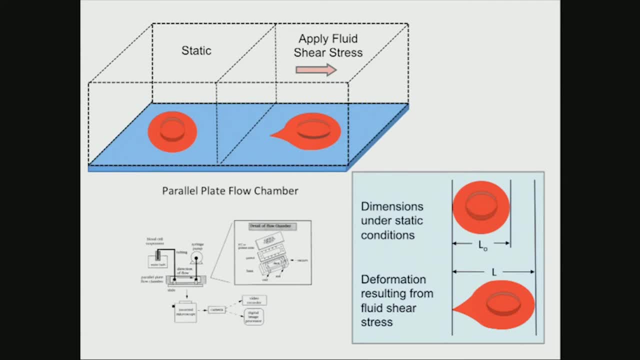 is a parallel plate flow chamber system, So the parallel plate flow chamber is mimicking a vessel. We can culture endothelial cells that line the vessels on these plates and then we can perfuse them with blood samples or blood suspensions to mimic what's happening in the vessels. 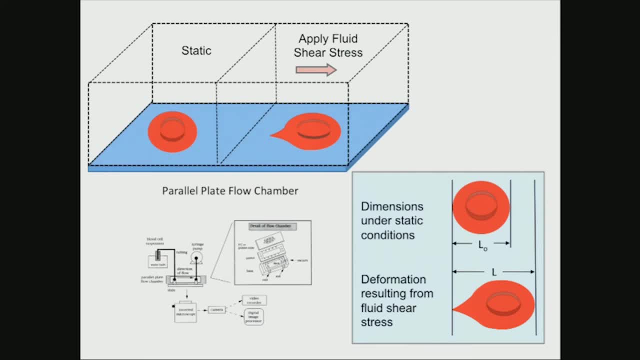 We can take advantage of. we know what happens, what it looks like, statically apply shear stress and we know there's going to be this deformation in response to stress. but we can also use this flow system to look at adhesive properties, And much of my early work was devoted to. 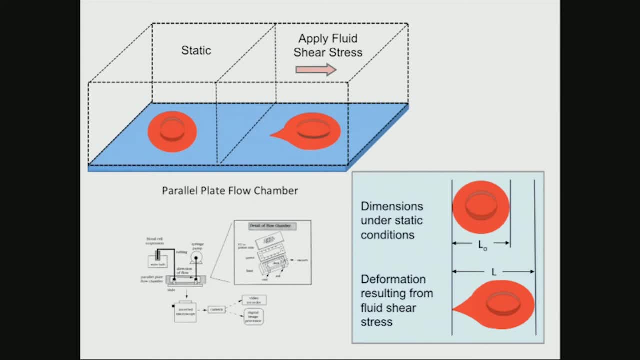 how do we understand adhesive interactions between individual sickle red blood cells and the endothelial cells lining the vessels in a way that it's going to give us some clues towards what's happening with vaso-occlusion and maybe actually help us have predictions around when a patient might be? 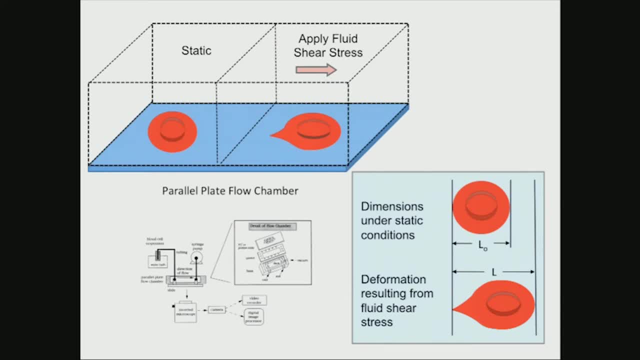 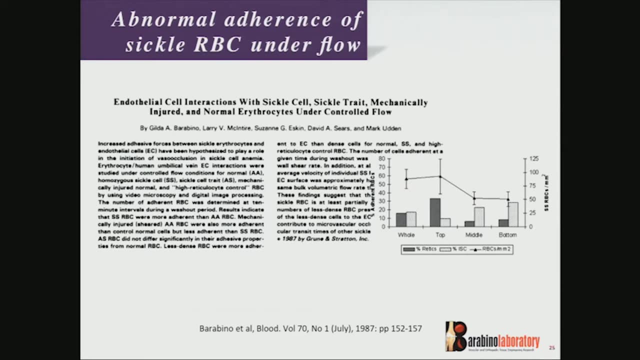 headed towards a crisis, which is when the vessels are completely blocked. So one of the earliest studies that actually came out of my thesis was we looked at a combination of cells that were from patients living with sickle cell disease. We also looked at red blood cells that were normal. 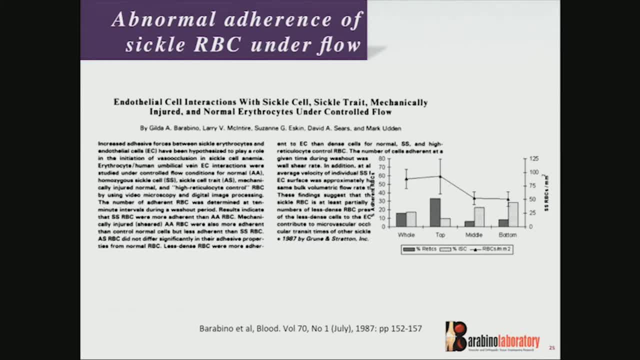 but we mechanically damaged them. And we mechanically damaged them so that they would have mechanical properties similar to sickle cell properties And the damage mostly was within the membranes. And what we found in looking at those cells, as well as cells- red blood cells- 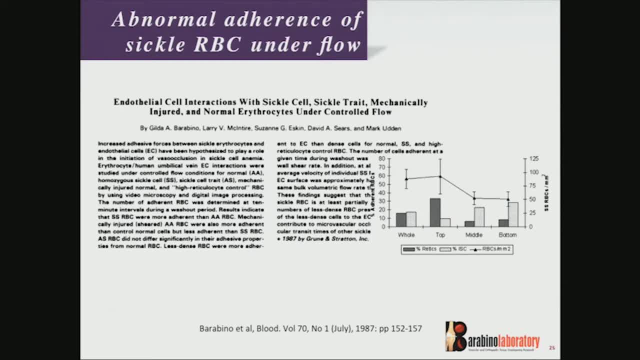 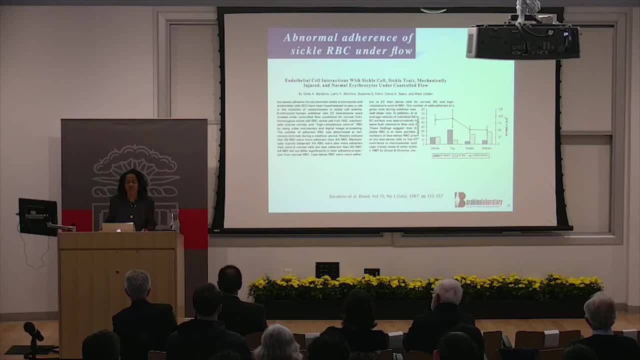 from people who were not patients. they were carriers of the disease sickle trait, And what we found was that the most adhesive, that of course you would expect to have the most problems with vaso-occlusion were those for sickle cell patients. 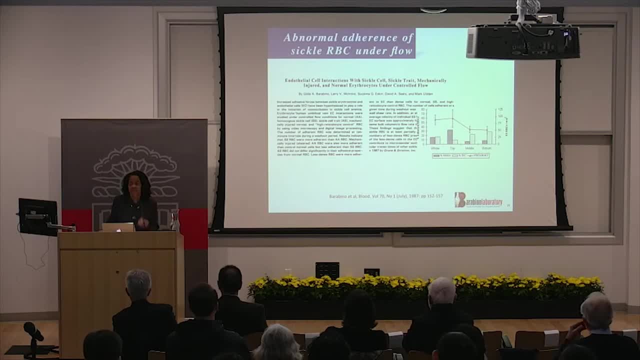 When we looked at the separate. I told you there were the separate categories based on the density and the stiffness of the cells. When we looked at the separate categories, what we found was that the younger more deformable cells, the reticulocytes. 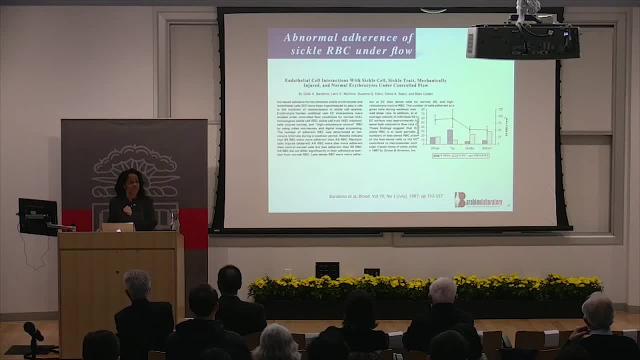 were more adhesive than the more damaged cells. This was in contrast to what had been seen through static adhesion assays, because the static assays said that the more damaged cells were actually more adherent. The lesson that we learned there is that you need to do these experiments. 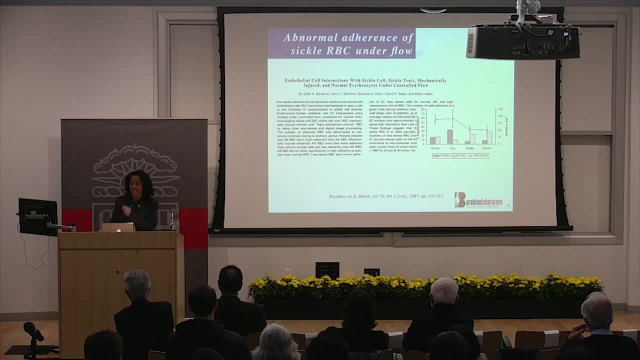 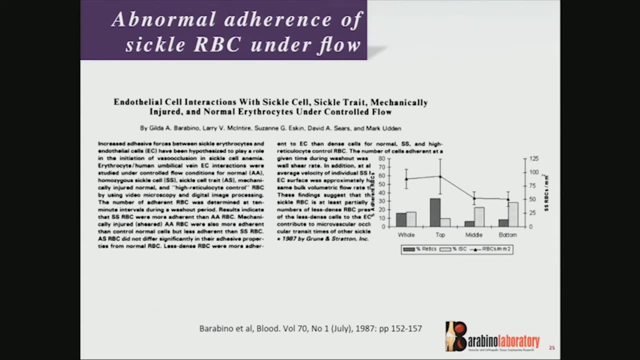 under physiological flow conditions. The static conditions did not tell you enough about what's happening in the physiological sense. So we found that under dynamic conditions that mimic those in the body- the reticulocytes, the younger cells- which was not what you were expecting. 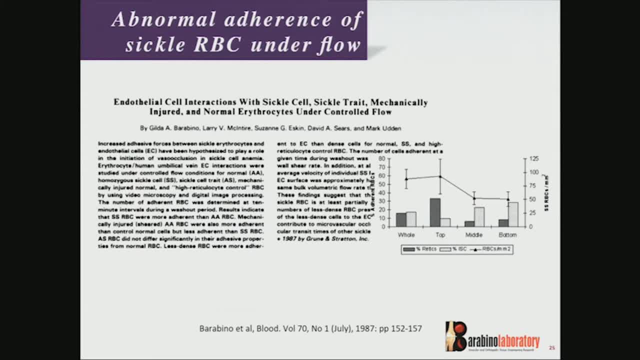 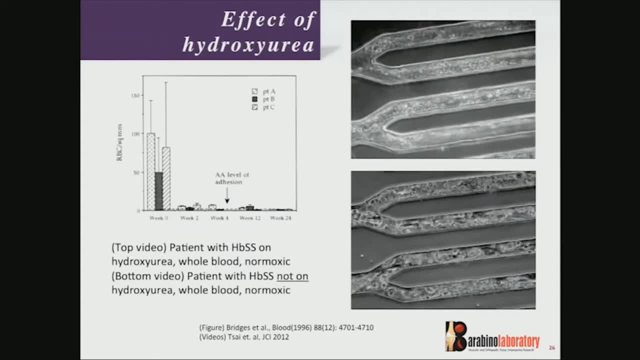 were actually playing a bigger role in vaso-occlusion. So when we look at other aspects as it relates to therapies, what I want to show you here is one of the drug treatments. So it had been for quite a period of time. 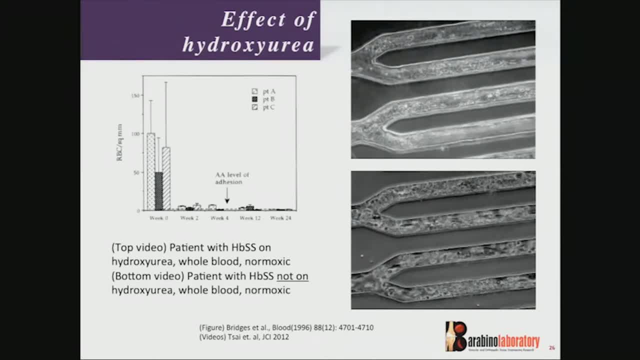 only one FDA-approved drug for sickle cell disease, and that was the hydroxyurea. Only recently there's been another drug approved and that's a glutamine that's only recently been approved, But for the most part, one of the major therapies. 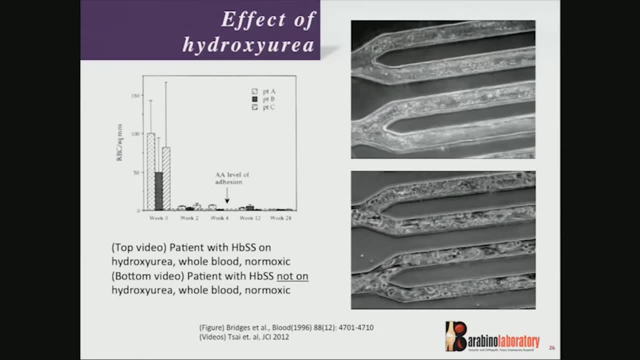 that was afforded to sickle patients was hydroxyurea. So in one of these early studies, we were trying to better understand using this system. what's the mechanism? How does hydroxyurea work? It doesn't work for all patients. 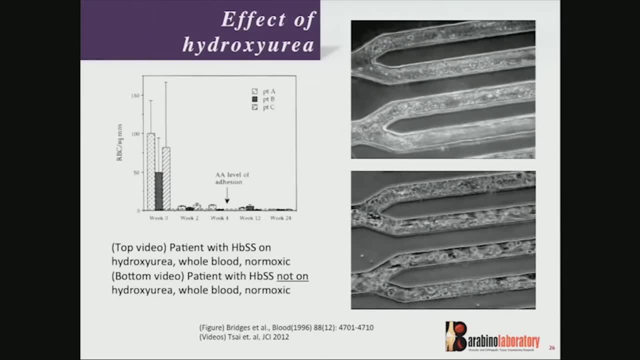 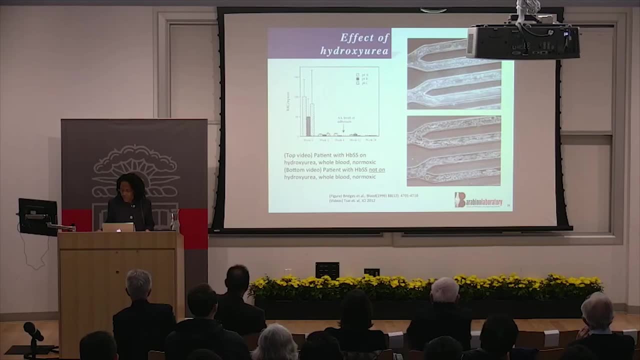 and it doesn't work all the time, But patients who were on hydroxyurea the urea had less vaso-occlusive crises, And so what we found in this study was that those who We looked at adhesion for those. 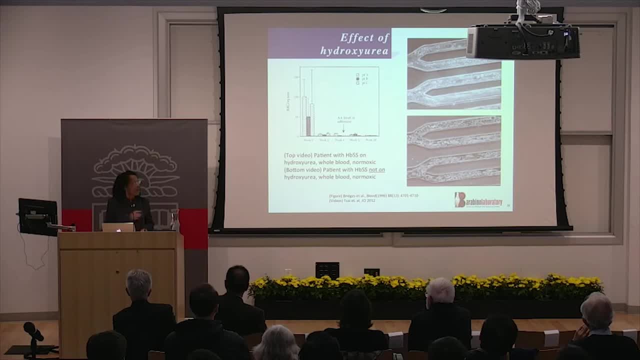 before they were on the drug and then after they were on the drug. And what was shown here is as early as two weeks after drug treatment their adhesion went down to levels of normal And what you see here in this flow in microfluidic device. 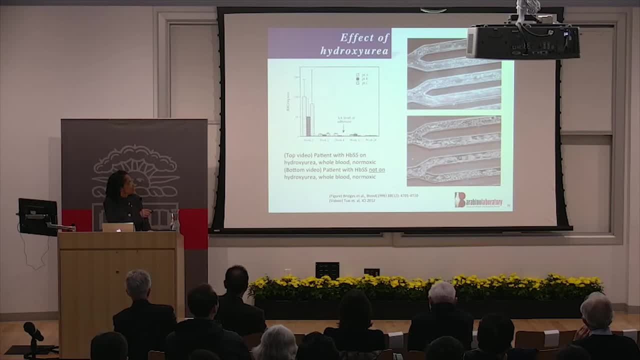 this one is for a patient who is on hydroxyurea And see the difference between that flow and the flow here where the patient is not on hydroxyurea. So we're learning something about the fluid mechanics and how there's a response to drug therapy. 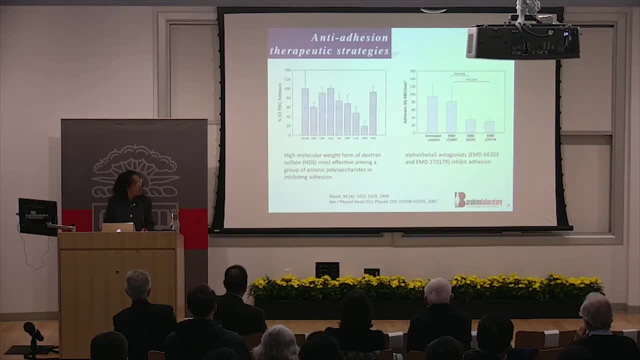 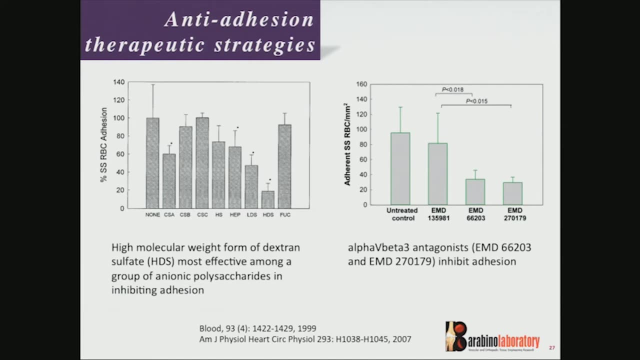 from that work. Another thing that we were using to look at therapeutic approaches by understanding the fluid mechanics of the system was we know that we can better understand the interactions between the sickle cells and the endothelial cells line in the blood vessels if we understand the molecular mechanisms. 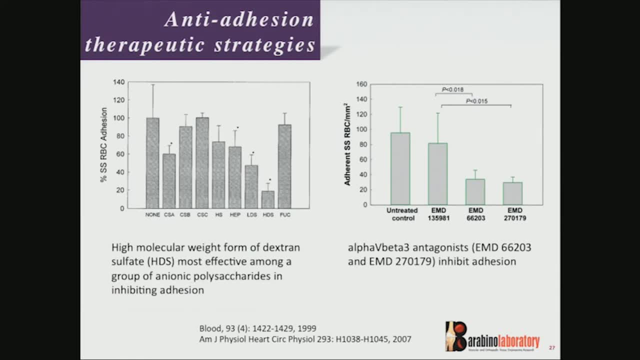 So what molecular mechanisms are accounting for the adhesion? So what about the surface of the red cell and the surface of the endothelial cell? So in one study we looked at anionic polysaccharides as a way to be an anti-adhesion therapy. 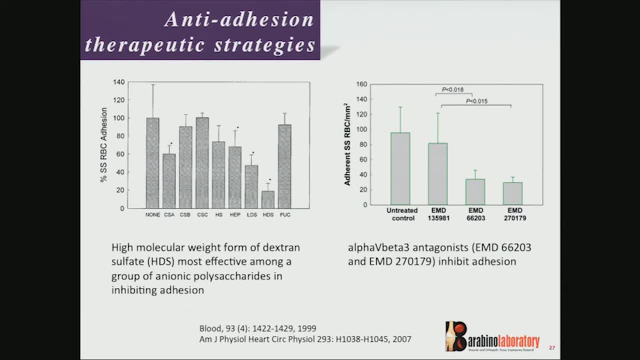 because it turns out, sulfated glycol lipids that can be exposed on the membrane of a sickle red blood cell. they may not necessarily be exposed. normally they can be inhibited by anionic polysaccharides. So in this study what we found was that 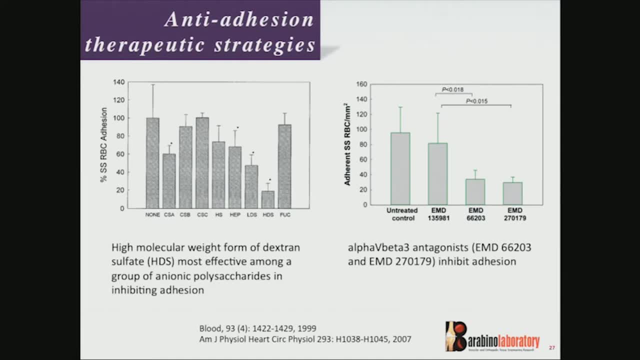 this one particular anionic polysaccharide, this high molecular weight form of dextran sulfate, was very effective in blocking adhesion. In another study we looked at a receptor on the endothelial cell that was called alpha-V-beta-3 and saw that antagonists to that receptor 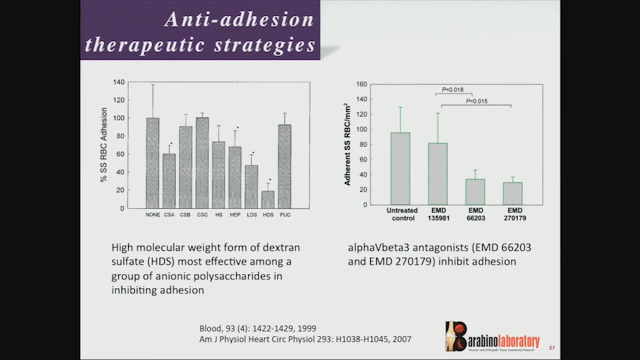 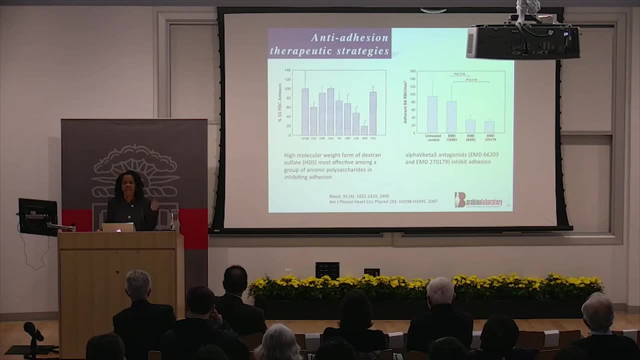 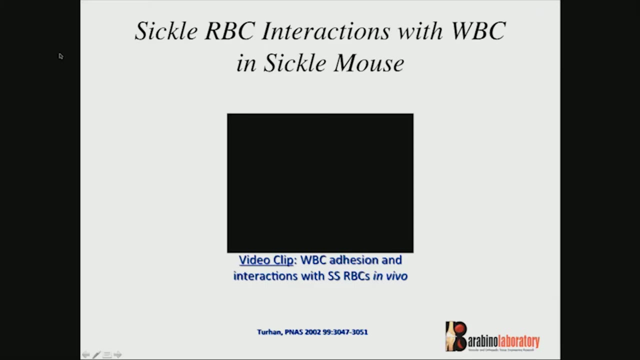 which was these two MD compounds actually blocked adhesion. So why is that important? If you understand these molecular mechanisms of adhesion and you find ways to block them, that can form the basis of a drug therapy. So we've done what I've been showing you. 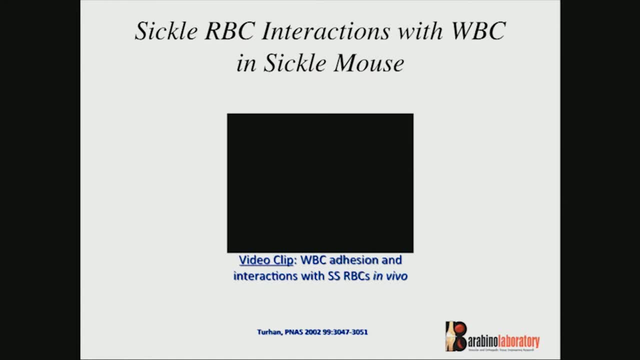 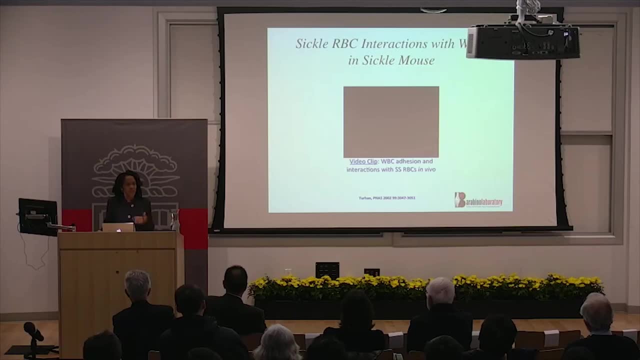 is in vitro studies, where we're using human endothelial cells and we're also using human patient samples, But we also learned what's going on from a fluid mechanical point of view by using mouse models. This study was done outside of my lab, but in this particular case, 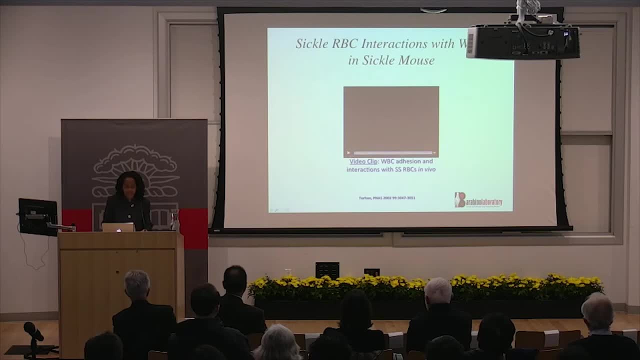 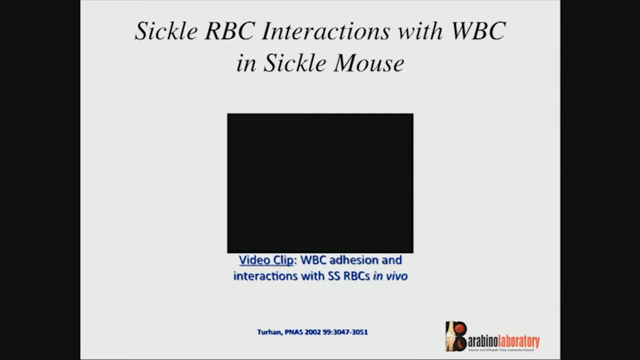 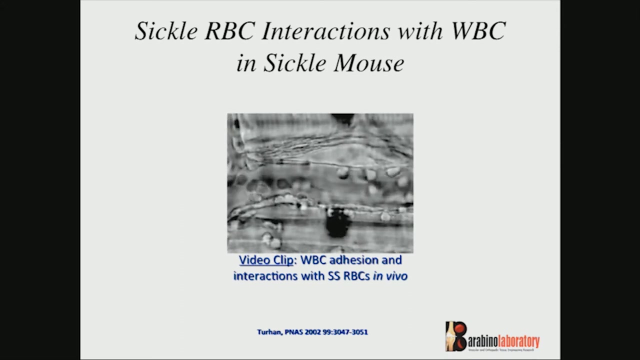 they were using a mouse model to mimic adhesion And this intravital microscopy- the first one that you're going to see- is an inflamed vessel, but the SA was. it's a wild type, so it's basically a control. so it's not sickle cell disease. 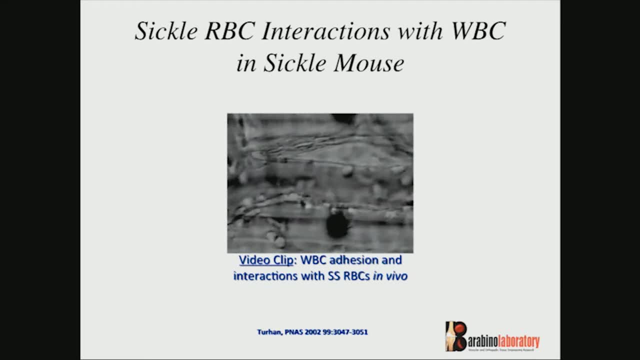 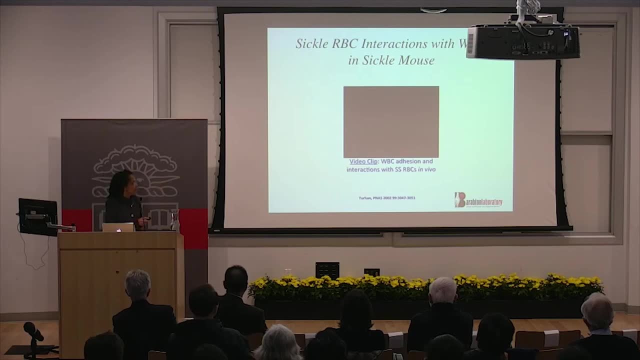 But here's what they were showing: that white blood cells could adhere to inflamed vessels. And so now we're looking at a sickle mouse with inflamed vessels, and the inflamed vessels already had these white cells adhere, and now they're perfusing sickle red blood cells. 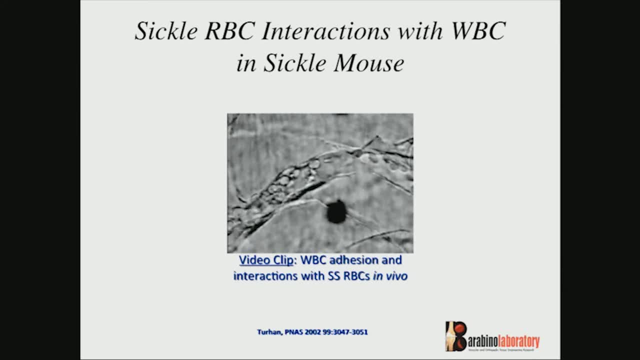 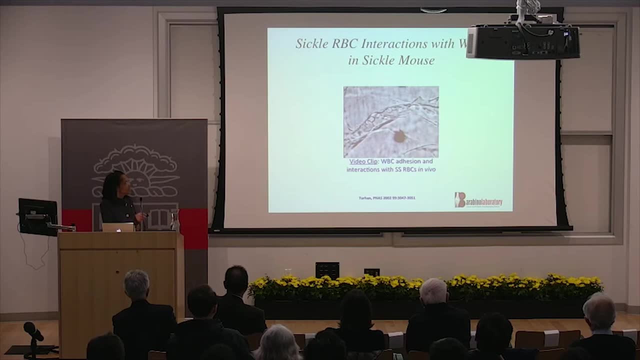 and we're trying to get a better understanding of how sickle red blood cells interact with white blood cells that are now interacting with the vessel wall, And what we're finding here is that the sickle cells can then actually adhere to the white cells that are adhering to the vessel wall. 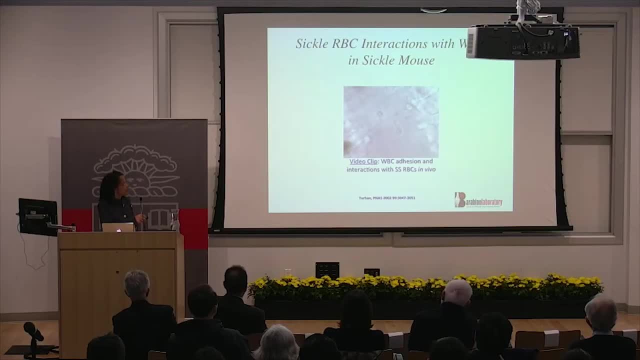 So not only can red cells adhere directly to the vessel wall. if there are white cells present, the sickle cell can adhere to an adherent white cell. And again, we're using fluid mechanics to better understand the process of vessel occlusion and what cell types are participating. 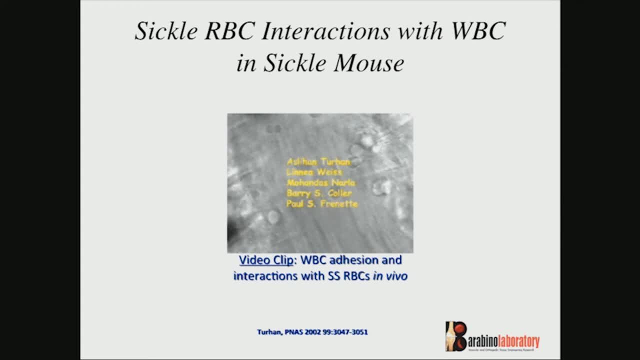 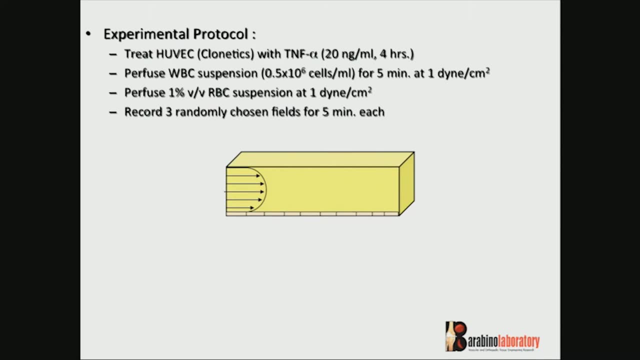 What's good about the in vitro system that I mentioned to you? now we can dissect out. so what you just saw in the intact intravital microscopy system was these cells participating, But which white cells are participating and at what level. So now in our in vitro system. 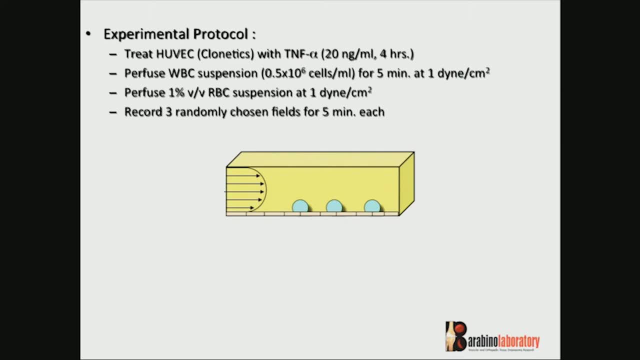 with the parallel plate flow chamber that I showed you. we're going to replicate what we just saw in the animal model and we're going to dissect it out to see what's happening. So we are also perfusing white cells and then the red cells and we're examining this in the video microscopy system. 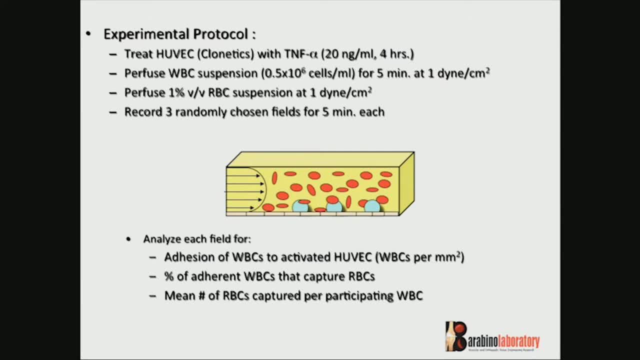 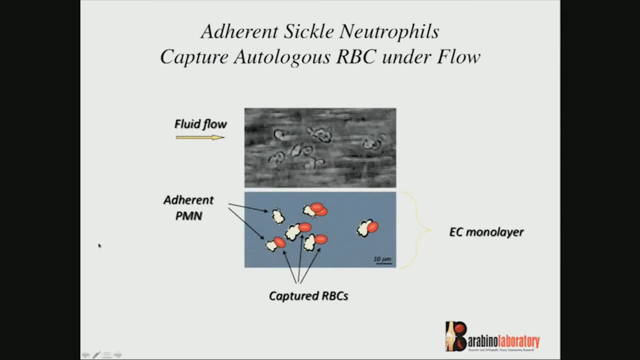 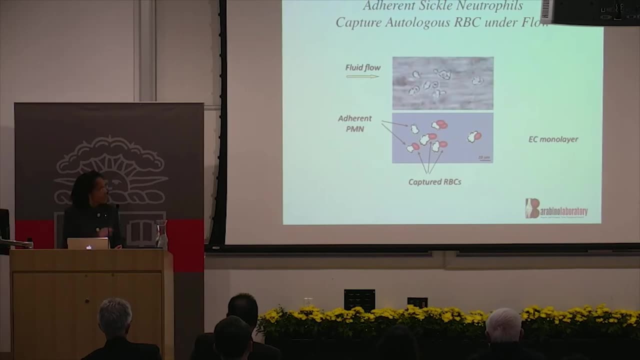 and we're looking at different fields and we're going to look to see which white cells might be playing a bigger role. So this is just the in vitro system that you can see. we're mimicking the flow and we here as well, can see white cells that were adhering. 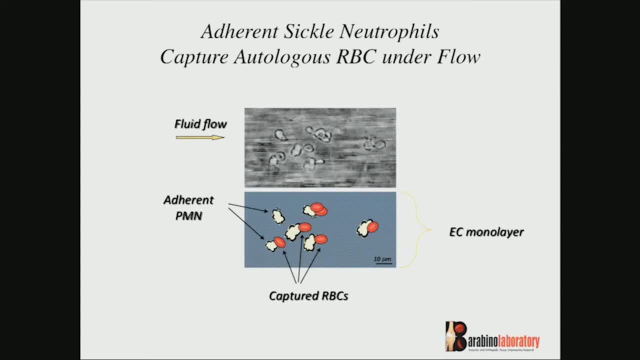 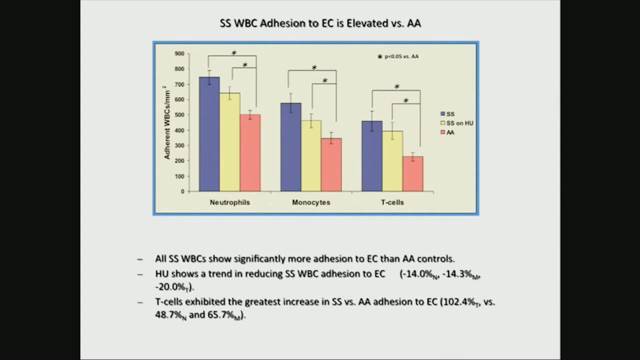 and then red cells adhering to the white cells. Because we could dissect out and look at different suspensions. we were able to show which white cell type was playing a bigger role and it turned out the neutrophils were playing a bigger role in just white cells adhering to the endothelial cells. 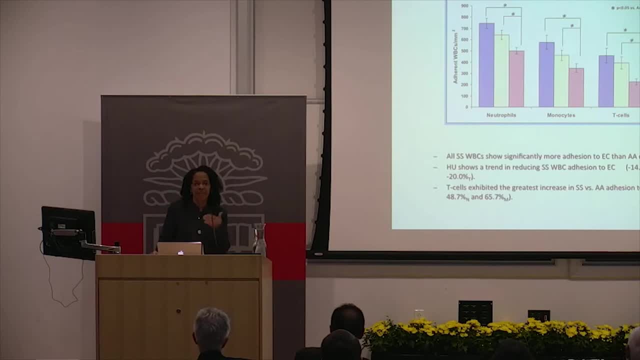 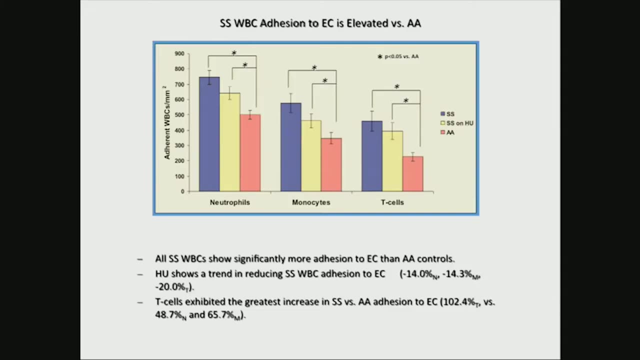 And importantly, I showed you earlier what happens with adhesion when patients were on hydroxyurea. So here we also looked at patients who were on hydroxyurea and we found that they had not as much adhesion as not on hydroxyurea. 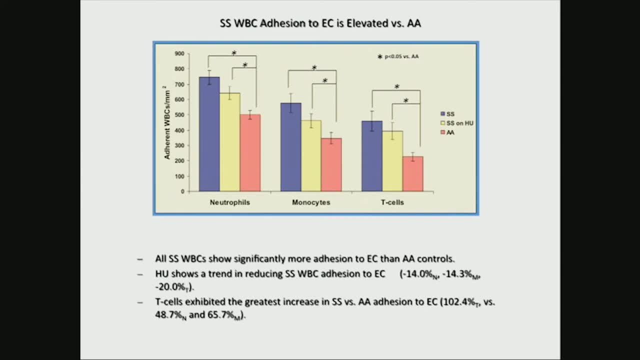 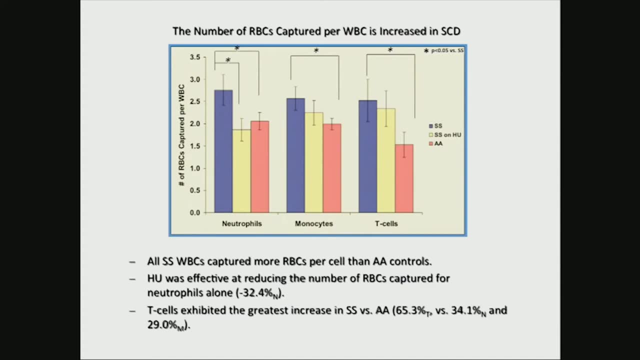 but more so than if it was a normal situation. So again we're getting clues, and in this case we're actually looking at the ability of those white cells to capture red cells, similar to what we saw in the in vivo case, and here we saw that these neutrophils 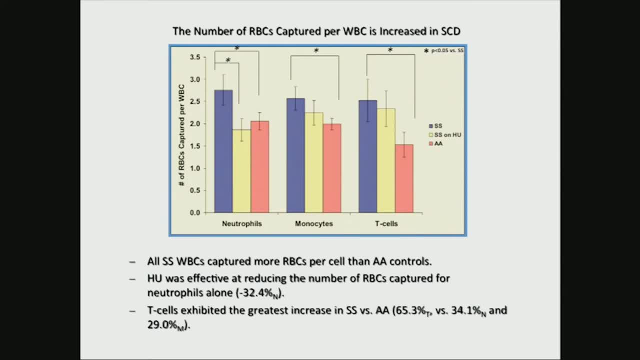 played an important role in capturing the sickle cells. and again, the patients who are on hydroxyurea. hydroxyurea seems to serve as somewhat of a mediator that ameliorates that what you see for patients with sickle cell disease who are not receiving hydroxyurea treatment. 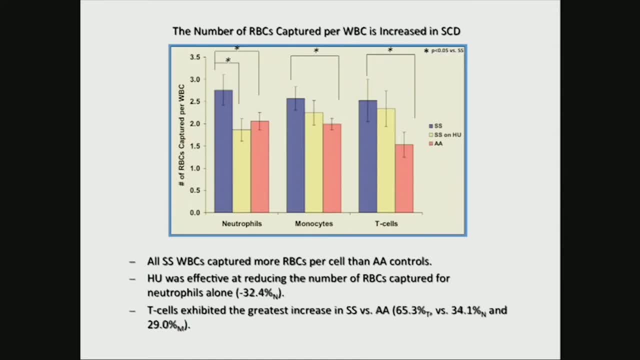 So that gave you a sense of how do we use the different mechanical property related to adhesion to better understand the process around vasoclusion, what happens in a therapeutic setting and what types of cells might be playing a role in that adhesion. Now I'm going to turn. 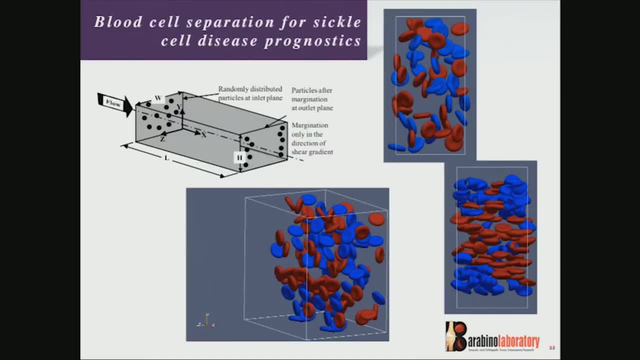 attention to other studies that we were doing to exploit the mechanical properties of the sickle red blood cells. In this case, our goal is: we're still working on this, but in this case our goal is to come up with a device where we can separate cells. 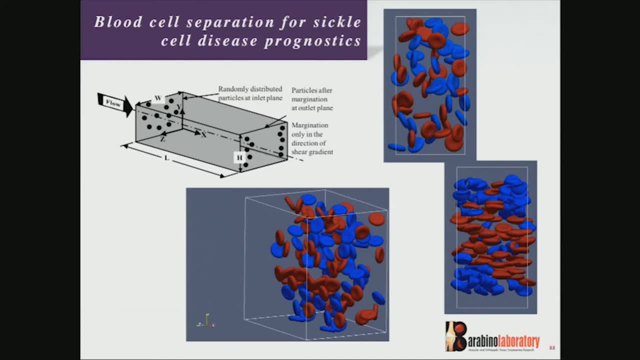 based on their mechanical properties. We know there are different types of subpopulations of red cells for sickle patients and we also know that if you understand the percentage of different types of cells, and maybe at a different point in time, it may give you a clue. 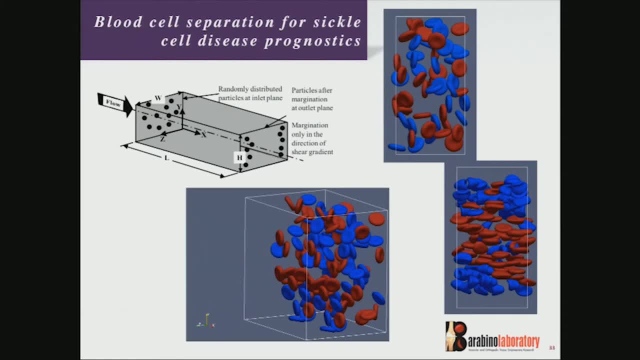 to how severe the disease is or the progression of the disease. So in this case we are using simulations of flow channels and cells of different stiffness in the flow channels. So the red cells are representing normal stiffness or normal red blood cells of that level of stiffness. 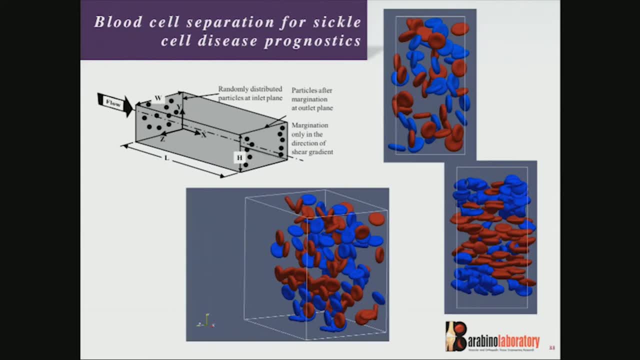 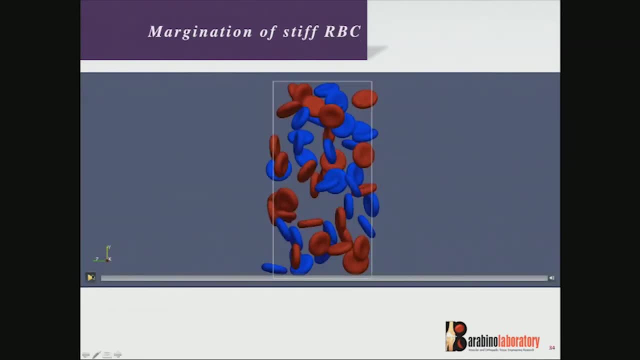 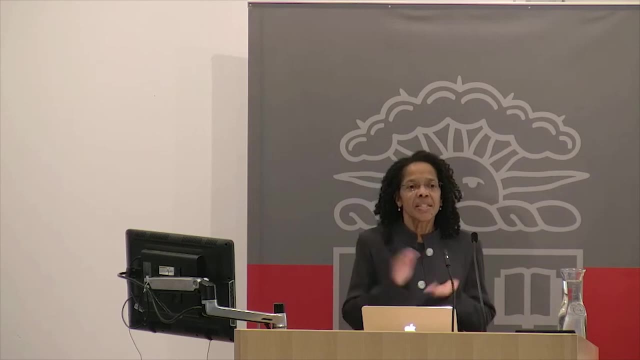 and the blue ones are actually representing cells that are more stiff and they would represent the sickle cells. So one of the things that we can see in this animation, from this simulation, is that the cells that are stiffer in channels are going to marginate. 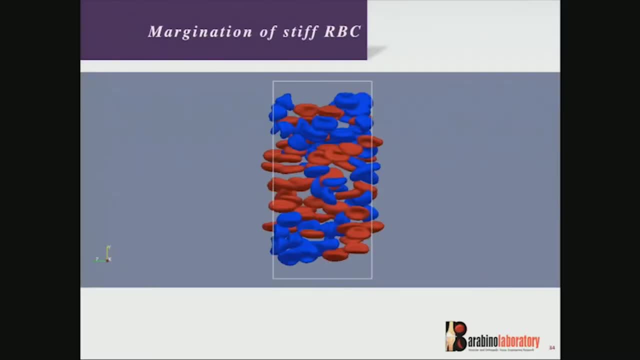 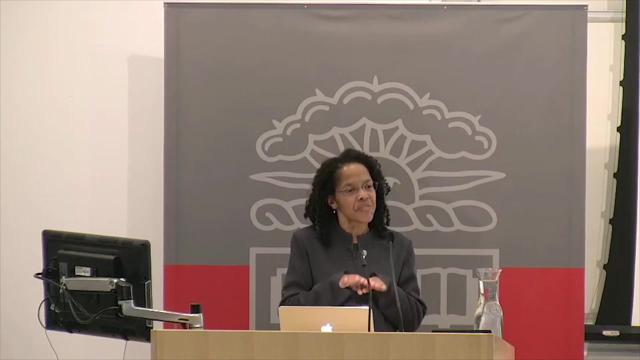 and go to the surfaces, so they are going to push out. So, if we are trying to devise a device that will allow us to separate cells based on their stiffness, better understanding this through simulations in terms of what are the properties and how do stiff cells behave under flow, 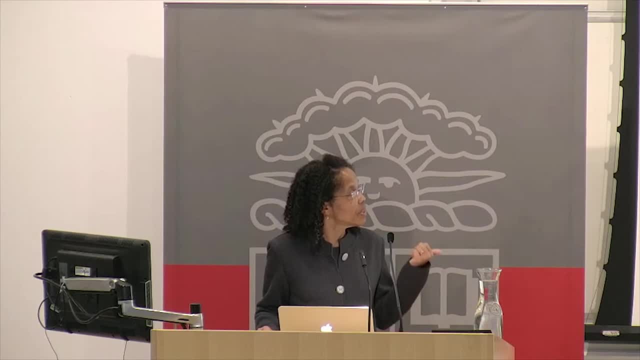 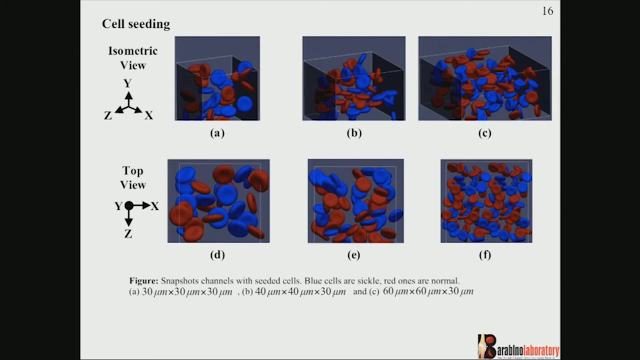 this is one way of doing it and that's what this simulation is actually showing us. What is the behavior? Now that we understand that, through a simulation, we can then, through the simulation, put in different populations of cells, with different percentages of the stiff cells and the cells that are not as stiff. 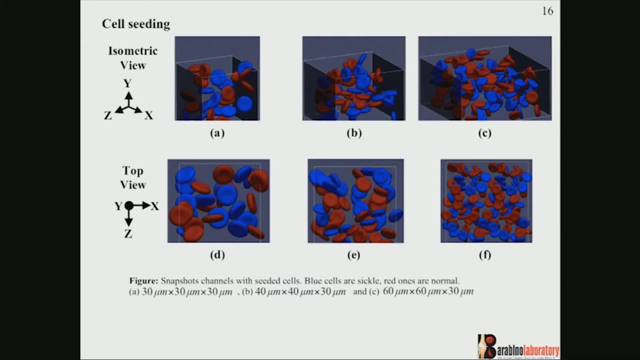 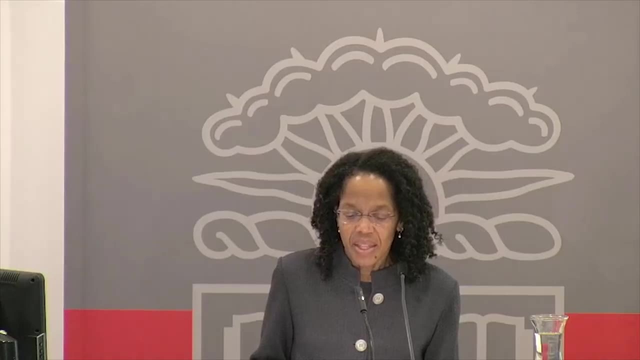 and we can use. we can change the geometry of the channels, We can change different parameters in the simulation that would approximate the kinds of shear stresses that you might see in the body, And this one just gives you a sense of simulating how cells are moving. 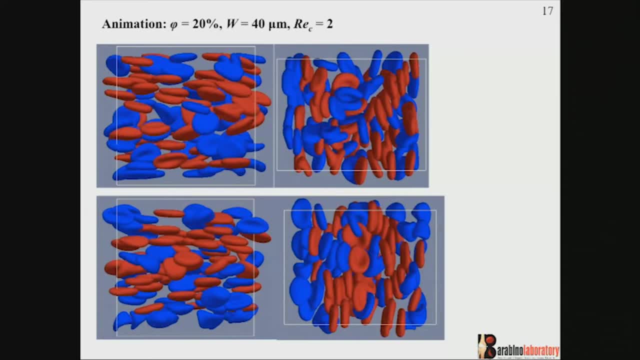 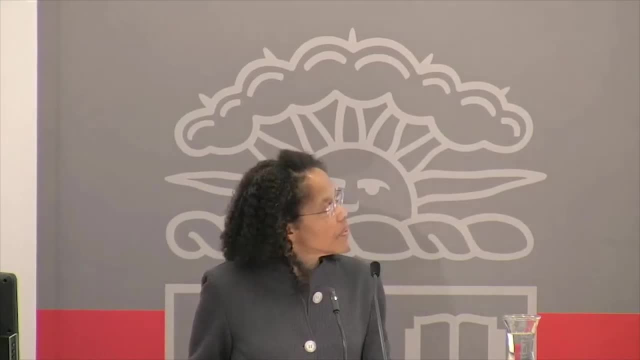 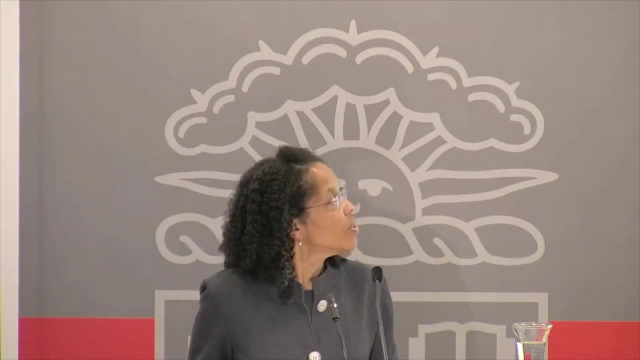 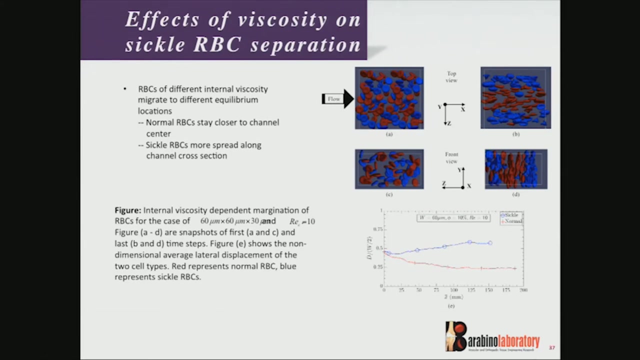 different groupings of cells, different levels of stiffness and different configurations. And the next few slides that I'm going to show you are static images, but what they show is that if you, through your simulation, if you change the internal viscosity of the cells, you can see differences in how 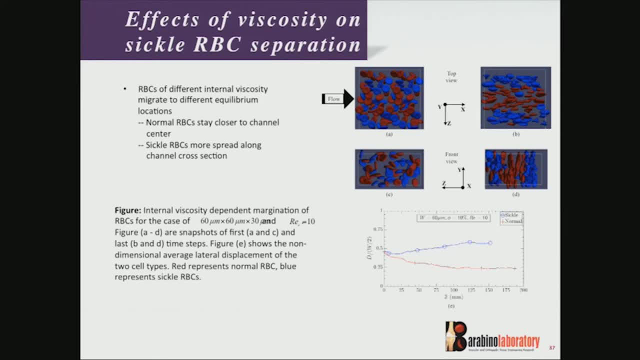 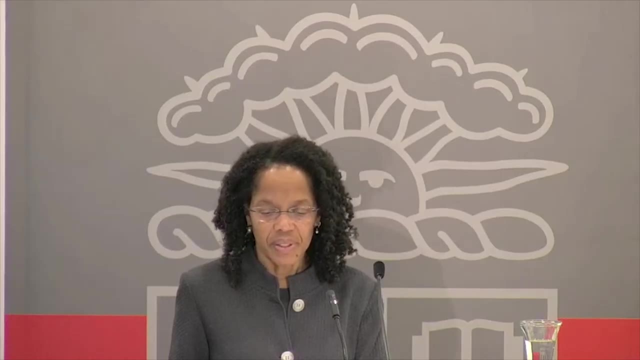 they move within the channel. We see that, regardless of the viscosity that the red cells will, the ones that are less stiff will stay closer in the channel center and the ones that are more stiff will spread to the surface. We look at the different cell types. 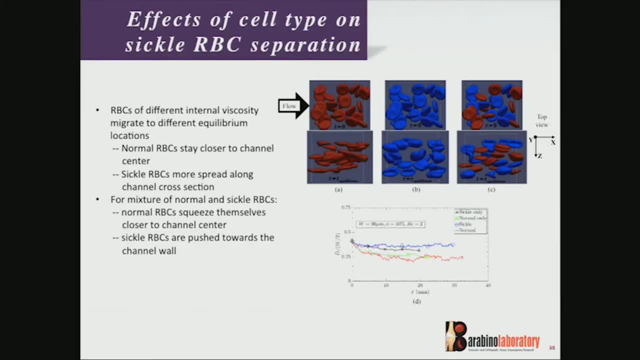 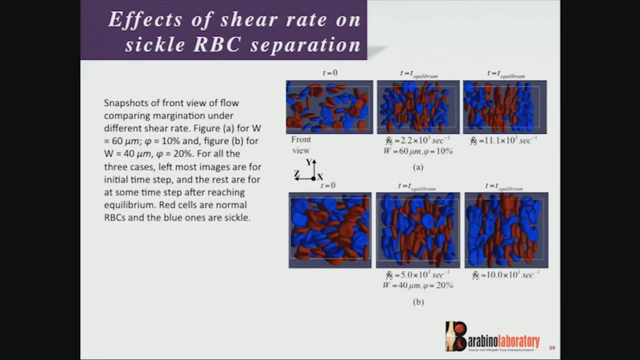 and again. we can see the different patterns if you have different mixtures, And we also look at things if you change parameters, like changing the rate of shear, and you will see differences as well. And what we found is that if you were trying to maximize- 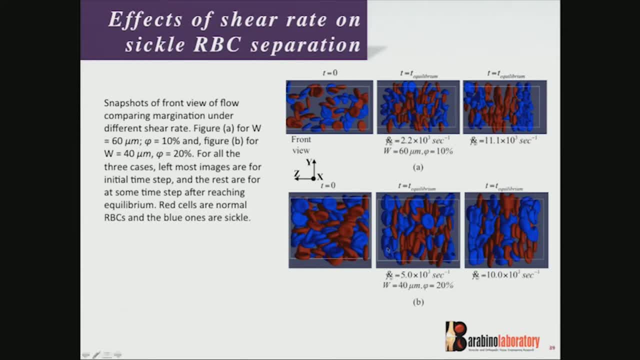 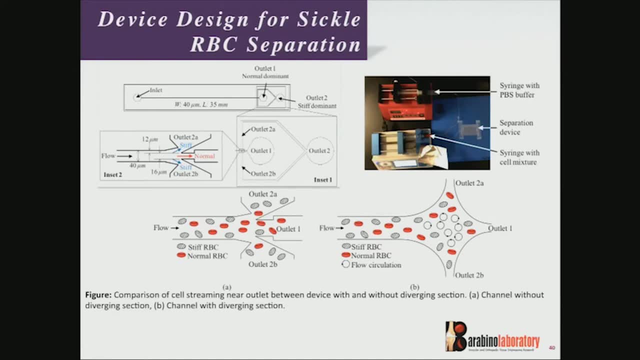 your ability to separate cells based on the level of stiffness that you would use higher shears. So that's good to have simulations, but you also want to have some experiments to back up or confirm the simulations and you want to absolutely eventually come up with an actual device. 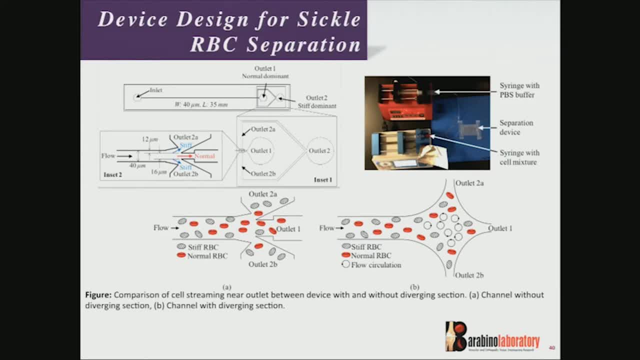 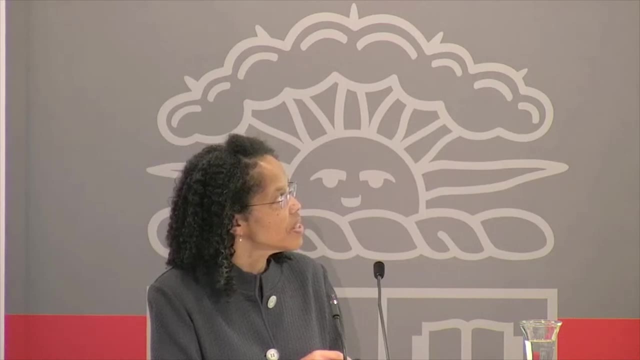 So this is early stage device where, based on the simulations that I just showed you and the properties that we found and the parameters, these are ways of having particular outlet systems where you can in fact separate the cells based on the level of stiffness, And there's been some experiments. 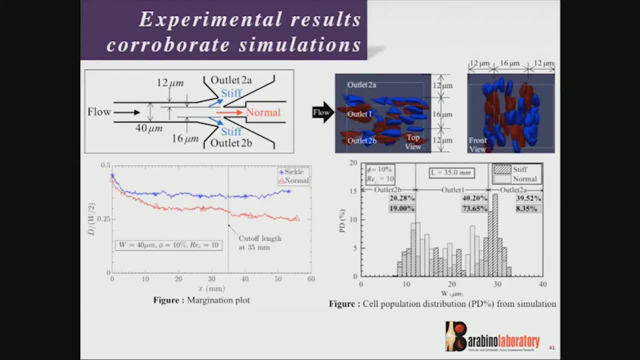 to demonstrate that, And so far the experimental results have been corroborating the kinds of things that we've seen through the simulations. So the next step here would be to further refine this device. Once the device is working, we would actually take blood samples from a patient with sickle cell disease. 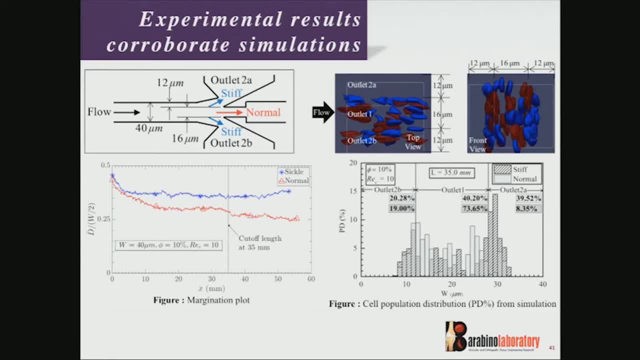 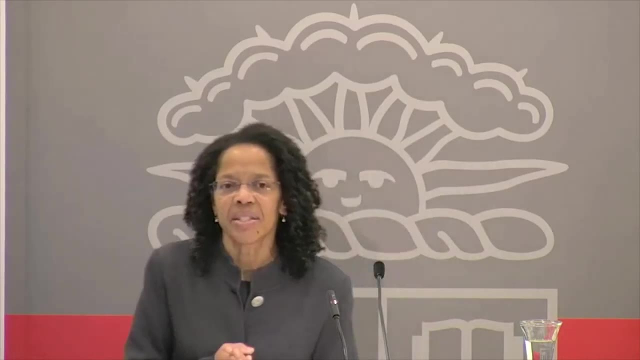 run it through the device, do the separation and collect the cells of the different levels of stiffnesses and look for clues how you can correlate that around disease progression. And the last area that I'd like to talk to you about is some other studies that we've been doing in the laboratory. 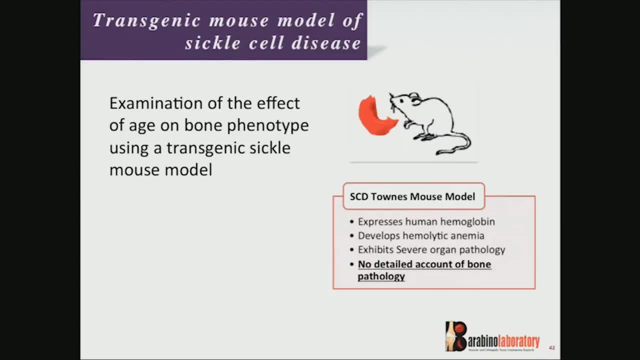 more recently, and these are specifically looking at bone for patients with sickle cell disease. Bone is one of the most understudied tissues for sickle cell disease and we know, if you can imagine, you've got a problem, as I mentioned earlier, with the red blood cell. 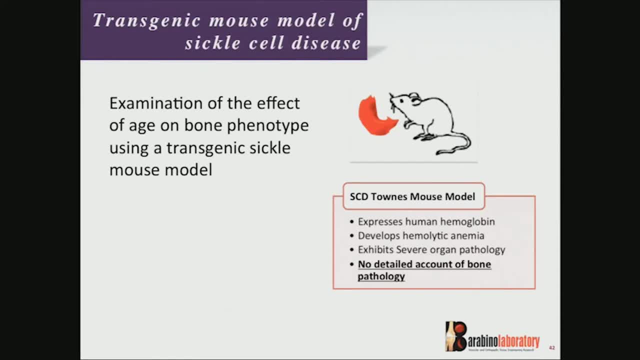 the red blood cell is in the vasculature, so it's going to affect every organ and every tissue. Not only that, the blood cells are emerging from the bone marrow, and so there's no way that you would expect that there's not going to be problems. 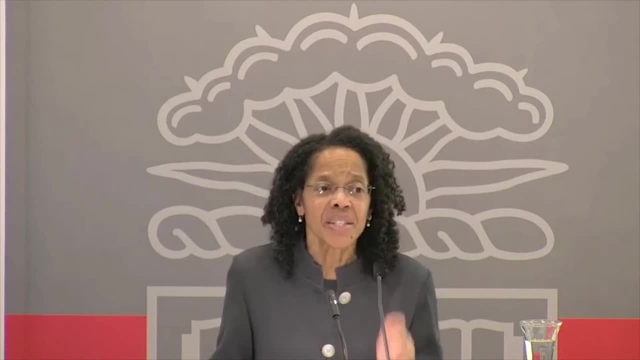 with the bone. What we want to do- because it hasn't been done in an extensive way- was actually look at mechanics as it relates to bone. For these experiments and these studies, we used a sickle transgenic mouse, so the mouse is transgenically manipulated. 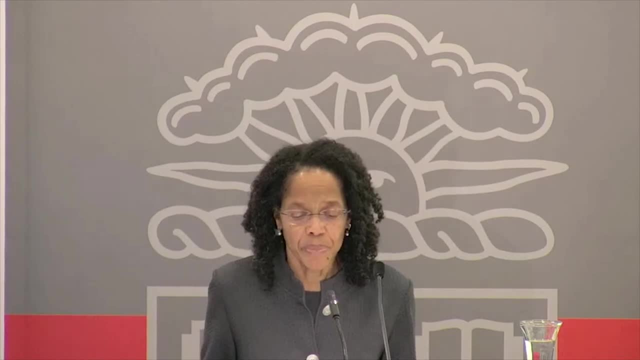 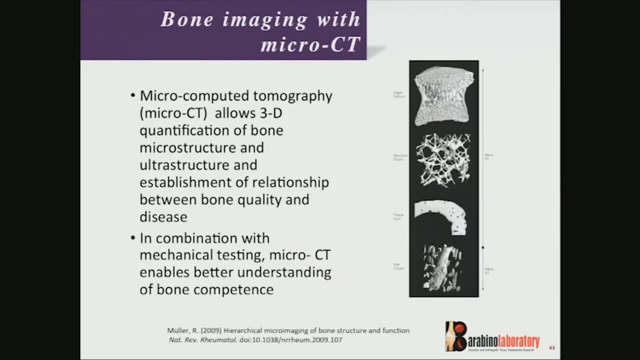 to express sickle hemoglobin and through this we're going to look at the bone phenotype for sickle. We're using micro CT so to look at imaging and the micro CT allows us to look at the structure of the bone in a way that we would not be able to. 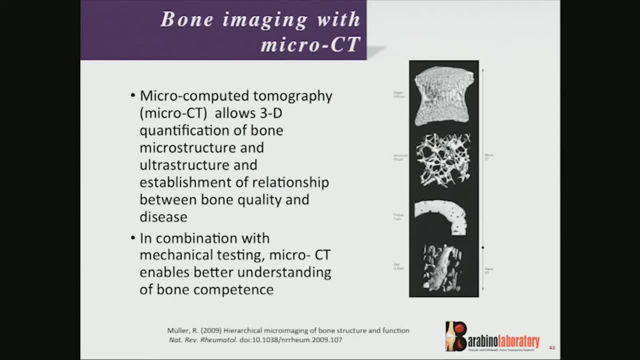 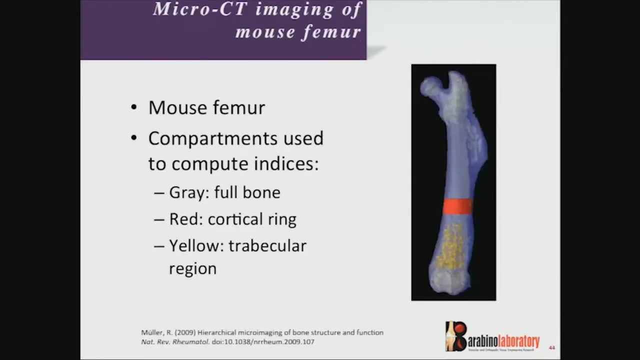 if we did not have the imaging of these kinds of images, and we're combining this micro CT with mechanical testing. The bone type that we're looking at is the mouse femur, and it turns out that the mouse femur, in many studies, has been shown to be a decent model. 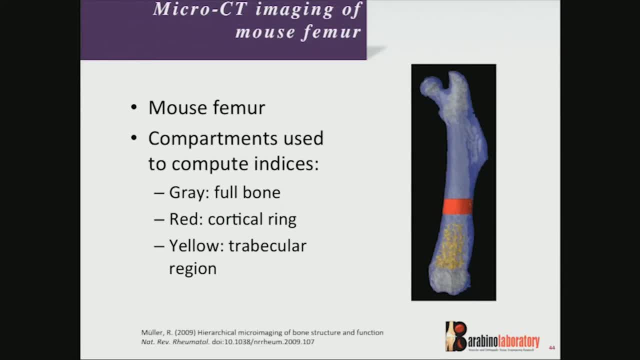 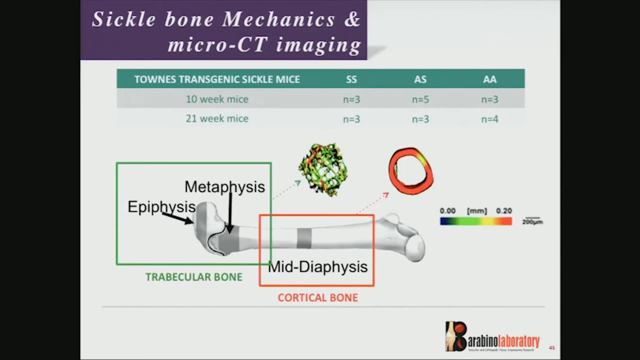 for human bone behavior and in this mouse femur we've been looking at the cortical ring and the trabecular bone, And here's some of the well, I'll show you next some of the results, but to give you a sense of what we were doing, 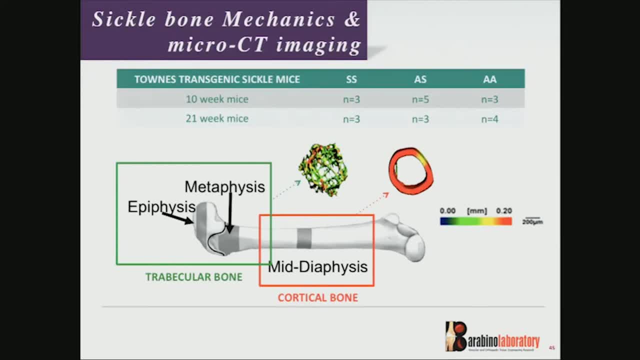 we were looking at 10 week old and 21 week old mice and the 21 week old mice are approximating at least adolescents and adults with sickle cell disease. And the reason why it's important to look at the mice in older mice and try to approximate. 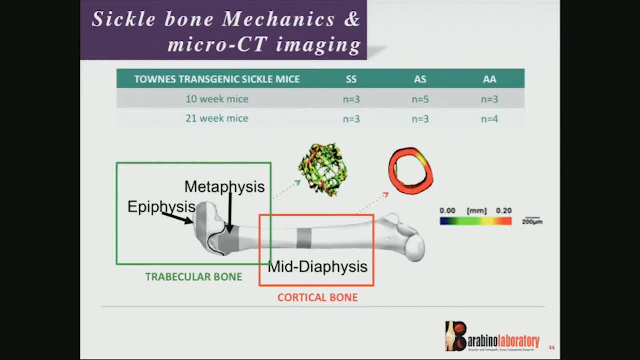 what happens with aging. there's so much in organ damage for those with the disease. the older you get, the more in organ damage there's going to be, And so we're looking at these areas of the bone. this is from the micro CT and we use this cortical region. 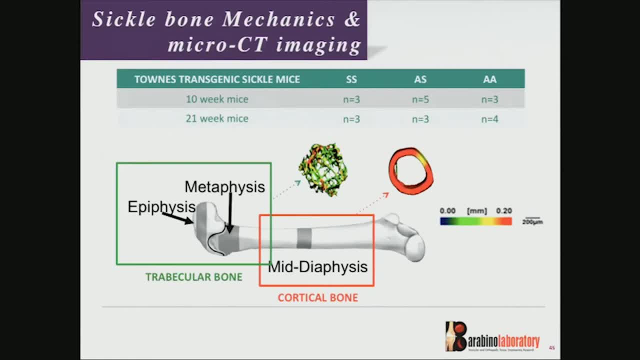 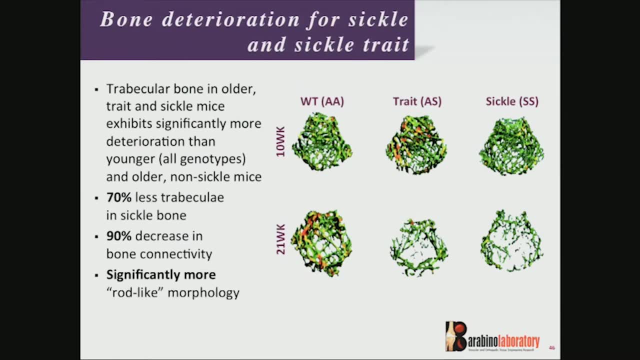 for mechanical testing. and again 10 weeks and 21 weeks And here's some of the findings. So, normal or wild type mice, these are mice that are trait mice, so they have some sickle and some normal hemoglobin and these are the sickle mice. 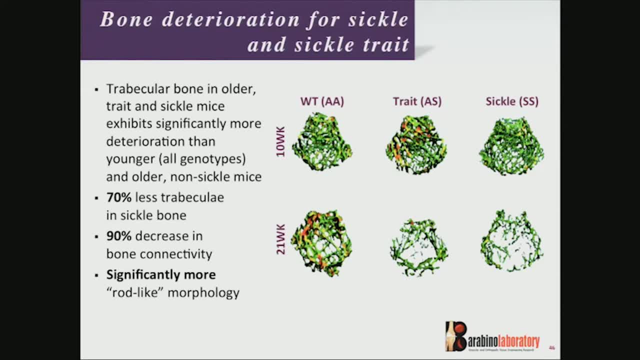 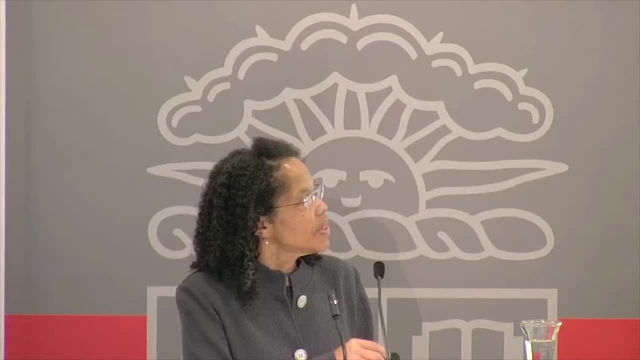 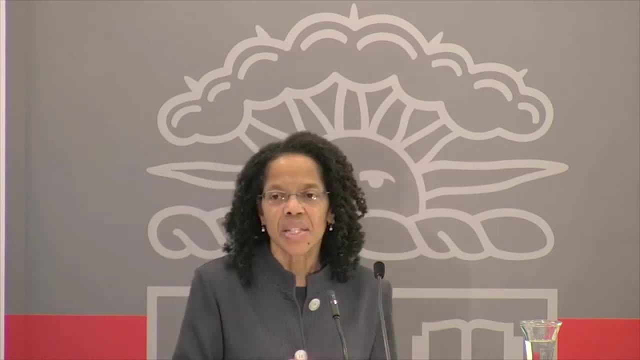 This is 10 weeks. Look at the difference in the structure at 21 weeks. So you're going to get some deterioration with respect to aging. normally We were surprised actually to see this much change for trait, because trait is carriers and they're asymptomatic basically. 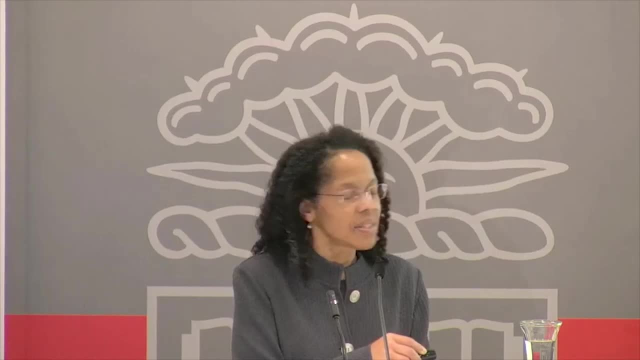 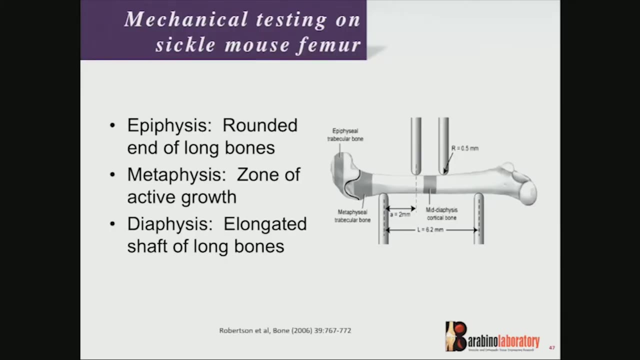 But this is actually. this is a dramatic change for sickle and sickle with age. We did what we call a four point testing to look at mechanical strength and other mechanical properties. based on this mechanical testing, using this part of the long bone, and I'm going to show you. 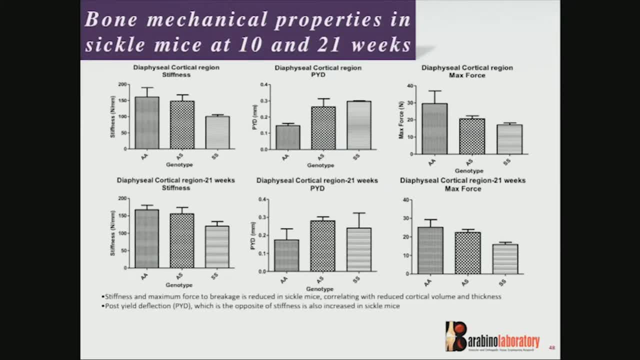 some results from that next Top- this is 10 weeks and the bottom is 21 weeks- And some of the things that we saw when we looked at stiffness and we looked at the yield and we also looked at the maximum force it took to break the bone. 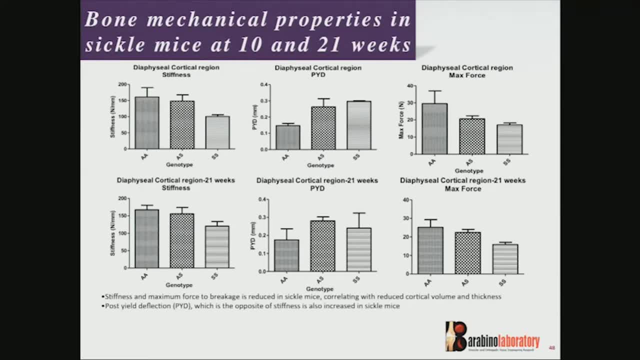 What I'd like to draw your attention to: that sickle has this decreased stiffness and sickle broke with less force, But surprisingly it had this higher post deflection yield And we saw the same kind of trend with age. So one of the things 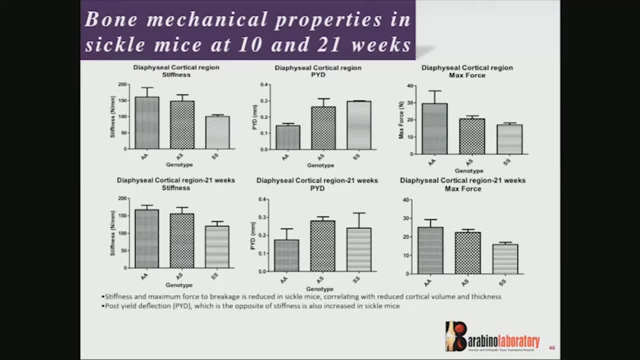 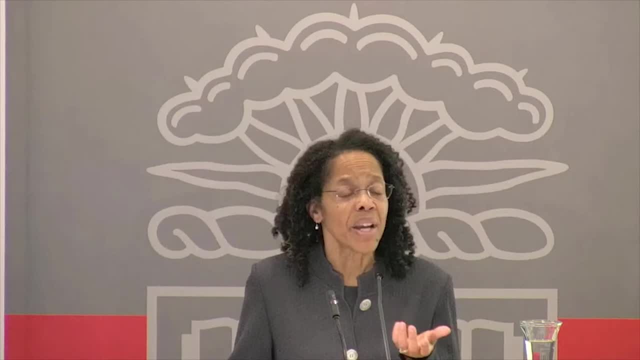 that we think about. why is it that we know the sickle bone is going to be more fragile and why is it that in sickle cell patients we actually don't see as many fractures as you might see with someone with osteoporosis, for example? 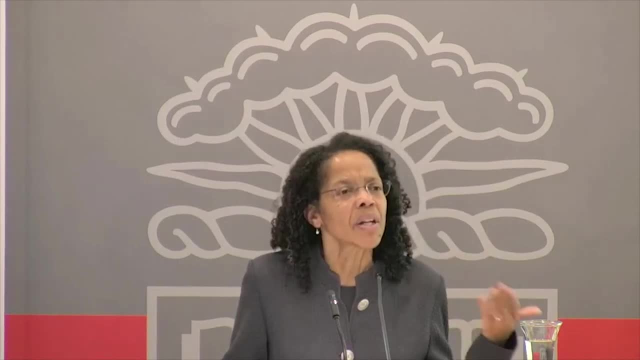 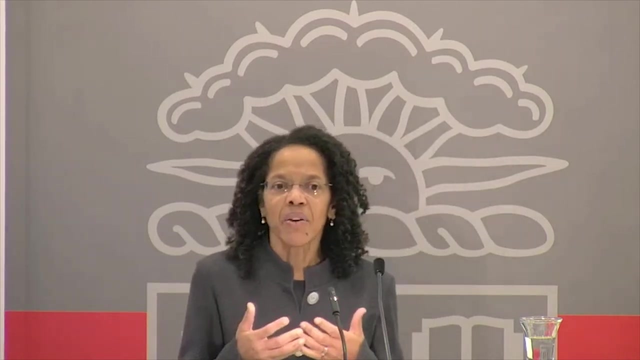 Yet the bone, especially from a micro architectural level, looks osteoporotic. But why are there not as many fractures reported anyway? So we thought that maybe this yield gives us some idea of what might be going on, and this would be another example of understanding a mechanical property. 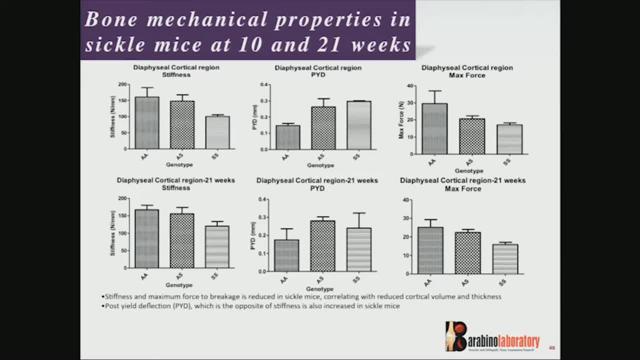 in a way that can help you understand disease. So it could be that the bone that is there is a bit more pliable, And so that maybe serves as a compensatory mechanism so that that bone is, even though it seems more fragile, it's not as prone to breakage. 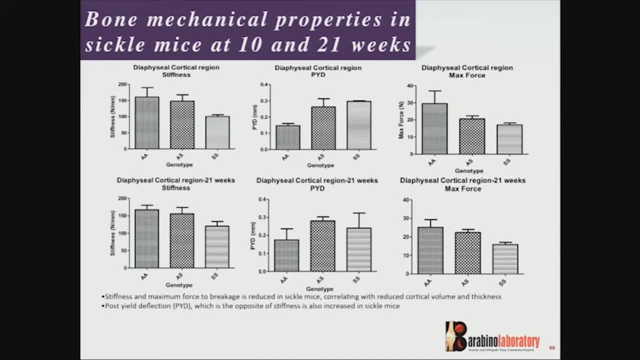 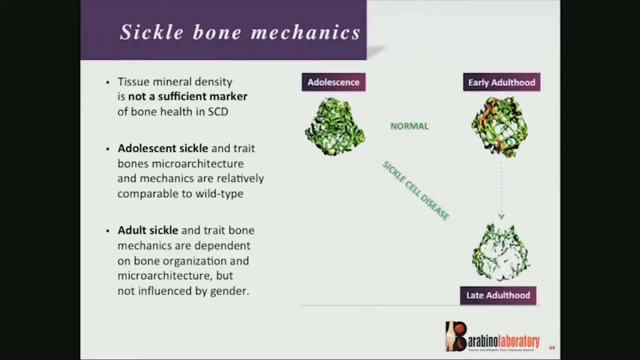 as it would be if it didn't have that level of yield. We don't know that for sure, but that's something that we could look at in the future. This just sort of sums up what we just talked about, that if you have this level, 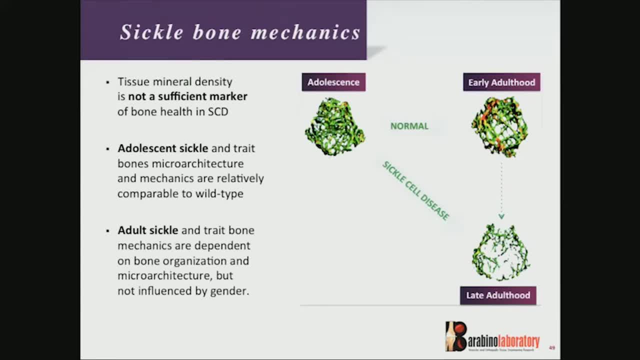 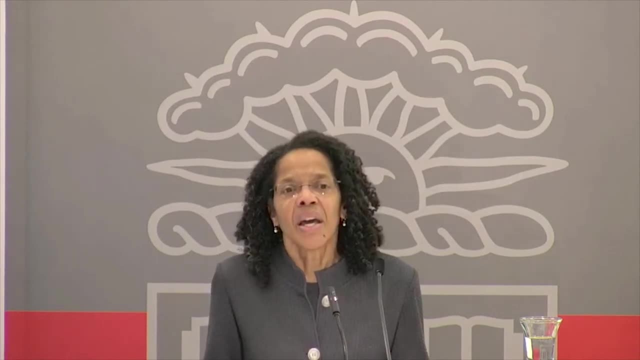 of what the bone structure might be. this is what it might look like normally as you get to our early adulthood, but this is what you look like when you have the complications of a disease like sickle cell disease and how it impacts the bone. We are looking for as many clues. 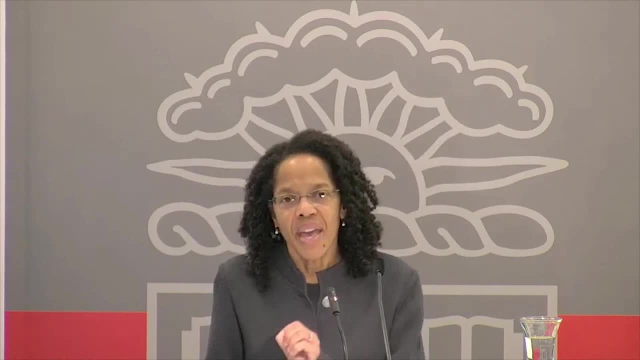 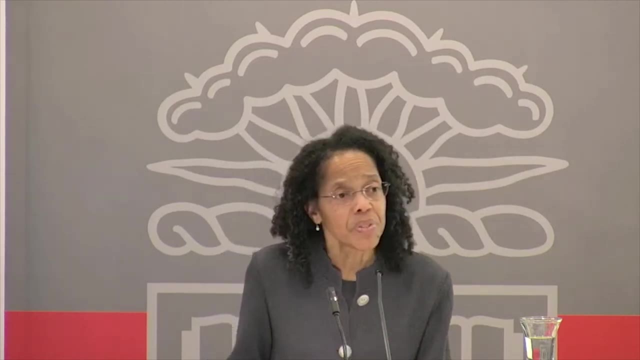 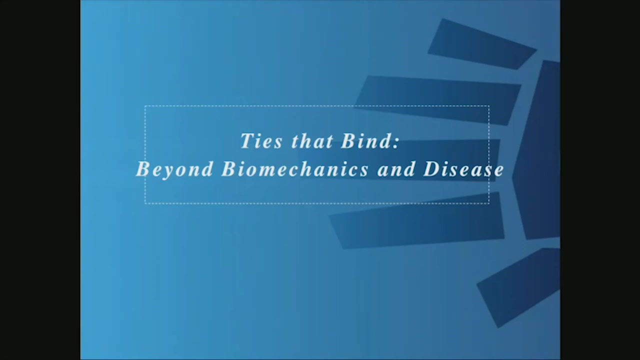 as we can get from these mechanical studies, so that they can help inform those on the clinical side who are actually charged with coming up with treatment strategies for the patients. So the last thing I want to leave you with is just a couple things to think about. 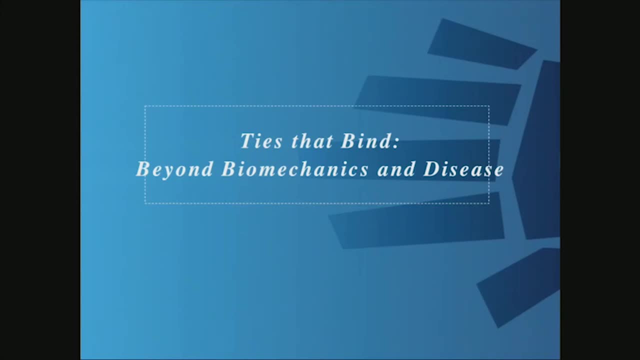 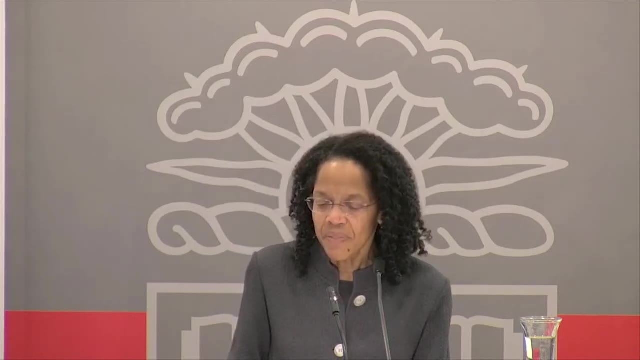 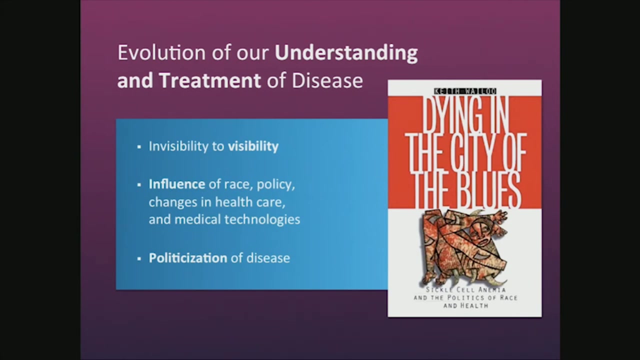 beyond the kinds of scientific studies that we're doing, to look at the connection, the interplay between mechanics and disease, And one of the things that I think is important to think about is the evolution of our understanding of treatment and disease. I draw your attention. 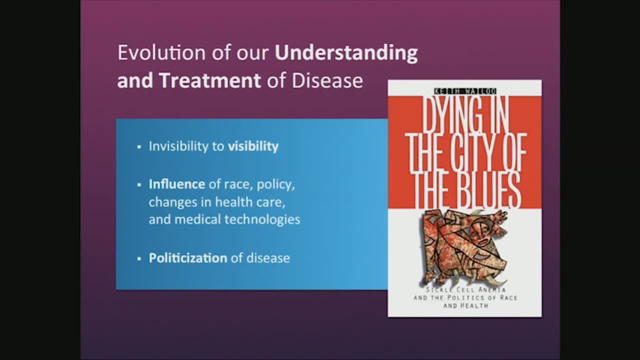 to a book that was written by Keith Wailoo, and the title of the book is Dying in the City of the Blues. He actually he's a social scientist, and he used sickle cell disease as a lens by which to study the intersection between race. 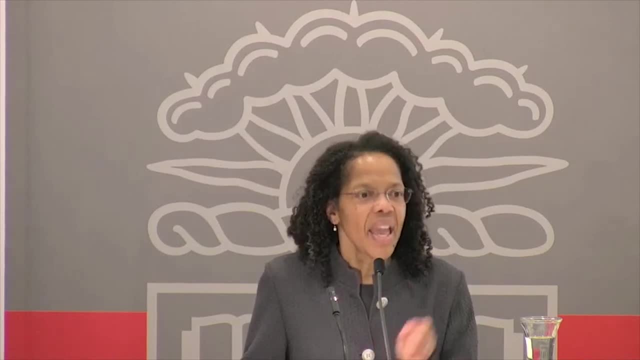 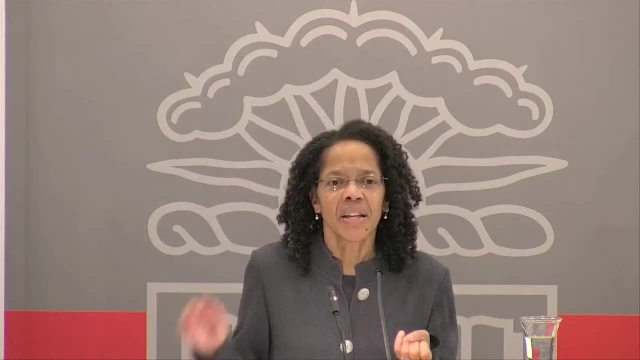 policy and disease And what he was showing in studying it. he did a study in Memphis. he looked at things like policies, regulations, and that's one of the reasons why I mentioned the Sickle Cell Act, of Sickle Cell Control Act in 1972.. 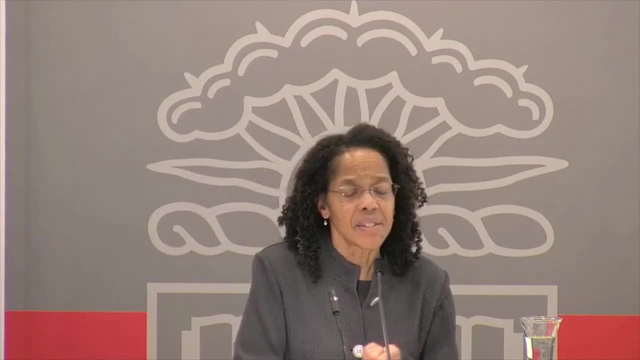 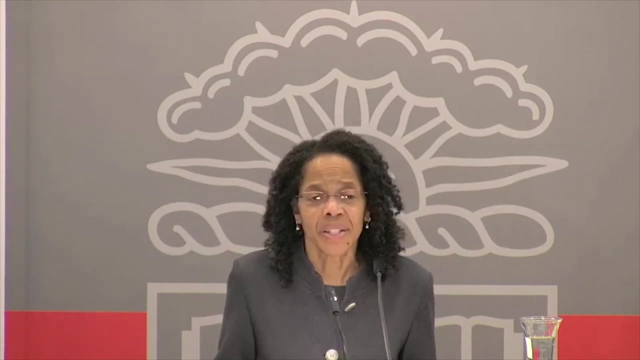 He looked at how people were being treated, access to treatment, to therapy, and how sickle patients might be treated in relation to others. Sickle cell disease is actually noted within the country as a public health concern and a health disparity, And I have been very much. 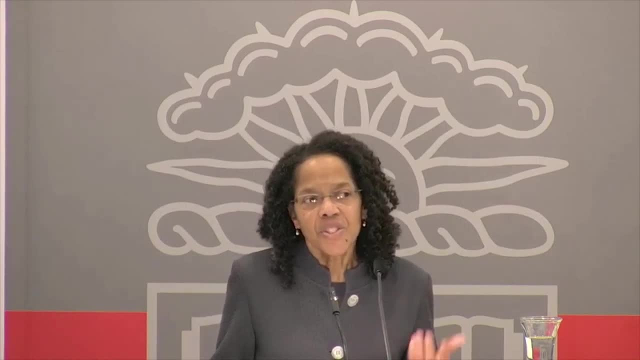 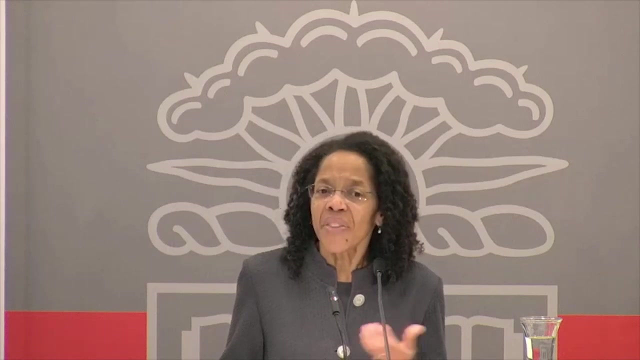 interested throughout my career in issues of equity, including issues of equity around health, and how the discoveries that we come up with as engineers and scientists- the new technologies, the new advances, the new techniques- how they are accessible to different populations. So I've been following. 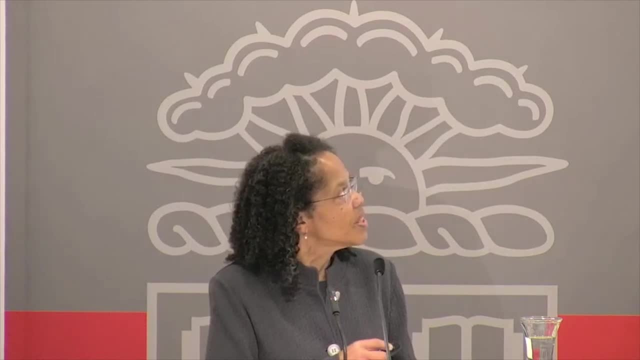 the work of Keith Wailoo. So one of the things that he talked about when he said invisibility to visibility, we have to pay attention to diseases and we have to have the kind of structure and support from the government and how we fund disease. 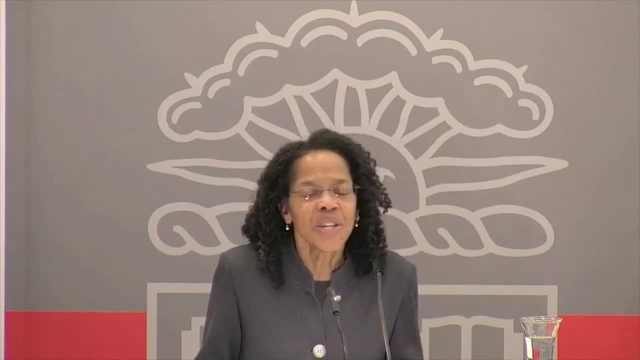 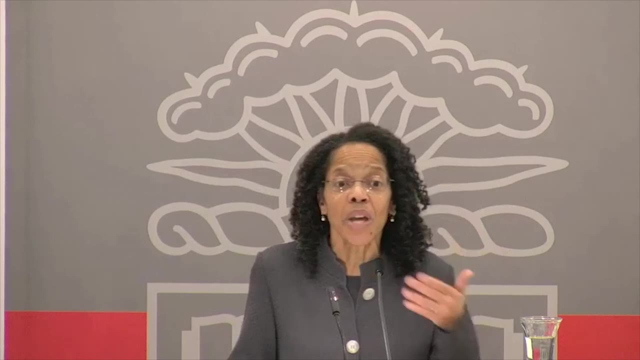 how we study them and how people have access, And I think you can imagine that. just think about what you hear on a regular basis. which diseases come to mind? which at the forefront, of course, cancer, but there are other diseases that may affect smaller populations. 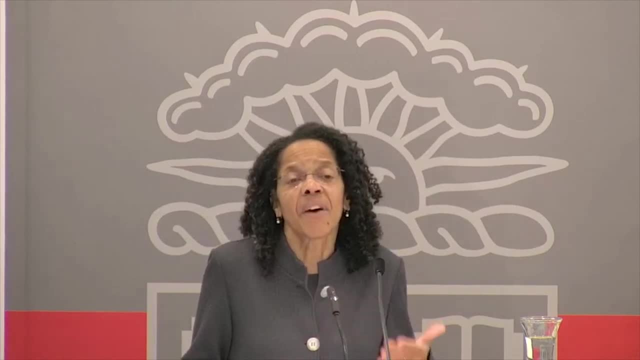 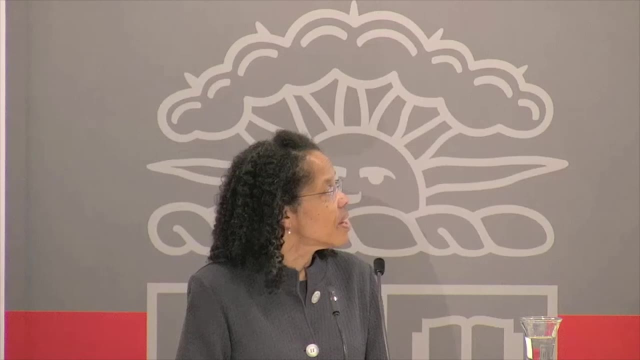 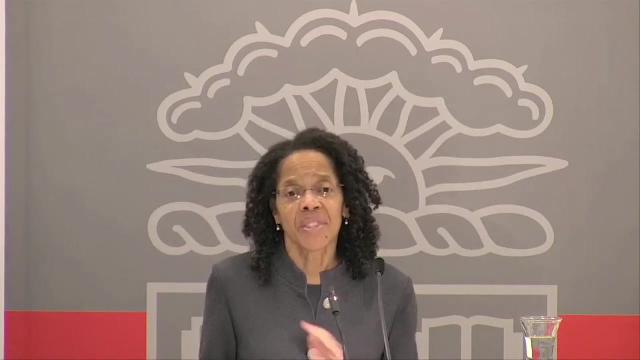 that get more attention just because of how it's positioned politically, for example, or who are the people who are predominantly affected by the disease. And he also talked about in many ways, how we politicize not just broad areas within society, but something as crucial. 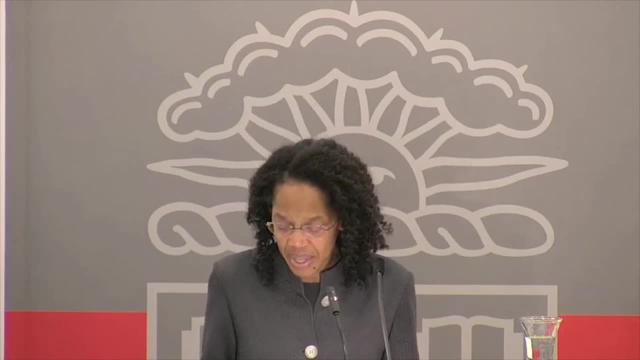 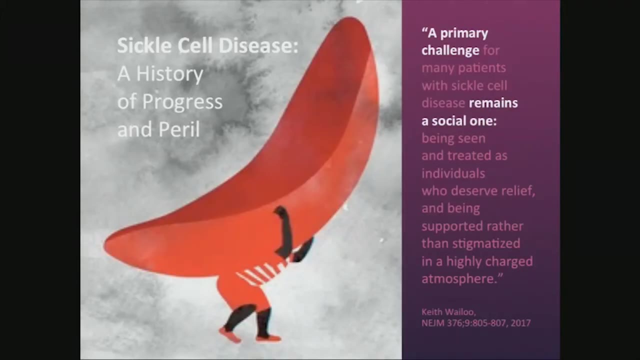 as health, which you think everyone would have the same kinds of access. He also talked about looking at sickle cell disease in terms of a history of its progress, but also peril, And the peril he was bringing in, the ideas of politics, for example. 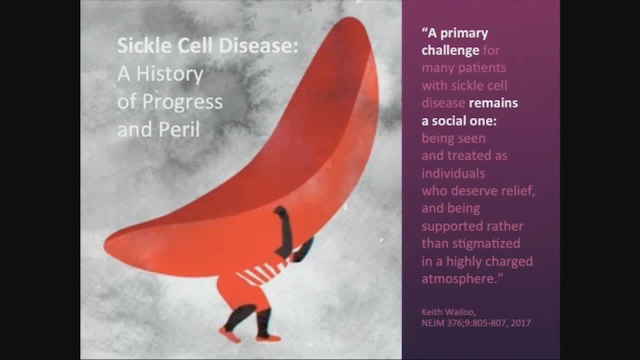 But sickle cell disease was first discovered 100 years ago And, with all of the advances that have come with understanding the genetic defect, what's causing it, what's causing the disease, we still are at a very rudimentary stage around treatment and strategies. 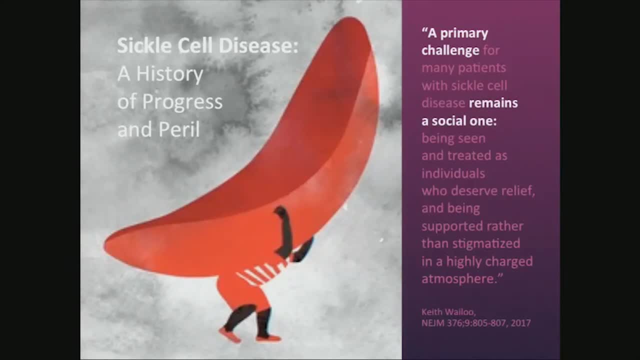 We're still at a very rudimentary stage of unlocking the mysteries of the biomechanics of cells and tissues that can tell us more about the disease. So there's much more to be done. I became very fascinated with the red blood cell in particular. 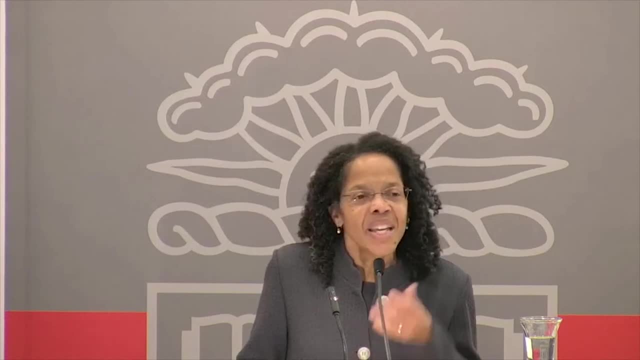 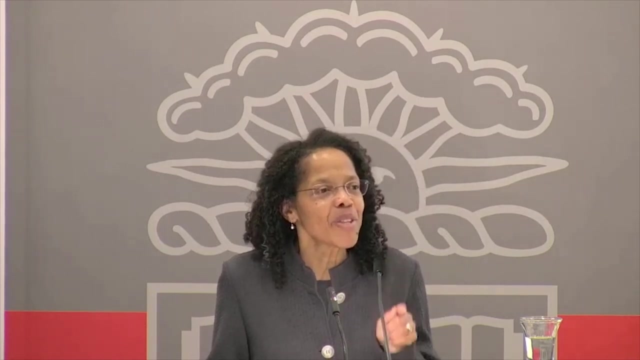 as a graduate student, because the red cell, as simple as it seems, it does so much And it has so many complications, even though it seems like it's a very simple cell. And, interestingly, the red blood cell is one of the. 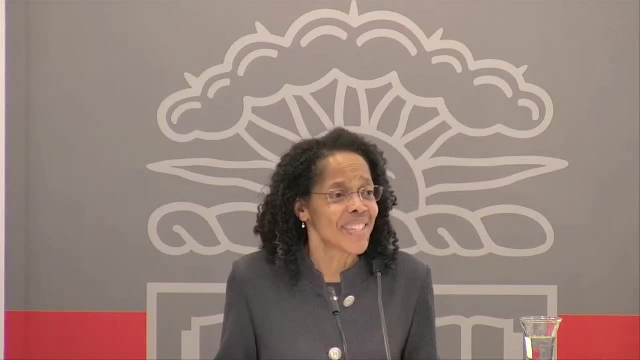 from a biomechanical point of view, is one of the most studied cells in the history of our studies of cellular biomechanics, And there's more work that's been done on the red blood cell, the mammalian red cell, than almost any other cell. 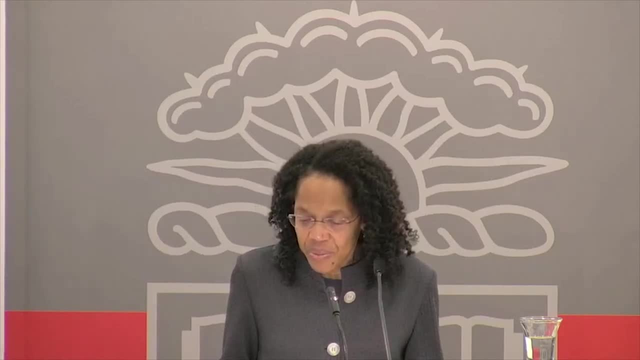 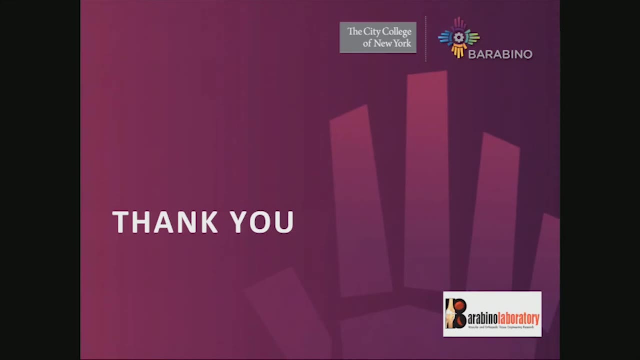 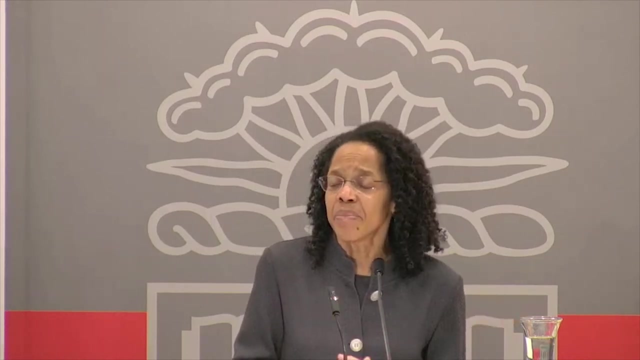 So with that I want to thank you very much for your attention. I hope you've seen a bit about my own journey towards looking at the interplay between biomechanics and disease, opened your eyes a bit to the mystery of it and what we can continue to do. 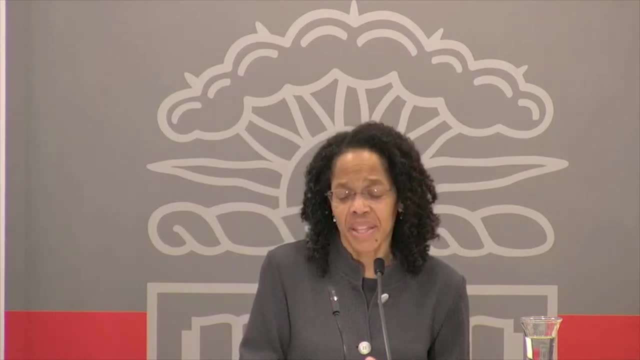 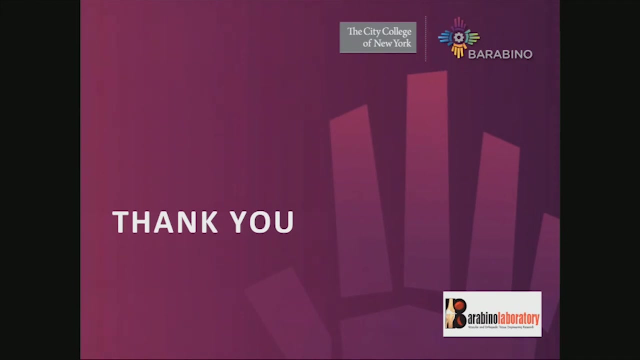 to unlock the mystery of disease using biomechanics and to look at a broader scope in our place in society in making a difference. So thank you very much. Thank you, Hey, Gilda, Great talk. So I had a question about your adhesion. 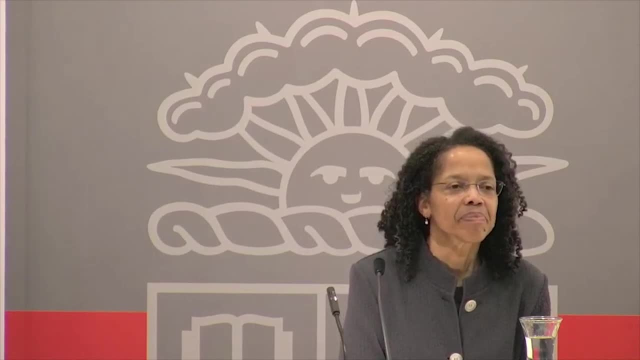 with white blood cells, And so you had mononuclear cells that were granulocytes, where you had higher levels of adhesion than monocytes, But in terms of their size they're very similar. So I was wondering if it was an adhesion molecule. 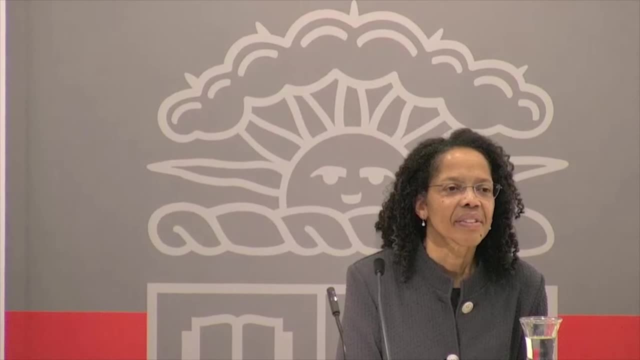 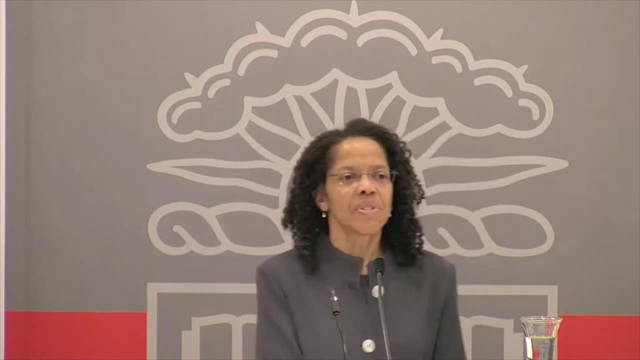 interaction or, if it was deformed, of adhesion of the neutrophils or maybe even stacking of the neutrophils that leads to higher levels of occlusion Right. So we know more about molecular mechanisms between the red cells and the endothelial cells. 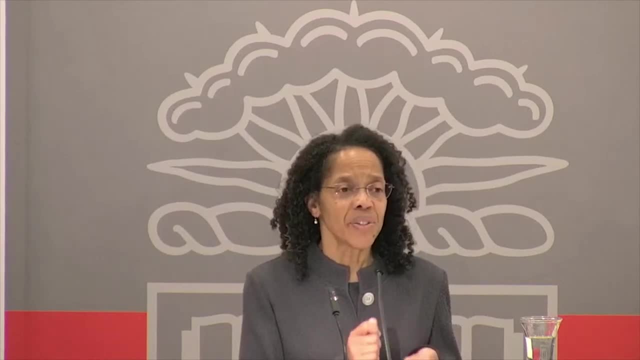 We're learning more about which molecules on either side of the white cell and the red cell are playing a role. So we do think there's a molecular interaction, But we're also learning that in addition to the molecular interaction, there are things that are just about. 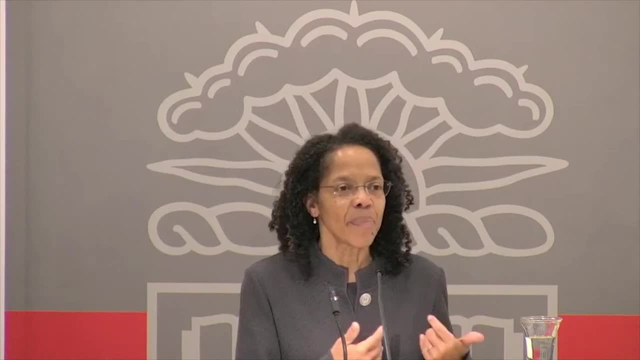 the physical mechanics, the trapping based on size. So I'm glad you bring up the idea of size because the white cells are so big. Did you try like GR1 antibody or something like that? We have not, But those are the kinds. 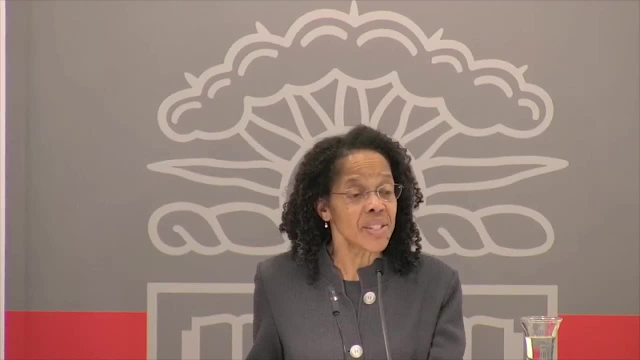 of steps that we need to do to be able to say definitively which one of these molecular interactions are playing a bigger role. Yes, would you like to ask a question, So you probably covered this, but can you tell me if the healthy red blood cells convert to sickle cells or they're produced as sickle cells. Okay, so if the patient has sickle cell disease, that means they have sickle hemoglobin in every cell that's coming out of their bone marrow has sickle hemoglobin in it. 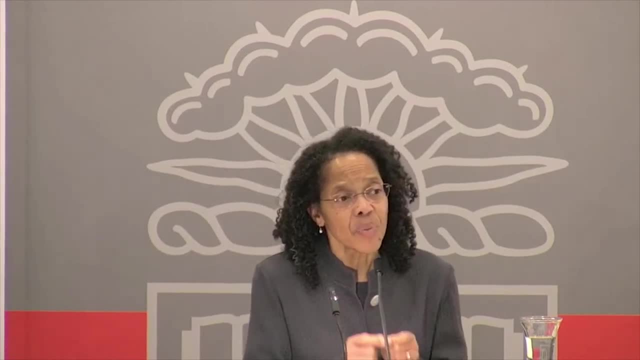 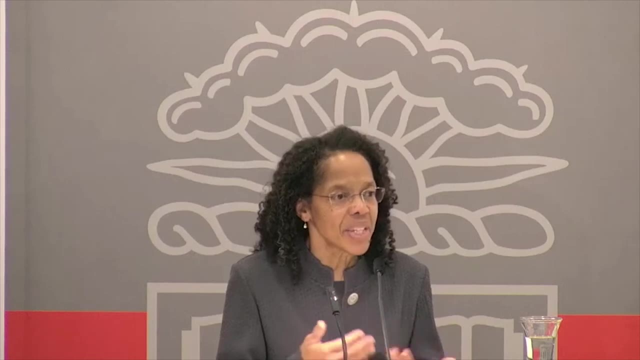 And what happens is every single cell with sickle hemoglobin is not always in a polymerized state. Okay, So at any given time in the circulation you'll have a combination of the cells that are actually in the sickle state and some that aren't. 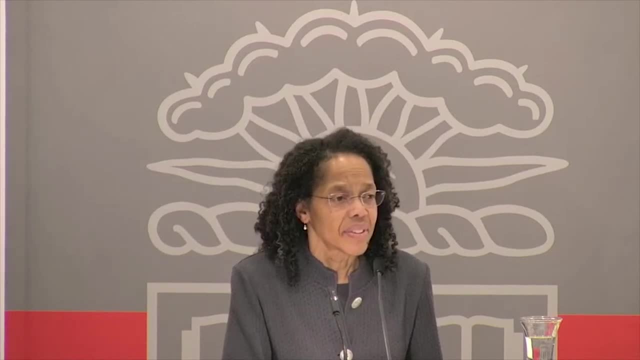 Do you know the rate of conversion to production? I mean so what's the ratio? and do you know the rate of change of that? or I can't put a time on it, but there is a particular delay time from the time that a cell 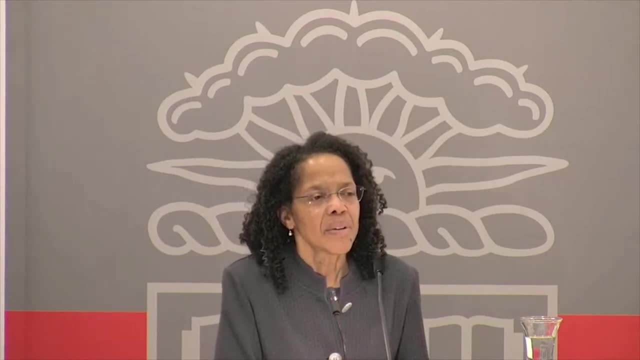 is in a deoxygenated environment to when it actually sickles. And so there are people who say, well, I don't know what's the rate of polymerization. And just one other question: If you know, if these in your experiments? 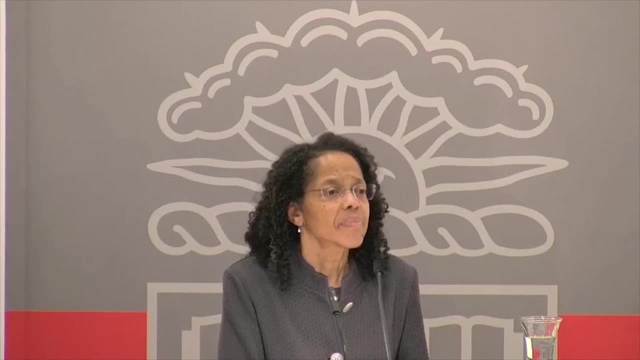 you can see how these in fact have very different physical properties than the healthy cells. Is there any way you can take advantage of that in terms of filtration process or anything that would actually remove them, Or is that just? it's just too pervasive. So the red blood cells normally have a lifespan of about 120 days, normally for a sickle patient. their cells are more fragile and the red blood cells are destroyed more rapidly and therefore it's also a hemolytic disease and that's why. 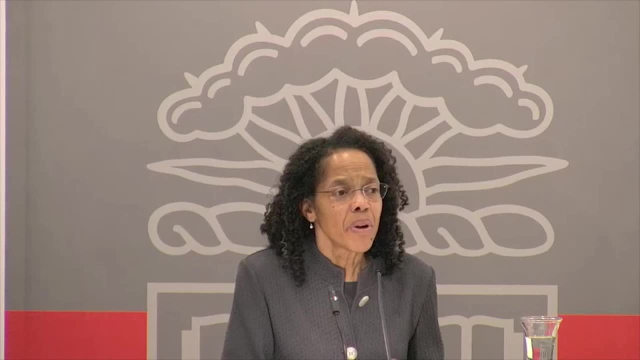 it's sickle cell anemia, And but this, one of the therapies that I did not really talk about is transfusion. So you can transfuse and there are many sickle patients that have had multiple transfusions. But, of course, the issue with a transfusion is it's temporary, because now you've transfused normal red cells with normal mechanical properties. but even those have a lifespan of 120 days. Absolutely, And interestingly enough, I didn't talk about this, but there was one strategy. 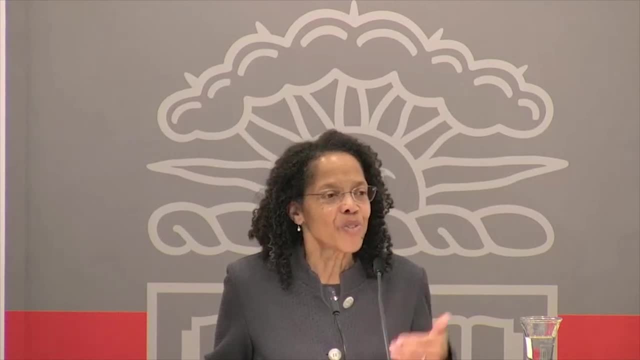 that was used where a drug. it was used in a clinical trial. there was a drug called- I believe it was called Floracor, but it was lubricant, And the idea was that can you take a lubricant and it lubricate your cells? 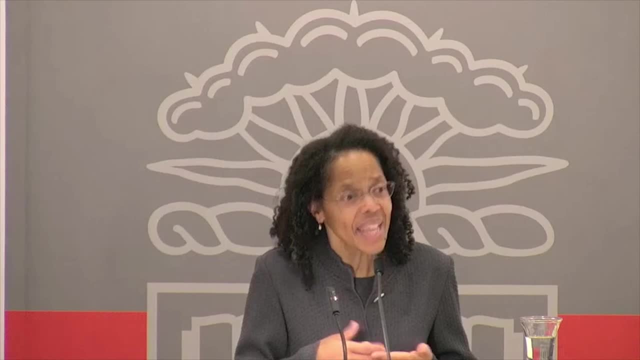 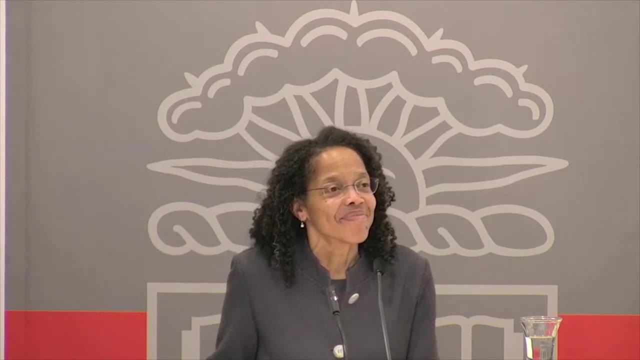 and therefore enhance it or improve the flow. Gilda, I'm very impressed with the depth of studies that you've done to look at adhesion and inflammation, the biomechanics, as well as the flow And, as you're probably well aware, 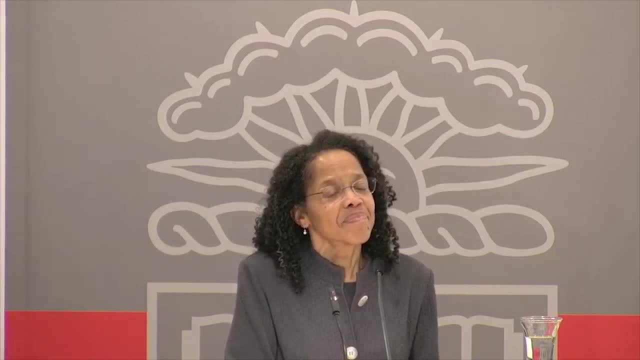 there's a lot of interest in repurposing of drugs. Yes, And through some of the systems that you've developed, it seems like you could look at sort of a a whole array of different types of drugs that you could use to improve the flow. 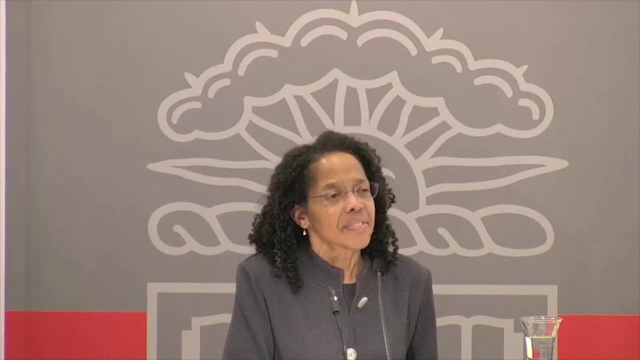 of the drug. Yes, A whole array of different, maybe anti-inflammatory drugs or other sorts of things that you could screen to see how they may affect the actual biomechanics, flow, adhesion and all of these, you know, different sort of points. 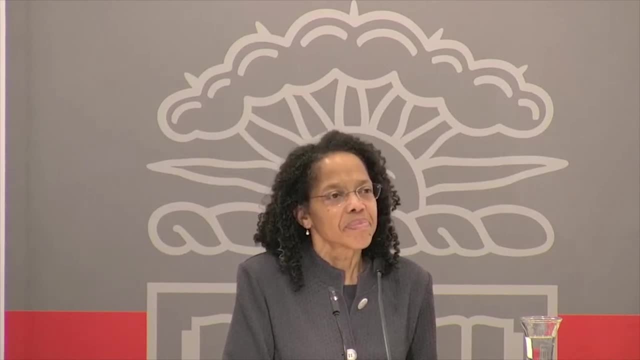 that affect the disease and the clinical outcomes. So do you have plans to do that? Is that something that has traction? Has you know, the clinical side of therapy moved towards testing other types of drugs? Yes, absolutely, it has. 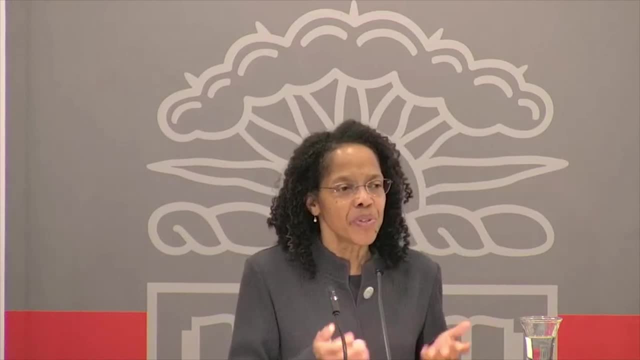 And so the beauty of- and this is again like an engineering approach- the beauty of being able to have an in vitro system. it allows you to do that level of testing. So so, so, here's what we do. 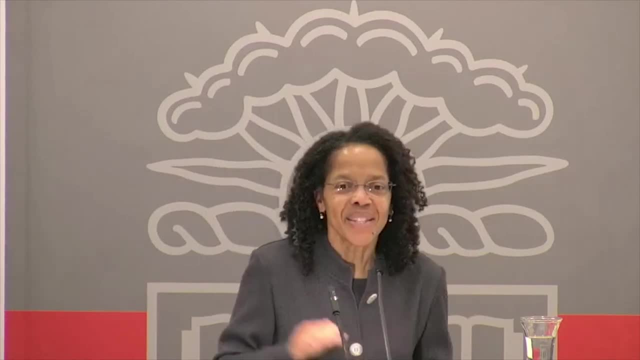 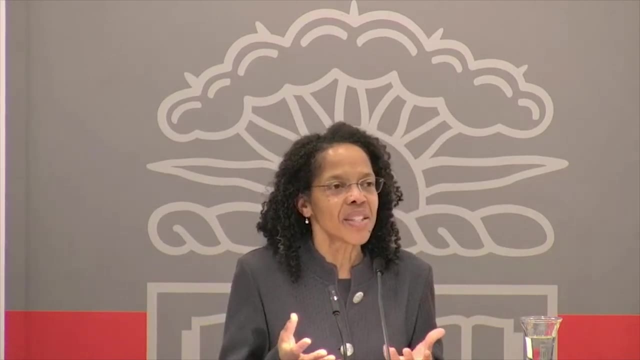 We typically do this as engineers. You, you break a system down and make it as simple as you can, and then you start trying to add back in, because you take these very complex systems and you're it's. it's a very complex system. 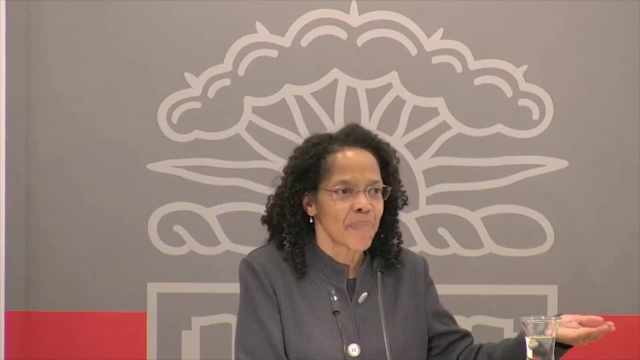 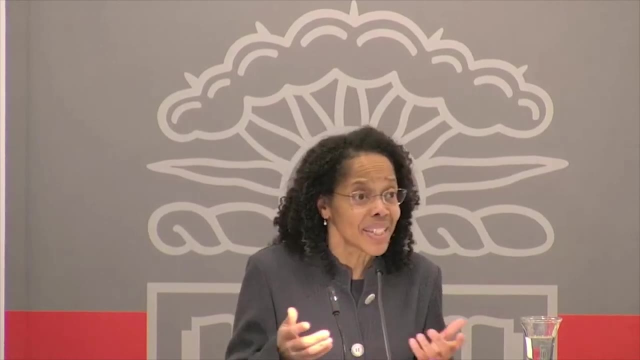 and you're trying to say: but what impact does this cell type have versus another blood cell type? Or you, you put an inflammatory mediator in and you're like: well, what cell type is it affecting? The beauty of our system is that we can. 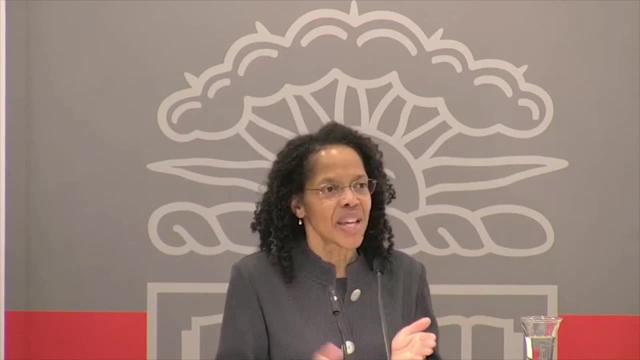 just take those different pieces out, Like now: we're just gonna take this cell type and put this inflammatory mediator in, with or without endothelial cells, maybe with or without protein. that's on the matrix and we can do that, and then we can add. 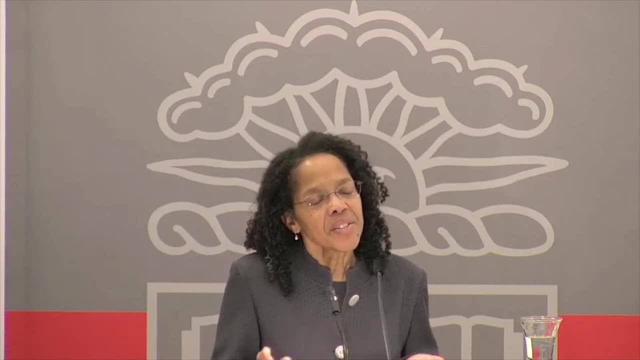 things back in and tell this complicated story. Another thing that's starting to happen- and many of you may know about this too- is, like I showed you, the original parallel plate flow chamber system we were using. That's considered. that's a big chamber. 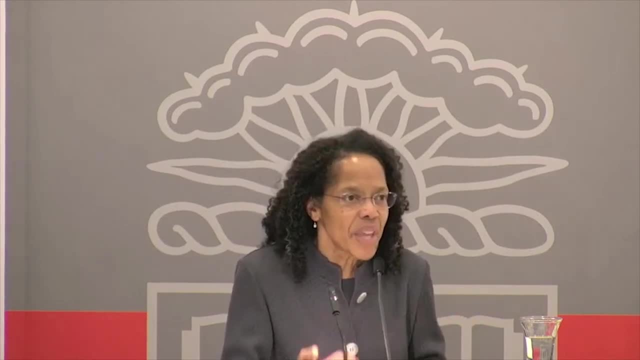 Everything is becoming more miniaturized, and so now we use microfluidics. but one of the reasons that it helps us to use microsystems one: it's recapitulating small vessels. but also you use fewer reagents and so you can do higher throughput. 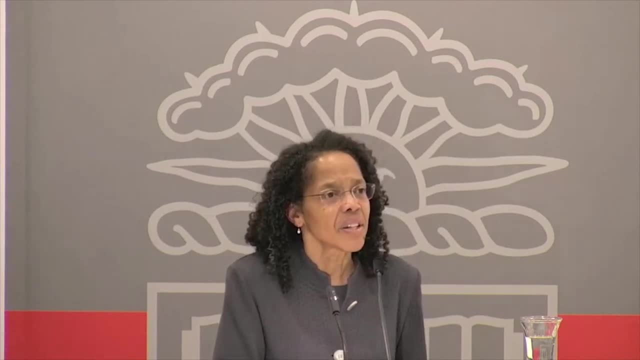 and that allows you to do the kind of testing that you're talking about: Try different drugs that may or may not work under different conditions. So the other thing that we've been trying to do over the years is the conditions. So what are the? 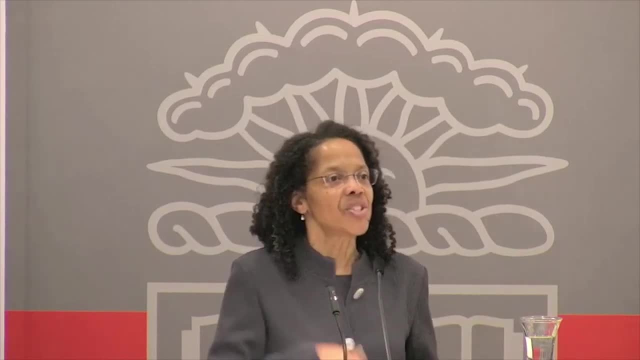 conditions under which you're more likely to see this type of adhesion which cell type? and so that your question is spot on, and that's the kind of thing that we're trying to do. Hey, Gilda, can I ask you one more question? 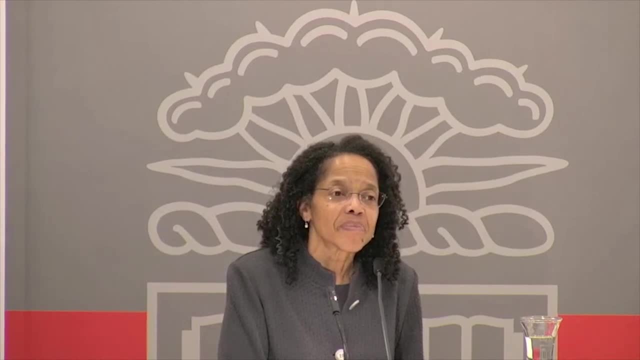 about the mechanics from the last part of your talk. And so when you see the less stiffening in terms of the mouse model, but it's just a sickle red blood cell. so is it that the red blood cell talking to the osteoblasts? 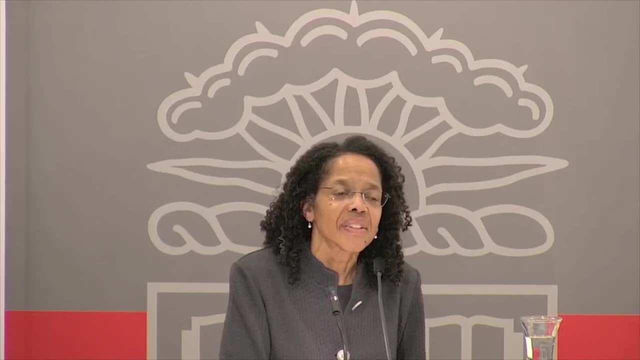 is not maturing into clasts, or is there like something with rantes, or do you know yet whether there's some molecular Right, So that we don't know? The first thing we were trying to do is like, okay, first of all we need to show. 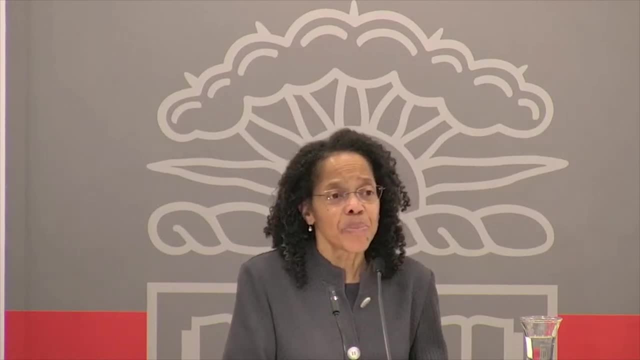 something about the broader properties in the phenotype. Now that we've done that, the next sets of experiments that we're trying to do is move it to the cellular level and to look at the different cell types: the osteocytes, the osteoblasts. 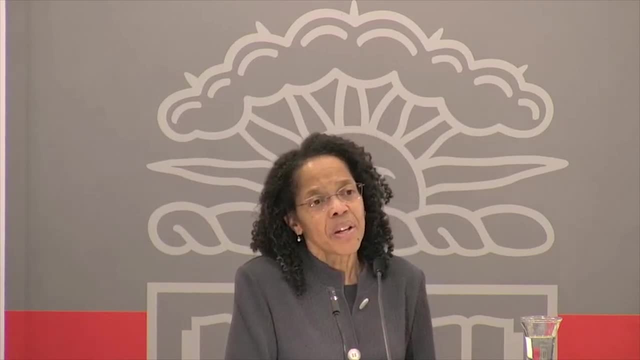 in the presence or absence of a mediator or not, and that's where we are right now- is to actually try to figure out what mechanism of cell death, what happens in presence of hypoxia or it's not a hypoxic region and eventually we're also. 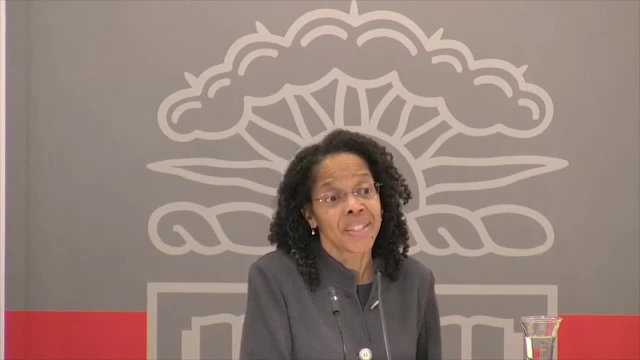 going to move into the bone marrow, which gets even more complicated. Hello, I just want to say thank you for your talk. My question, or rather request, is: do you have any advice for any us young budding scientists who might find that it's difficult to advance? 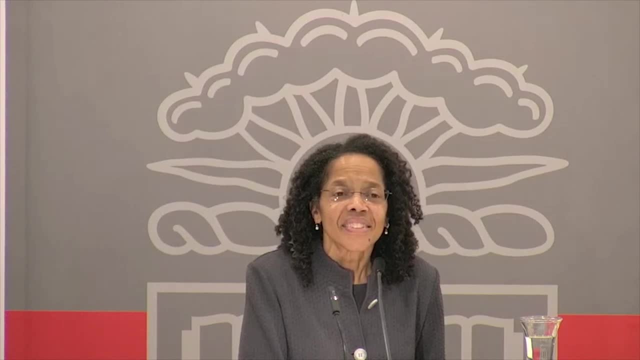 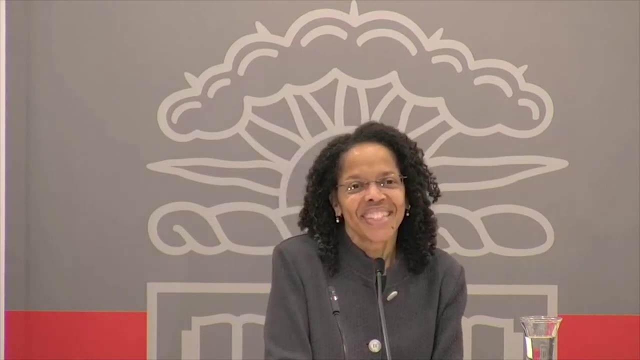 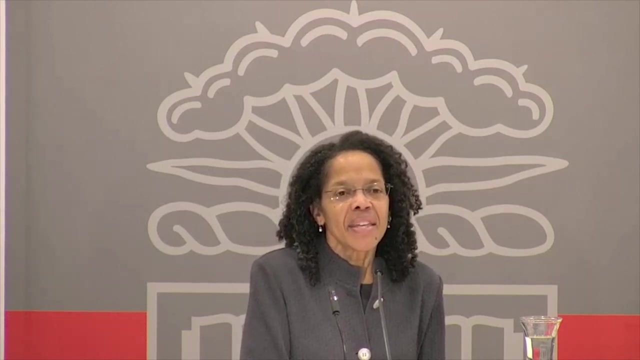 in a career in science due to the political climate or policies surrounding, or just in general advice. Sure Well, speaking from my own experience, I think that part of what we need to do is find good, relevant resources that we're interested in devoting our research. 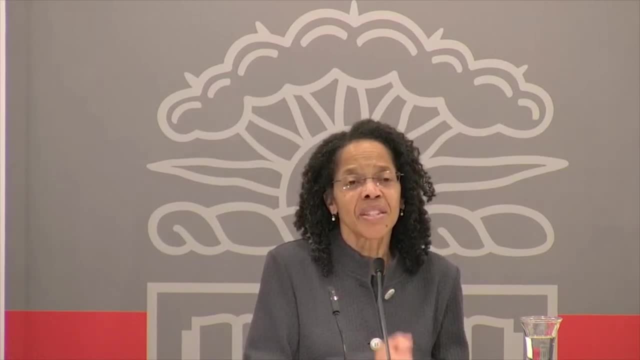 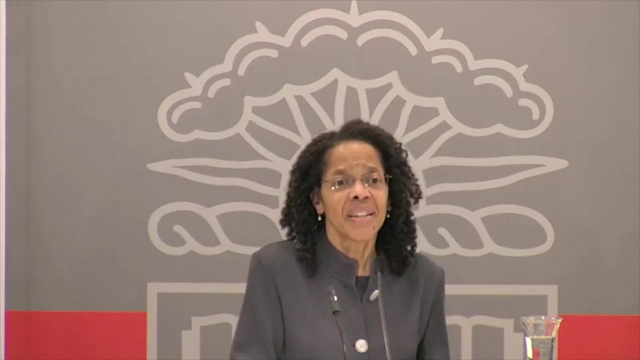 careers to. That's one piece of it. Doing the best work that we can do. Excellence- No one can argue with excellence, and so that's one piece of it. I think, connecting to those who can be our advocates- it could be the right. 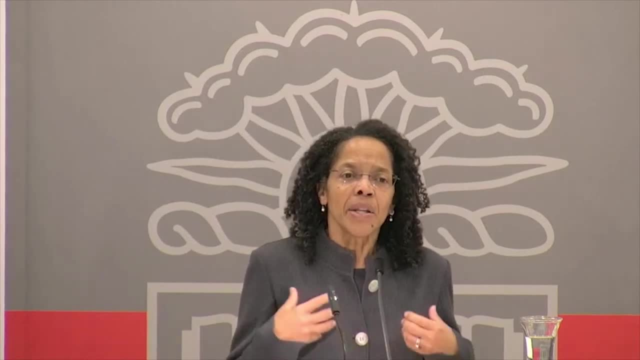 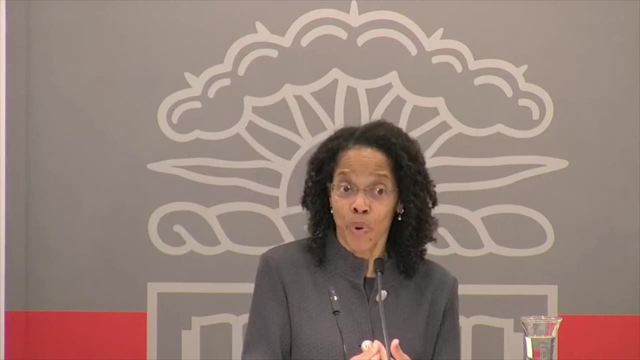 advisor. it could be an advisor, but to the extent that we can joining environments that we know, at least have some evidence of being supportive of people from different backgrounds, I absolutely do think that makes a huge difference, especially even if it's at the undergraduate or graduate. 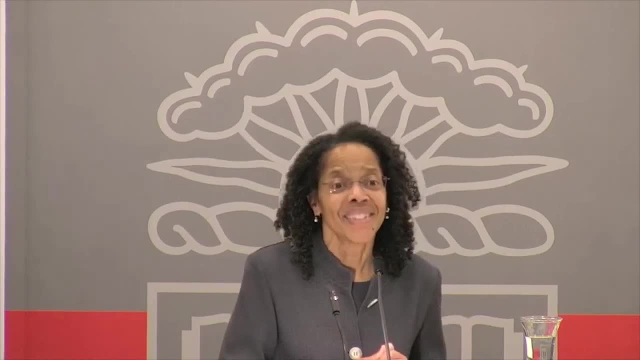 level. If you're going to take your time to join a group of people, you have to be smart. Sometimes I get asked what's more important: the project or the advisor. The advisor: You can change your project. You can't change that advisor. who? 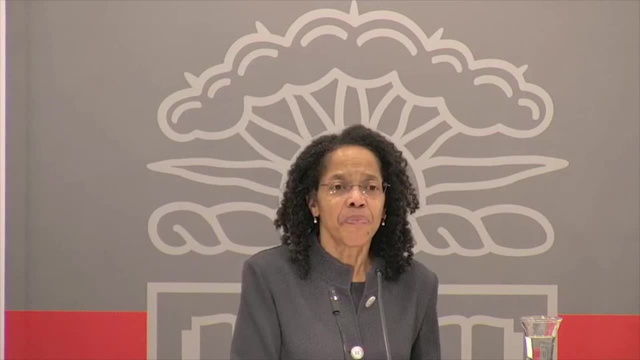 that person is And often times it's about fit. There needs to be a sense of community and often times I think it's the importance of support. We're not islands. Science is social, Engineering is social. We operate on problems collectively. 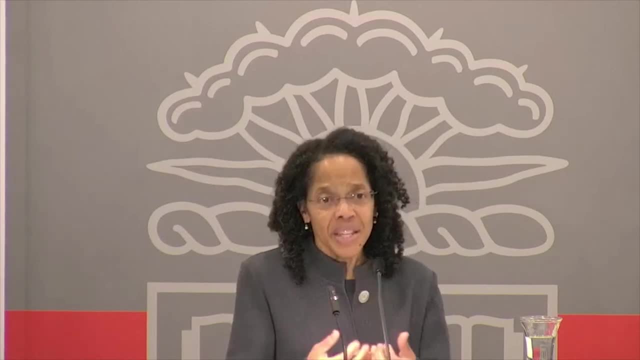 And so I tell those who are interested in joining the field, like, let's be part of that team, but let's not think that we have to do it by ourselves, and look for the support where we can, Since sickle cells, as I understand it, tend 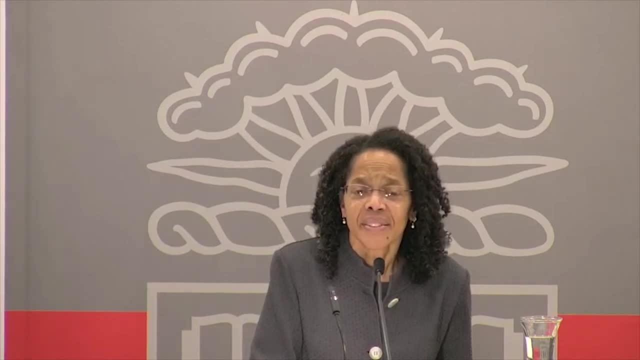 to adhere to the blood vessel walls. can you do something like dialysis so that the sickle cells would adhere to the walls in the dialysis machine and the red blood cells would come out? So I don't know that people thought of it from the dialysis. 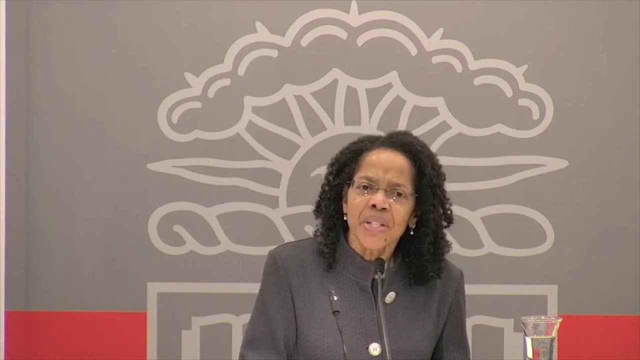 like transfusions. For some reason sickle cell patients can have every complication there is and they don't tend to be on dialysis as often as you would think for the kinds of complications that they have. But to your point about the concept, the concept. 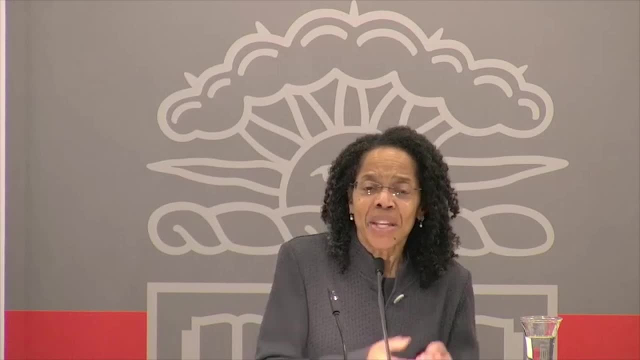 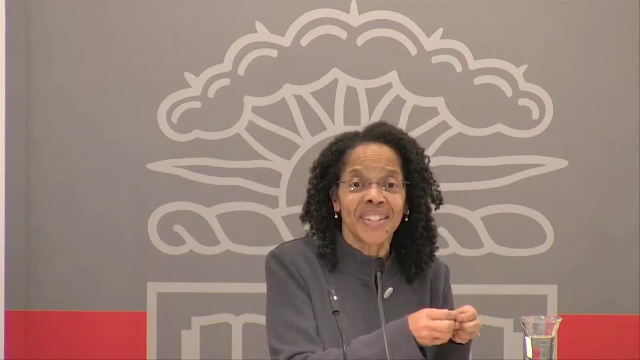 of like dialysis, like removing the blood cells from the cell walls. it's not a good idea, but I think that's a good way to take the bad actors out. Isn't that what you were just showing? that they take themselves out on the dialysis. machine and they take that. so the sickle cells would adhere to the tubing that they were flowing through and the normal cells would not get stuck. So you mean, like in an extracorporeal way? Yeah, Analogous to a dialysis machine. 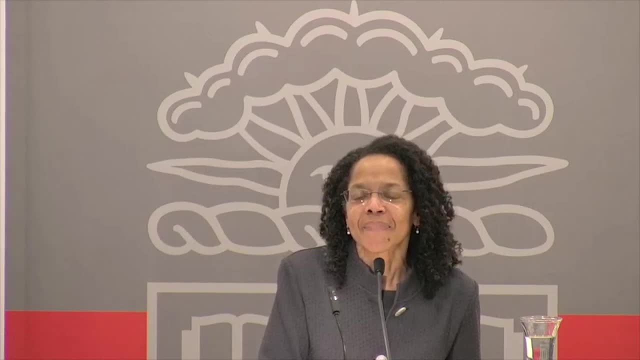 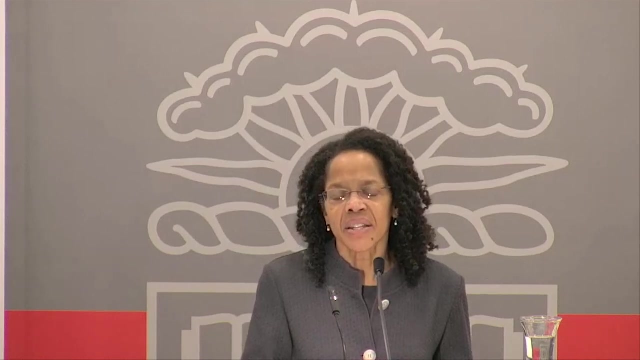 Sure, What percentage of. I had a cousin who died of sickle cells. so what is the percentage of sickle cells resident in a body? So if you have 10 quarts of blood, or how many quarts of blood, how much of that? has sickle cells in it, Which is an average density. So you separate cells out by density and they'll. you can get percentages of each cell type. So and then you can add those together and figure out. So for a sickle patient they might have like 20% of their cells that are irreversibly sickle, for example, And then another percent that is sickle and the reason why the percentage of reticulocyte cells, those young red blood cells, are so high in sickle- 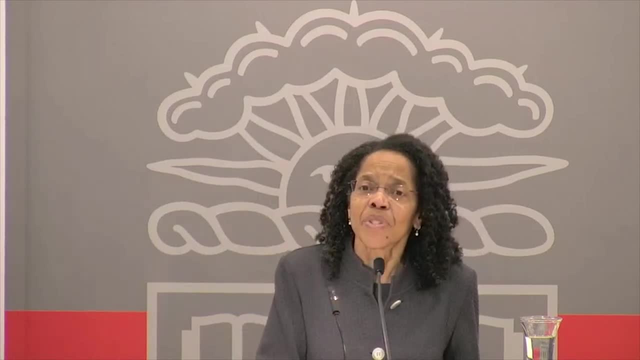 patients is because there's a hemolytic anemia and the cells are constantly being destroyed, so the body's constantly producing new cells. So at any given for any given of them have sickle hemoglobin, but the ones that are actually sickled or higher density might be 50 to 80%. Yes, If it's 70%, you know, then you gotta transfuse, Right. Hi, thank you for your talk. I was wondering what's the first symptom of sickle cell anemia. so 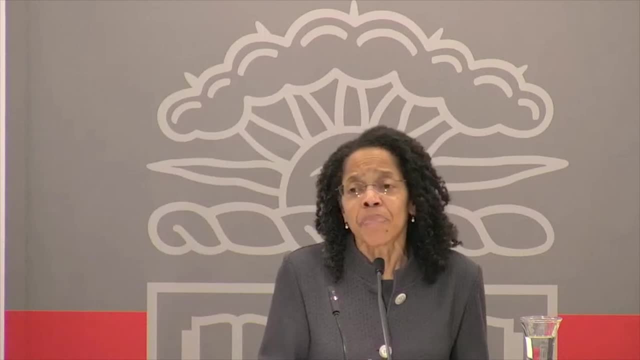 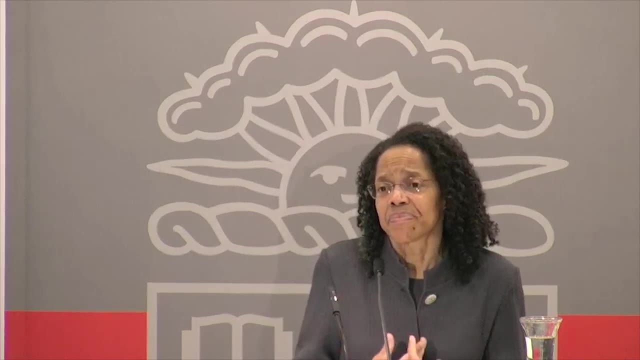 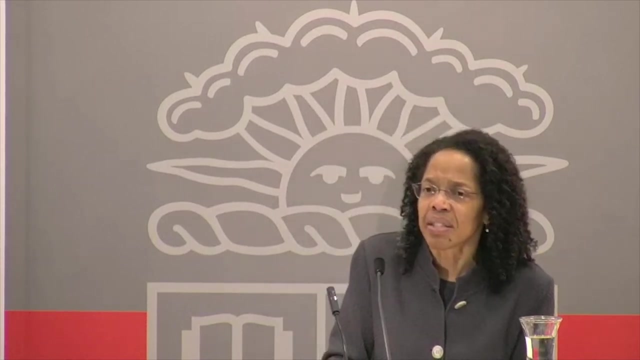 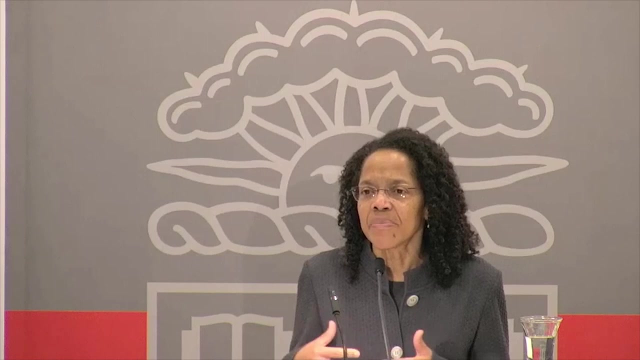 in kids. so the the big symptom actually is pain. So these vaso-occlusive crises, you're not getting any oxygen to these tissues and particularly in joint areas. so the big symptom is pain and pain in joints and often times in children and the fetal. 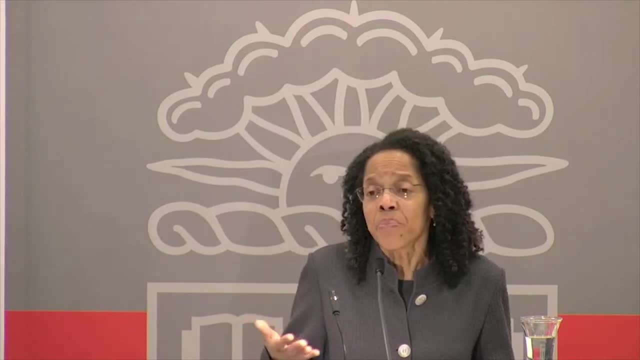 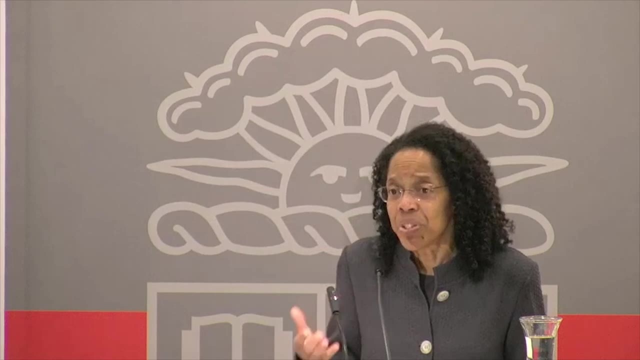 hemoglobin and the fetal hemoglobin will last for a certain time and then it turns over. so someone might have fetal hemoglobin that hasn't turned over to the adult hemoglobin for a couple months and in fact in Africa in particular there were many kids that had 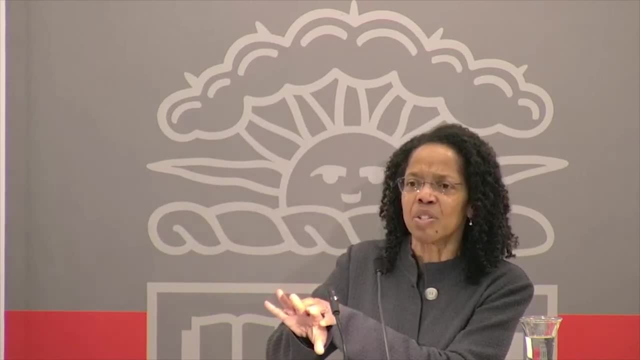 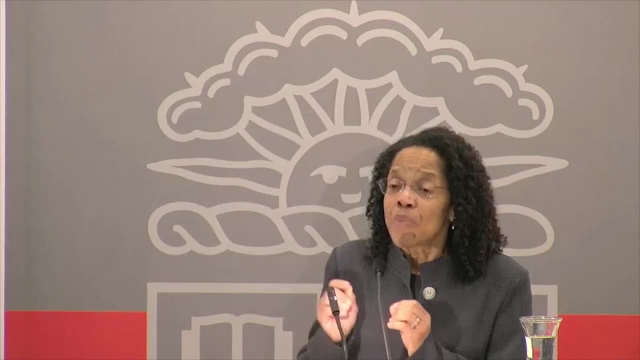 fetal hemoglobin, and they had a lot of swelling. so those are some of the signs that you see, and the clinical manifestations can be very early on. There's a lot of variability in the disease, though, so what you might see in one patient for a few months- 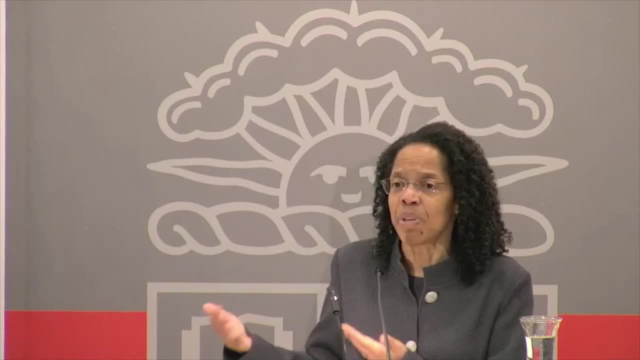 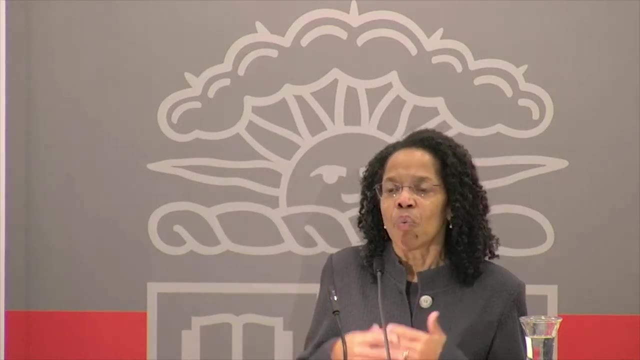 in a row with debilitating crises and then the next month be much better off. and we don't have a predictor, and so some of the work that we're trying to do is to continue to look at what might be a predictor, and so the reason why we're 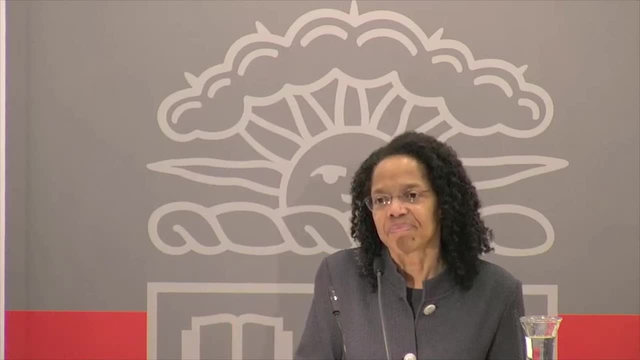 looking at biomechanics is like a very complex process, and so we're looking at the structure of the flow over these particles, the sickle cells. the drugs that are given, are they actually affecting the cell itself or the flow of the blood? because the question is: 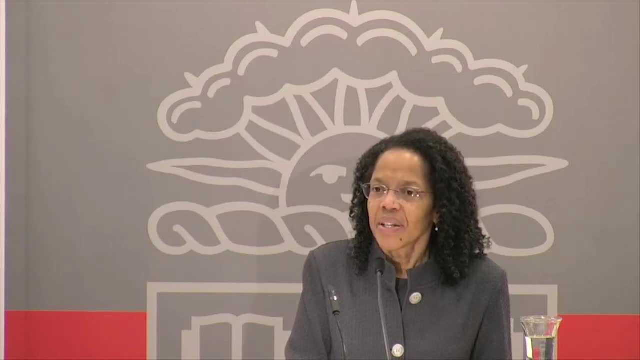 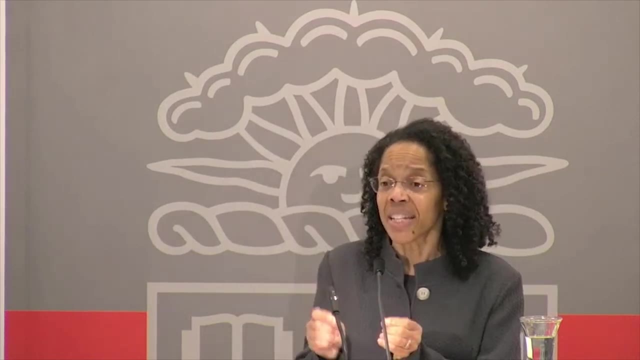 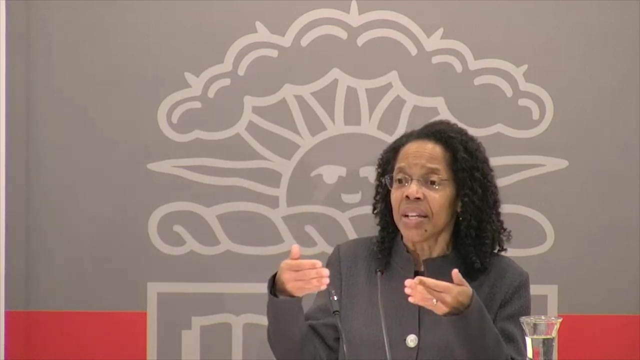 how the other normal cells can flow through, right, what exactly is happening with the drug? so there's different drugs and the different drugs target different things. so you might have a drug that's targeting sickling, so it's an anti-sickling drug, and so that 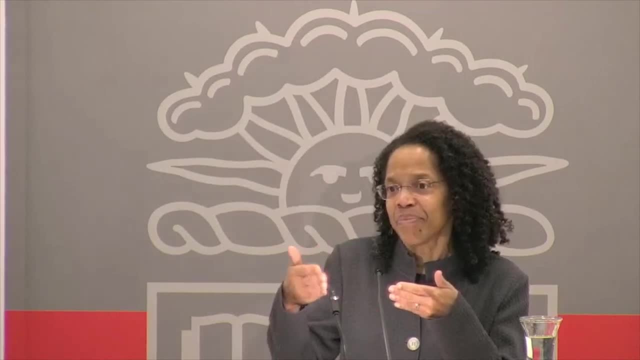 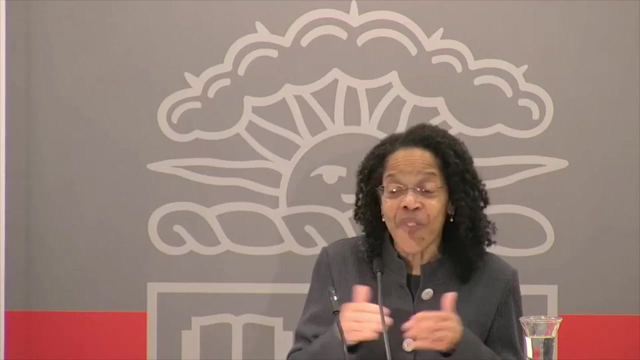 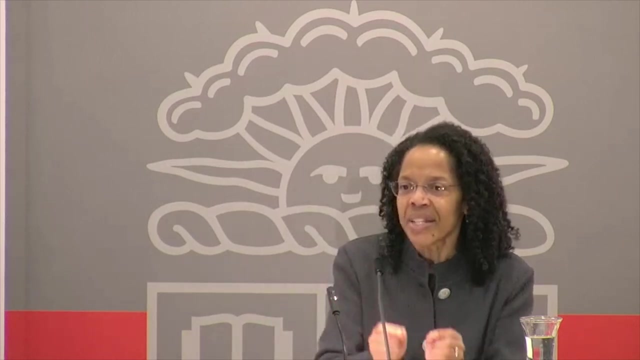 drug would be keeping the antagonist. so now you don't get the adhesion- the one that I mentioned- that they said it was a lubricant. in that case they were like, okay, this is going to make things more slippery, so it depends on what you're targeting. 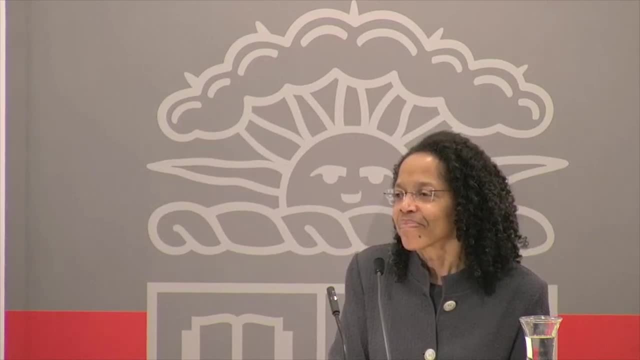 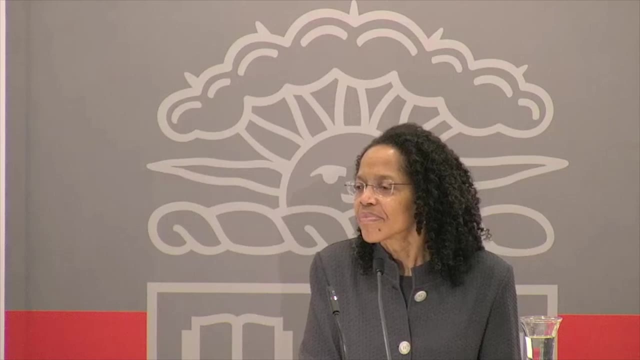 thank you for the talk. this question is not so much likely to come from your research, but so most of the research that I've heard to describe, I would say, would be prophylactic in nature, that you're trying to actually eliminate the underlying cause of oxygenation. 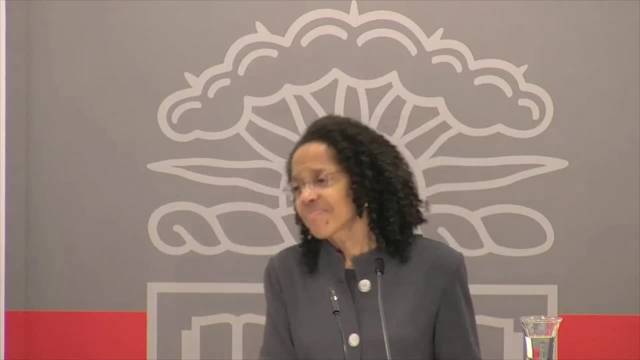 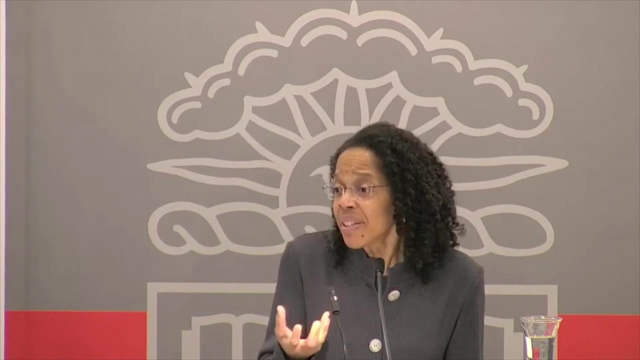 the hypoxia that is, you might imagine that, using some nanotechnology, that you could actually get more oxygen into the sickle cell, the ones that are reversible, and thereby lower the percentage. do you know of any research like that going on? I don't, but that's. 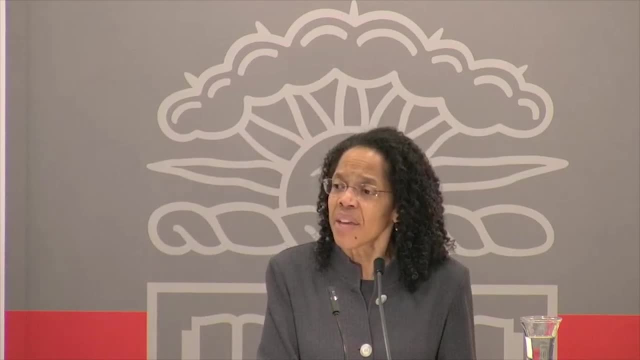 a great idea. how do you manipulate that? and I think that's definitely a reasonable strategy because it is all about the oxygen, so organizers prerogative. you also spoke about asymptomatic- yes, so carrying the trait, and I was really curious about the bone studies. it means 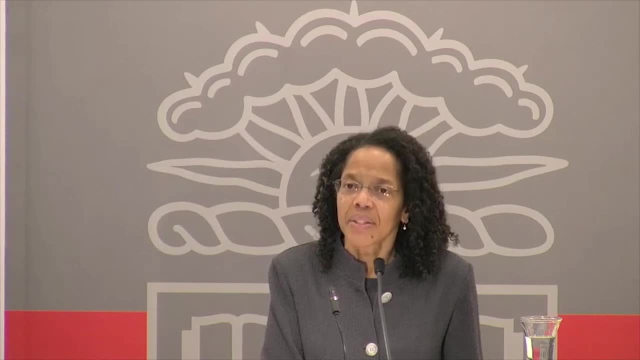 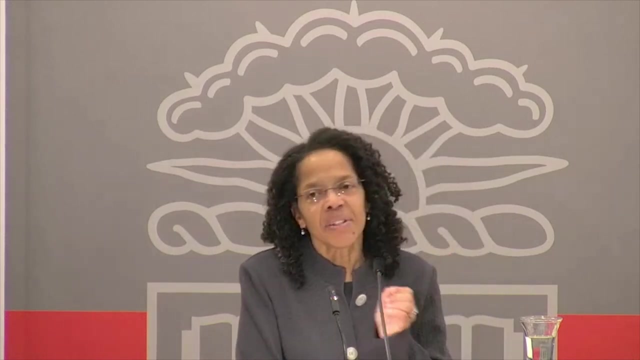 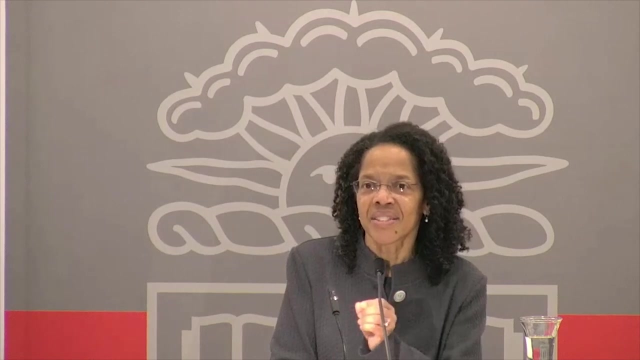 there are no sickle cells or fewer. I'm asking because I really don't know. so if they're carriers, that means that they have in each of their cells some sickle and some normal hemoglobin. what happens is, if you have any amount of hemoglobin, other than so. so, for example, hydroxyurea. one of the ways hydroxyurea works is because it up regulates fetal hemoglobin. so now, even though it's an adult, setting the percentage of fetal hemoglobin in the presence of the fetal hemoglobin along. 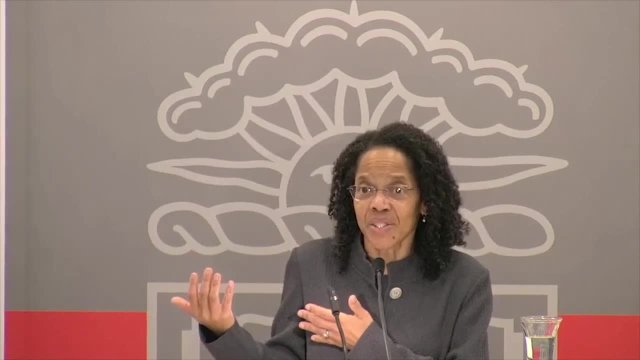 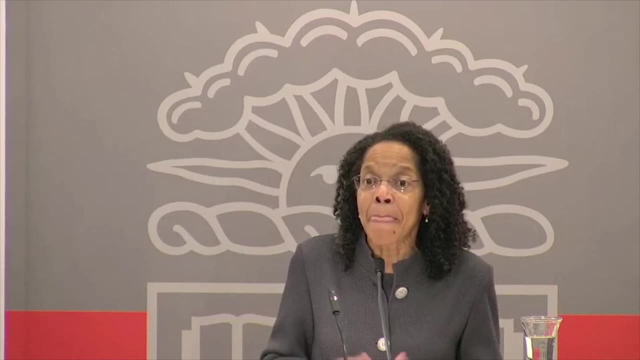 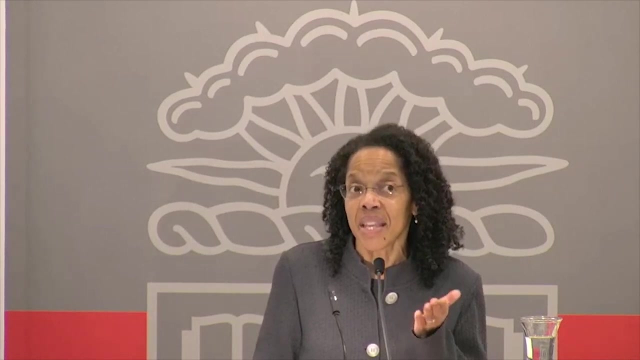 with the hemoglobin is not at a level to have these manifestations, so then they pretty much don't look at. we don't have to do anything for the people who carry us because they're going to be asymptomatic. but then they have what looks like a. 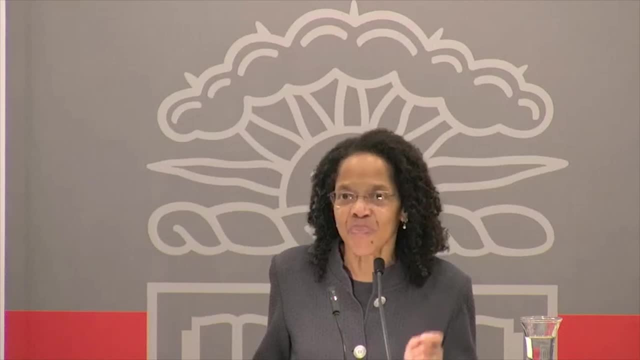 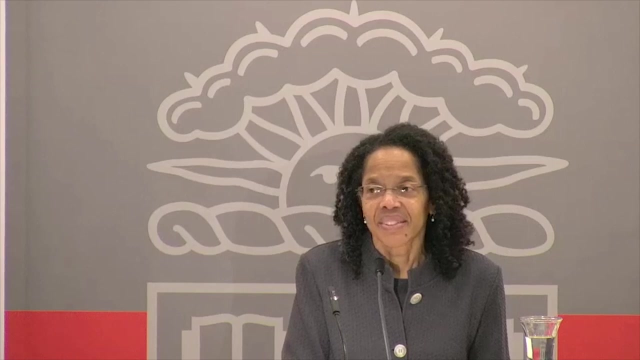 crisis, and so now for this work that we saw with the phone, we're thinking, wow, maybe there's something that we should be looking at for carriers and other tissues as well. so there's a there's a lot to think about. so thank you all very much. thank you all very much.